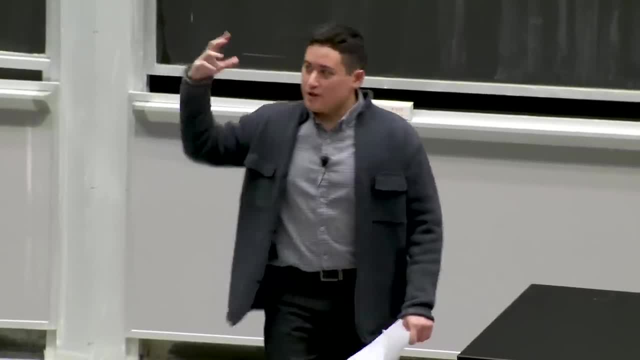 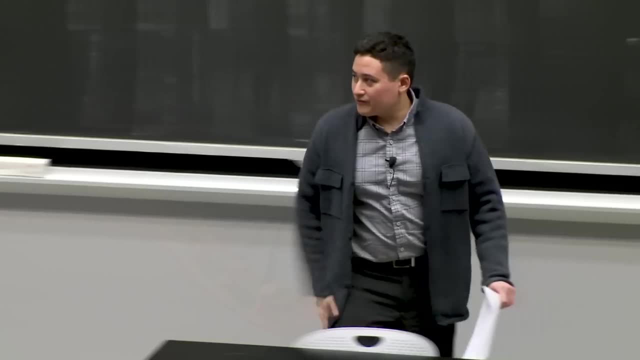 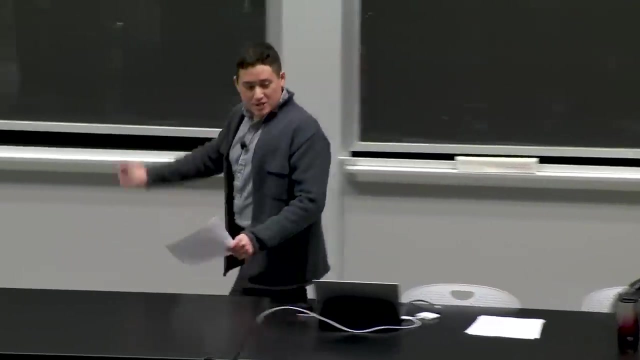 class with me. I will be teaching the first lecture and we'll have each of them teach one of the next two lectures and then we'll go from there. Yeah, so that's. this is intro to algorithms. OK, so we're going to start talking about this course content now. What? 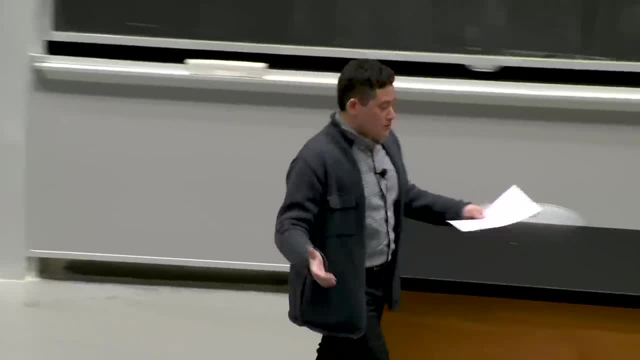 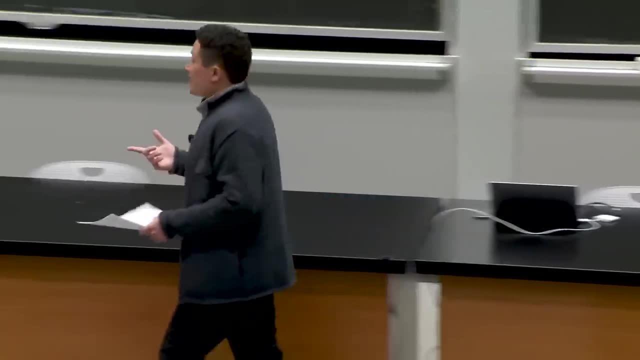 is this course about? It's about algorithms. right Introduction to algorithms. Really, what the course is about is teaching you to solve computational problems. But it's more than that. It's not just about teaching you to solve computational problems, So solve. 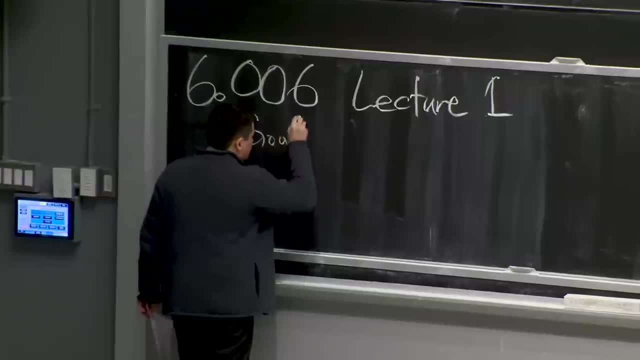 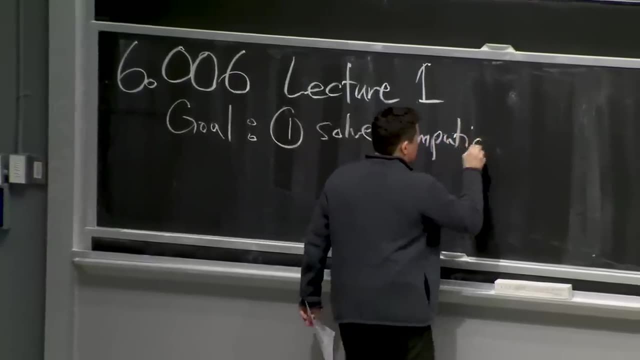 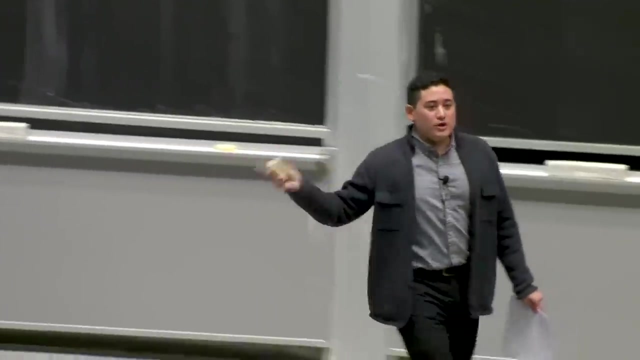 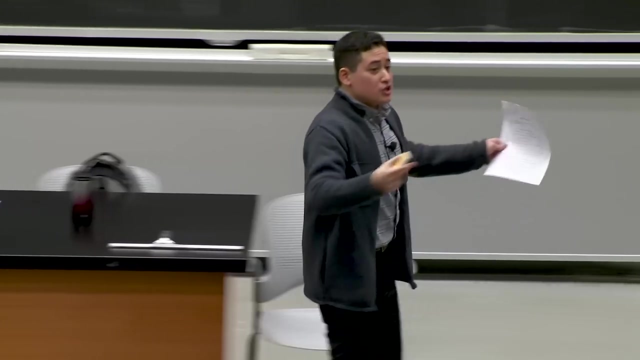 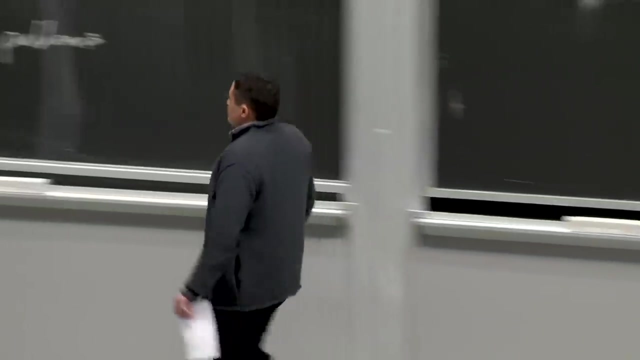 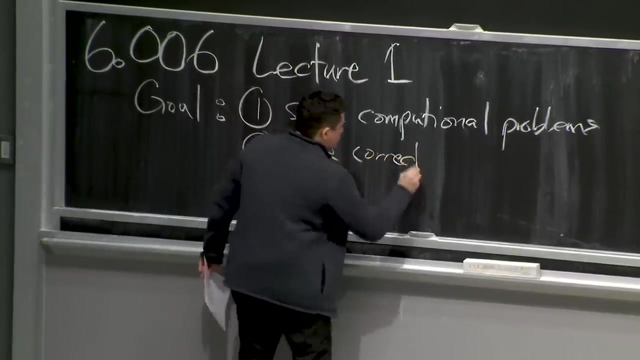 goal 1. Solve computational problems, But it's more than that. It's also about communicating those solutions to others and being able to communicate that your way of solving the problem is correct and efficient. So it's about two more things: Prove correctness, Argue efficiency. And then it's also about making sure you have the correct. 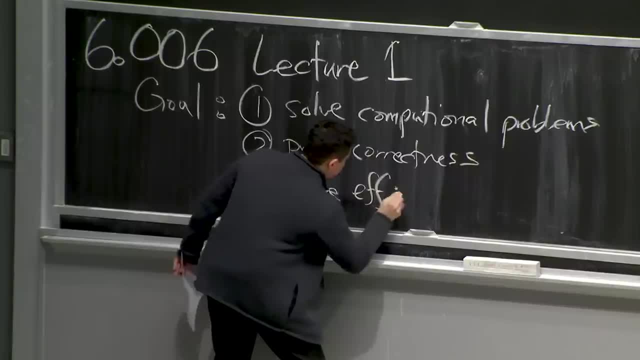 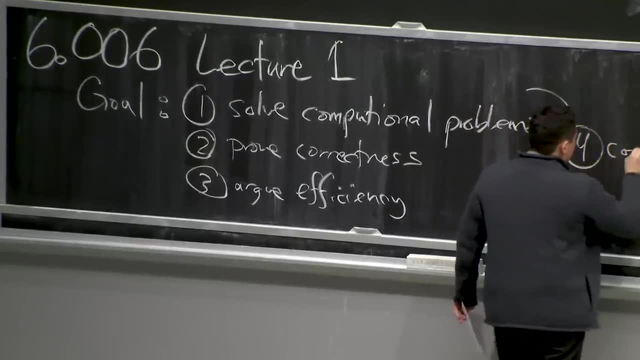 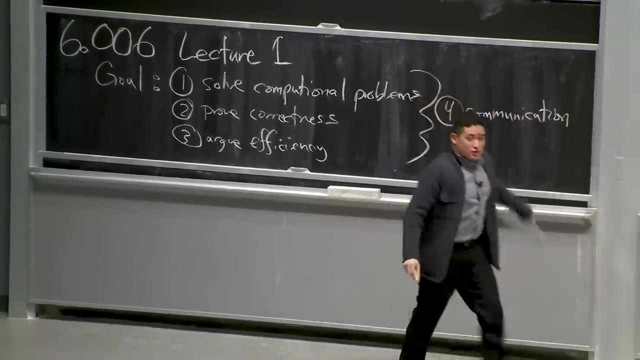 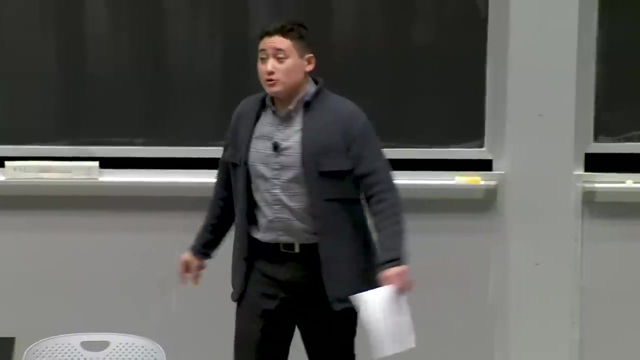 argue, efficiency, And in general, it's about communication. Communication- I can't spell, by the way, Communication of these ideas, And you'll find that over the course of this class you'll be doing a lot more writing than you do in a lot of your other courses. It really should. 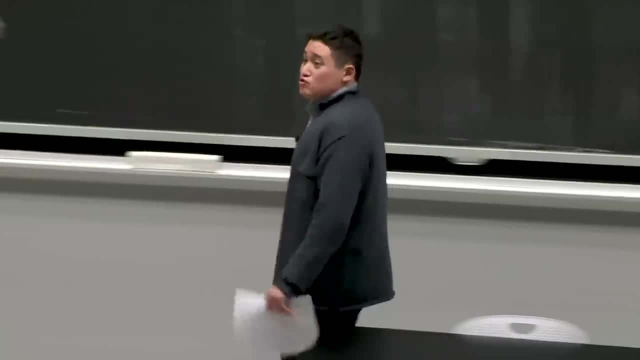 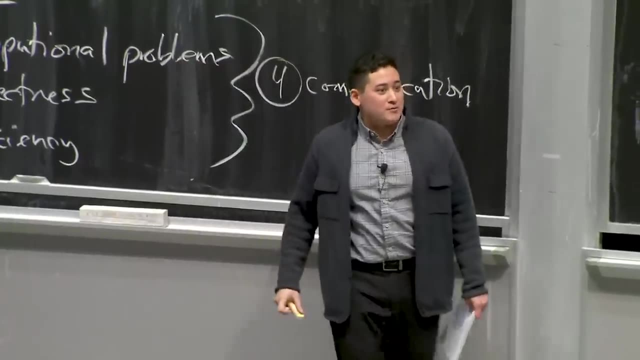 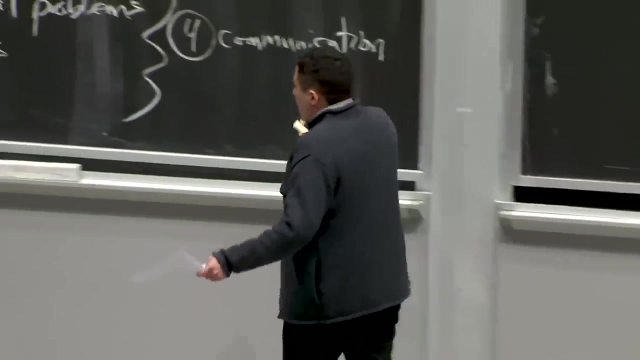 maybe be a CI kind of class, because you'll be doing a lot more writing than you will be coding, for sure. Of course, solving the computational problem is important, but really the thing that you're getting out of this class and other theory classes that you're not getting in other classes, 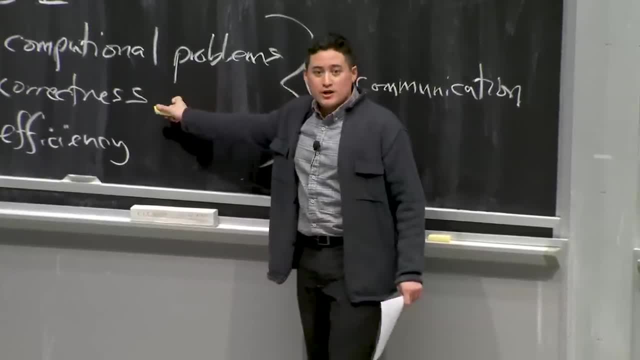 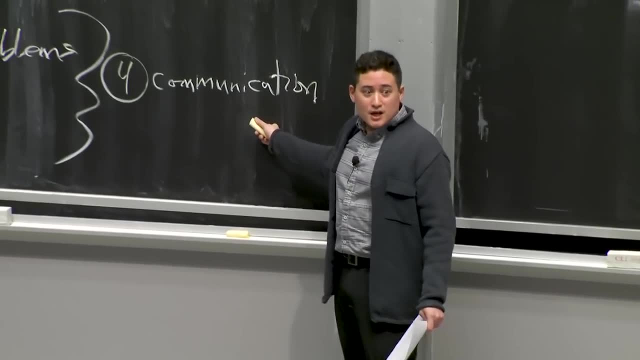 in this department is that we really concentrate on being able to prove that the things you're doing are correct and better than other things, and being able to communicate those ideas to others, And not just to a computer- To other people, convince them that it's correct. 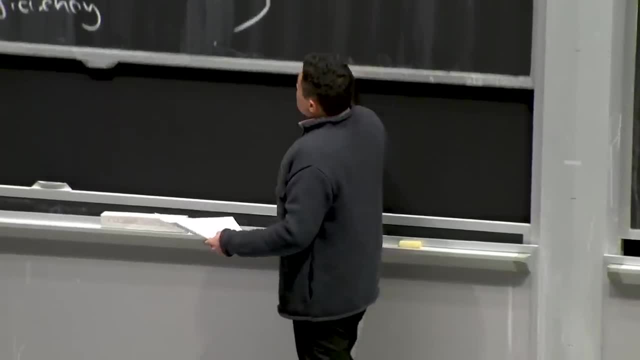 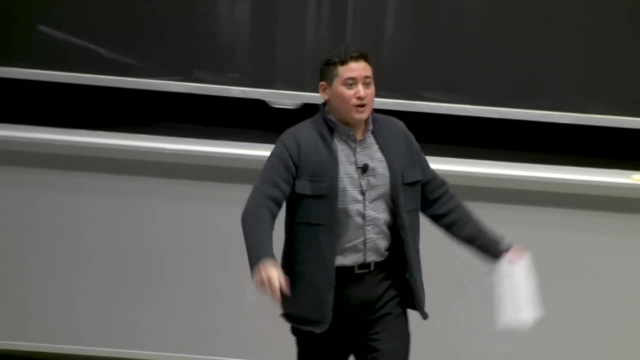 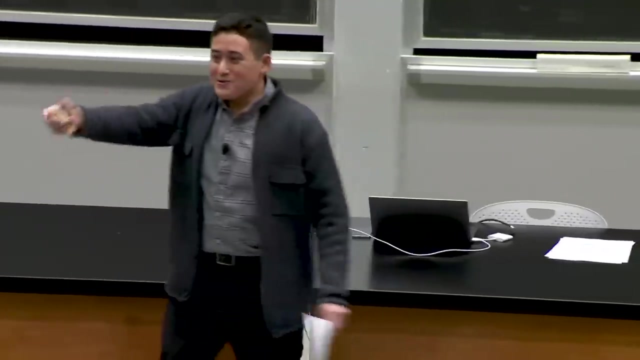 So that's what this class is about. So what do I mean when I say solve a computational problem? What is a problem? What is an algorithm? I know people make fun of me because I start with this question, but I mean, anyone want to answer that question? No, What's a problem? 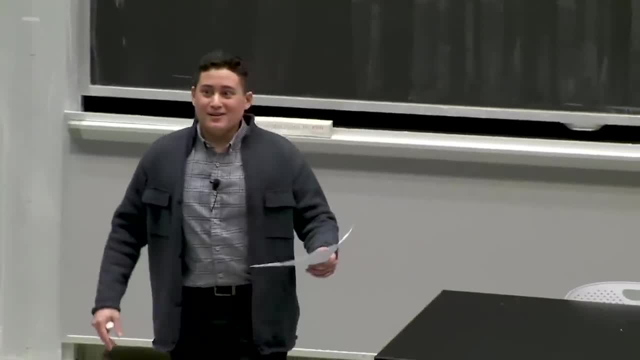 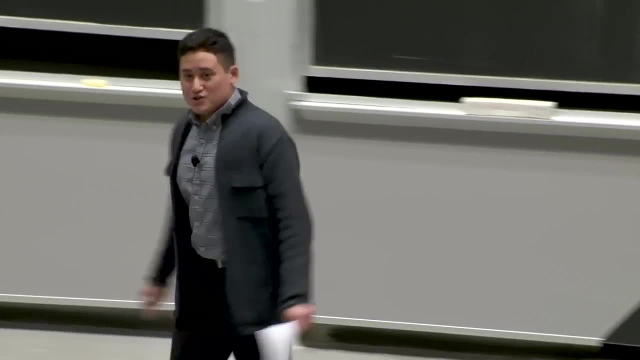 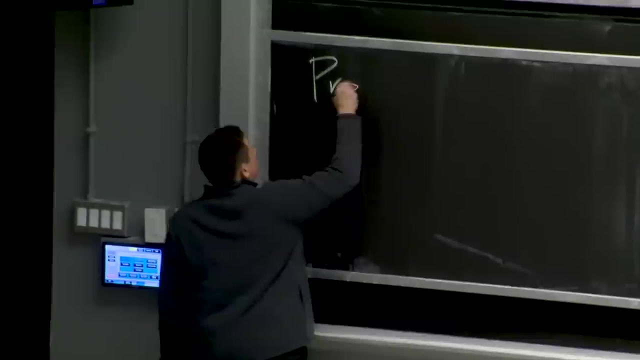 Computational? No, OK, so it's not such a stupid question. Yeah, Something you want to compute? OK, yes, that's true, But kind of a little bit more abstractly, what I'm going to think of a computational problem being- and this is where kind of 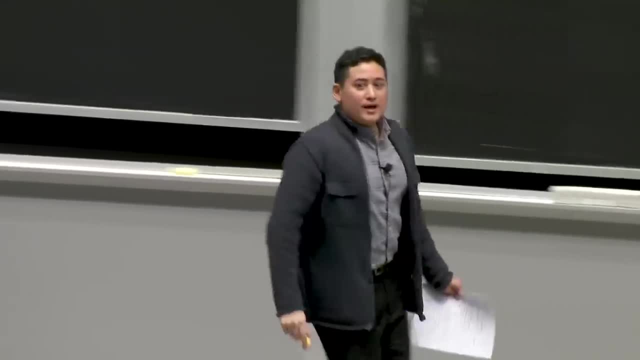 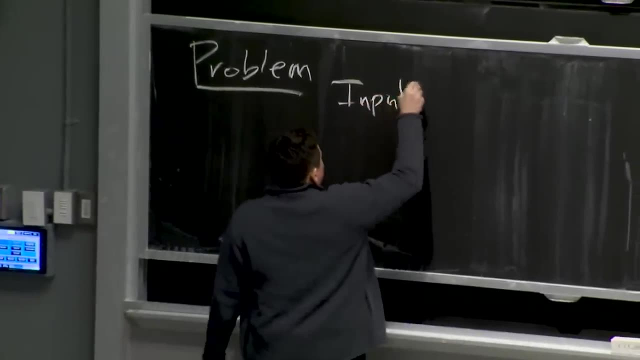 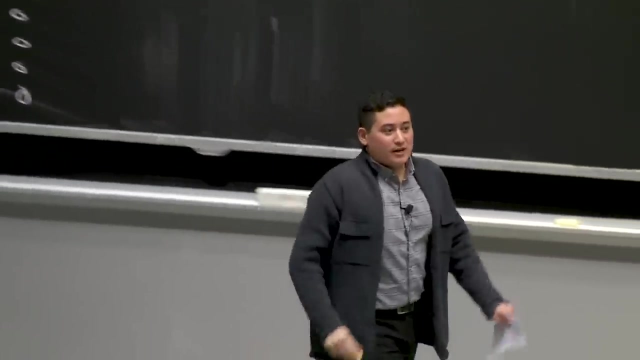 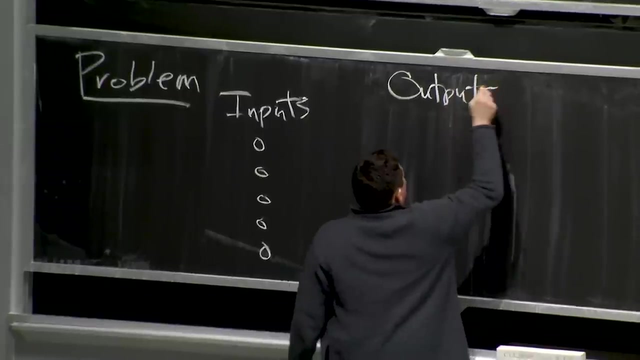 your prerequisite and discrete mathematics should come in. it's a problem is kind of: you've got a set of inputs, Inputs- OK, maybe I have one, two, three, four, five possible inputs I could have to my algorithm. Then I have a space of outputs, Outputs, And maybe, I don't know, maybe I have more of them. 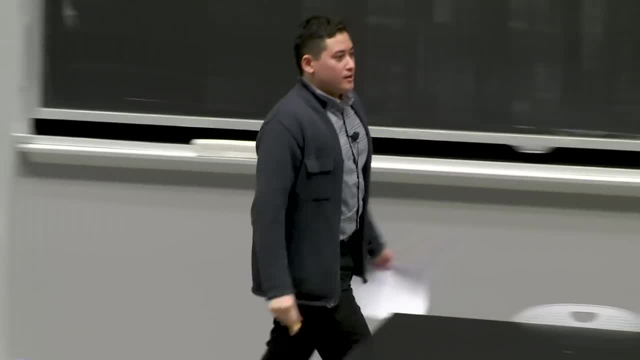 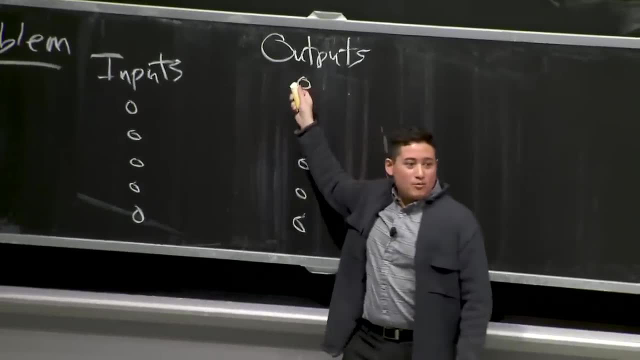 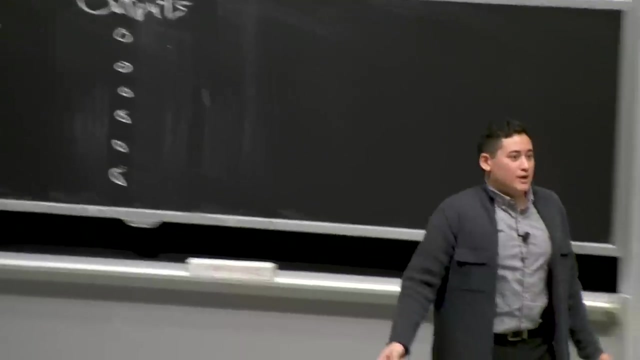 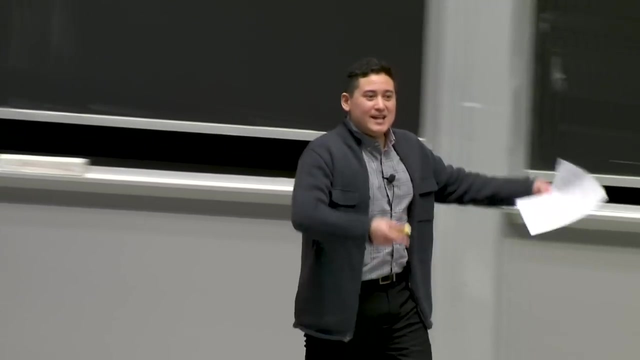 than I do inputs. but these are the possible outputs to my problem, And what a problem is is a binary relation between these inputs and outputs. So essentially, for each input I specify which of these outputs is correct. It doesn't necessarily have to be one If I say: give me the index in an array containing the value. 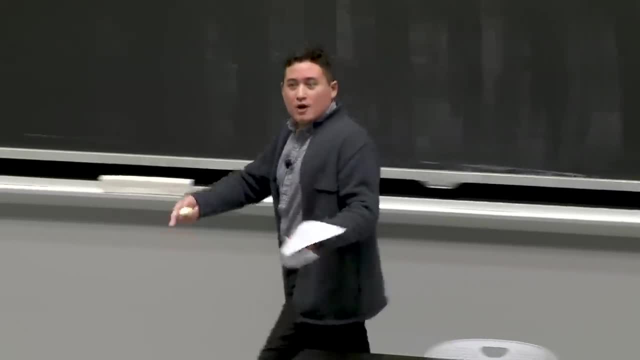 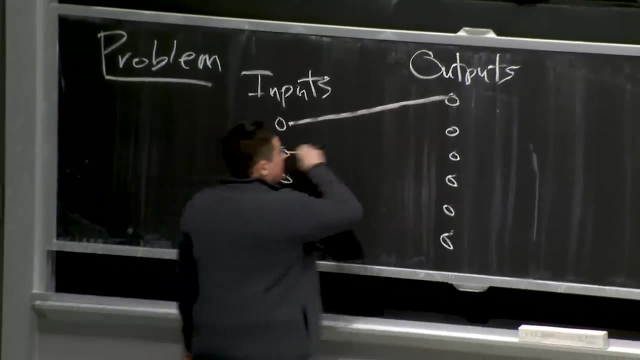 five. there could be multiple fives in that array, And so any of those indices would be correct. So maybe this guy maps to that output and maybe this guy maps to I don't know two or three outputs Right. This input. 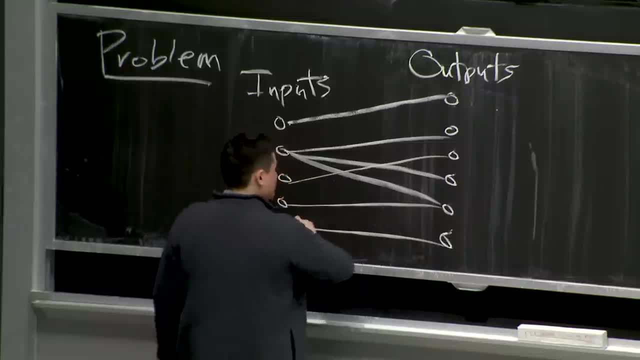 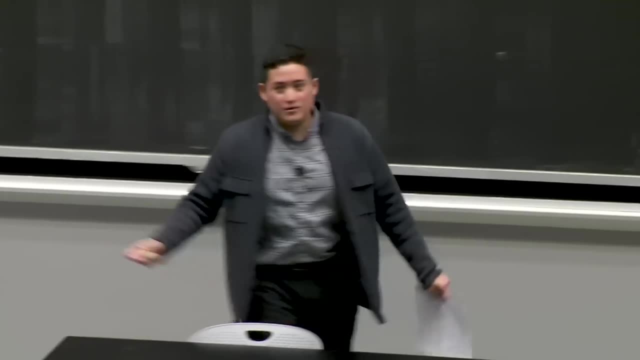 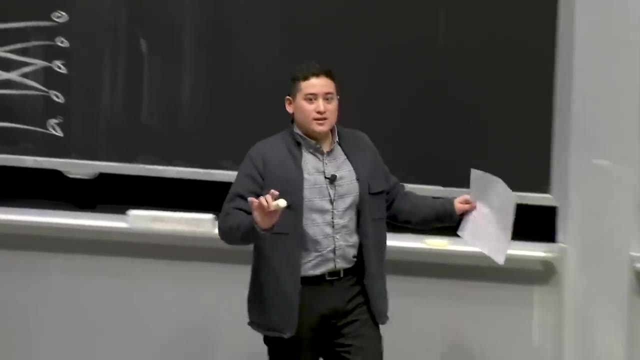 goes to one, two, I don't know. There's some kind of mapping here. These edges represent a binary relation And it's kind of a graph of bipartite graph, between these inputs and outputs And these are specifying which of these outputs are correct for these inputs. all right, That's. 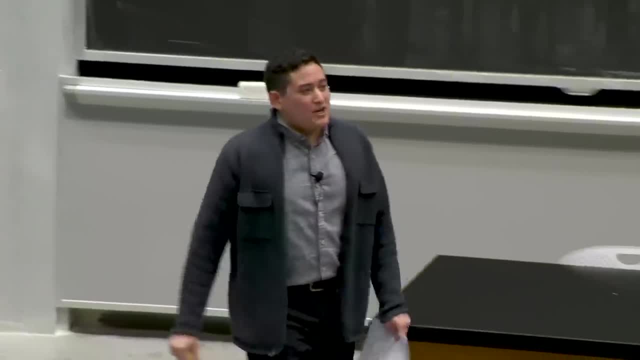 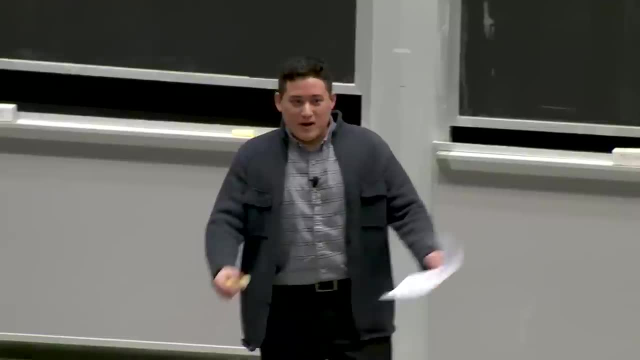 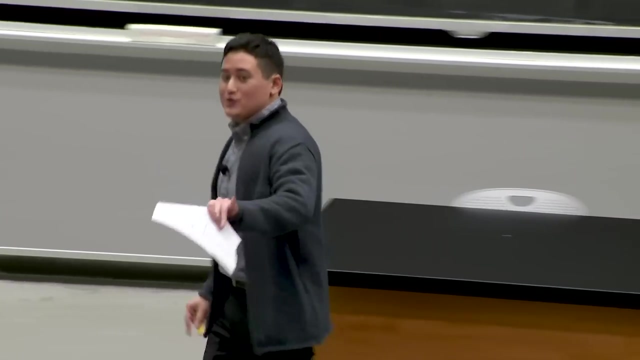 really the formal definition of what a problem is. Now, generally, if I have a problem, a computational problem, I'm not going to specify the problem to you by saying: okay, for input one the correct answer is zero, And for input two the correct answer is three, and so on and so forth. 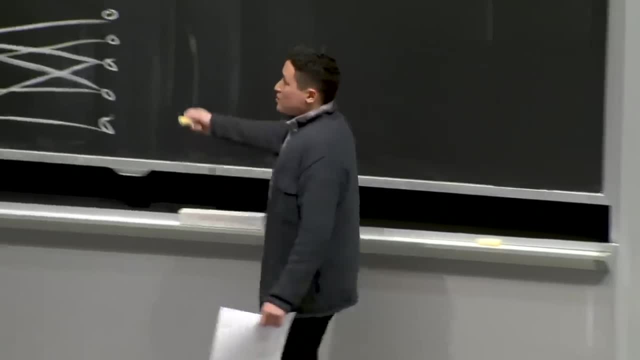 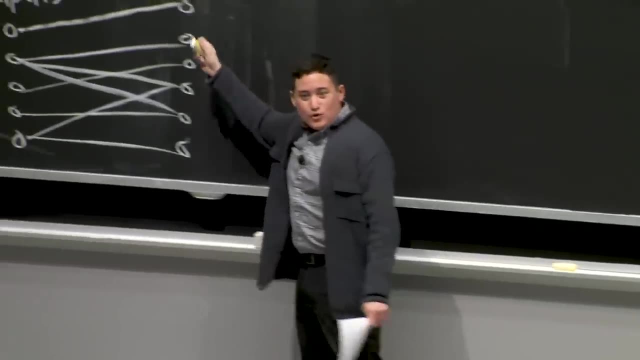 That would take forever, right? Usually what we do when defining a problem is specify some kind of predicate, saying that, oh, we can check. If I give you an input and an output, I can check whether that output is correct or not. 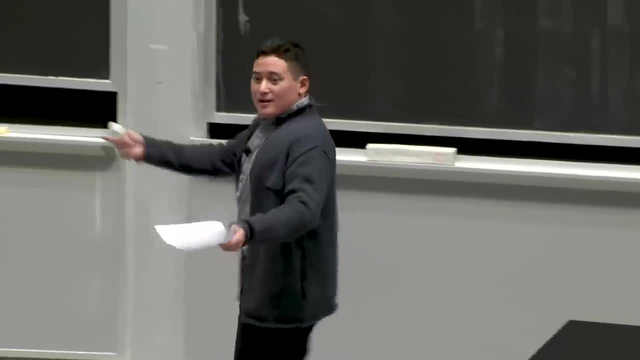 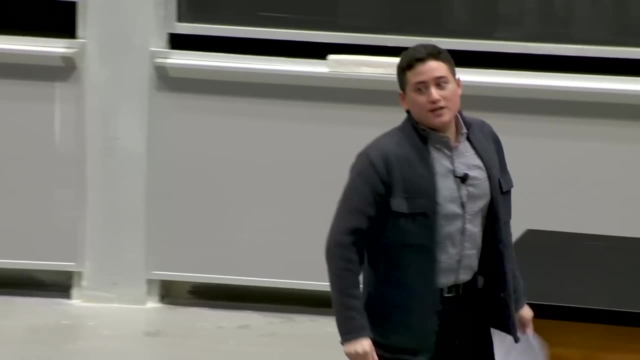 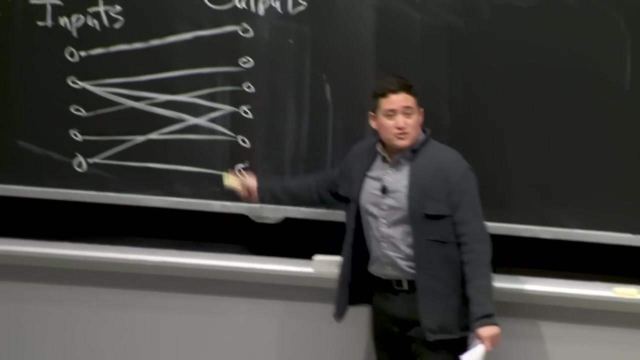 That's usually how we define a problem. If I am checking for whether this index contains a five, I can just go to that array, look at index five or the index you gave me and see if it equals five, right? So usually we're putting it in terms of predicates because in general we don't really want to. 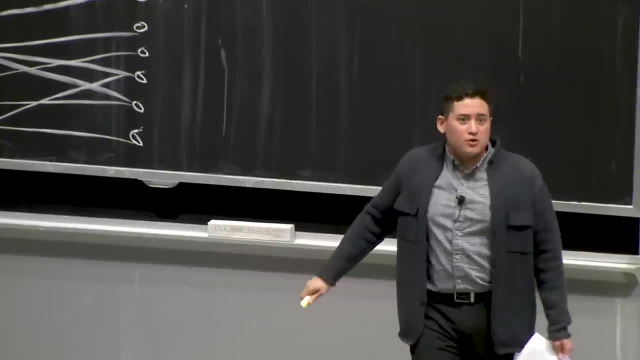 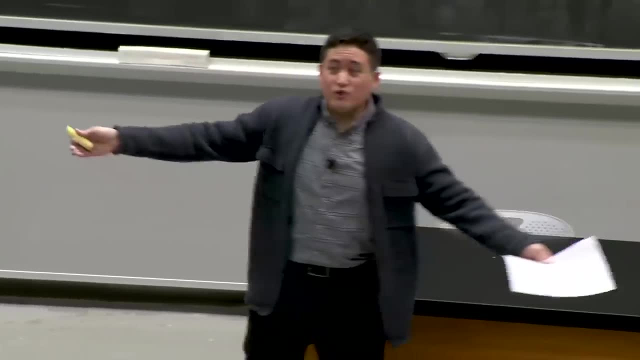 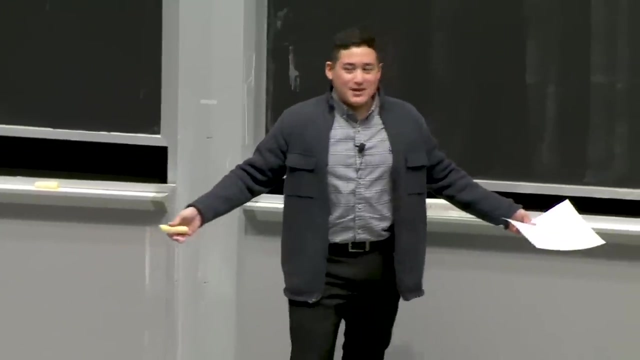 talk about small instances of problems. So let's say I had the problem of among the students in this classroom: Do any pair of you have the same birthday? Okay, All right. Well, probably if there's more than 365 of you, the answer is yes, right. 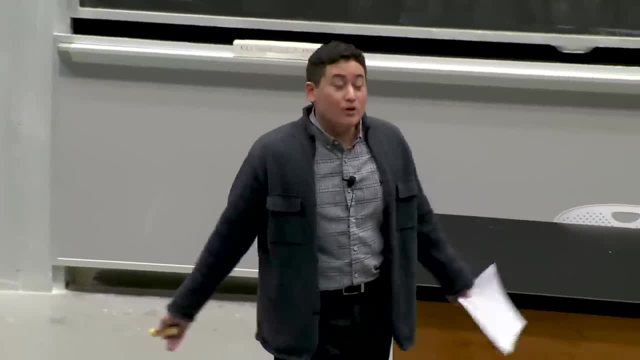 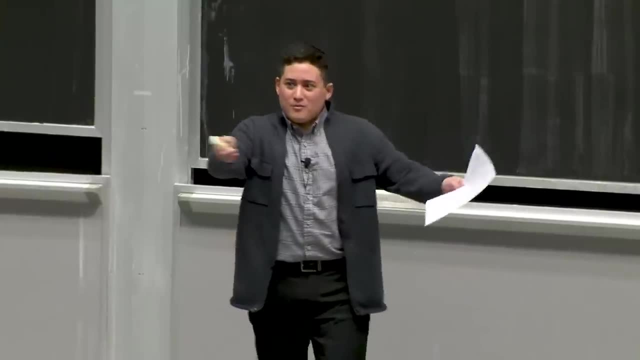 That by what Pigeonhole principle, right? Two of you must have the same birthday, right? But so let's generalize it a little bit. say that, oh, I don't know, I need a bigger space of birthdays for this question to be interesting. 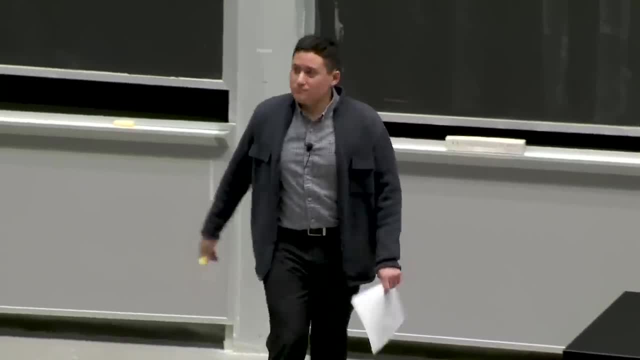 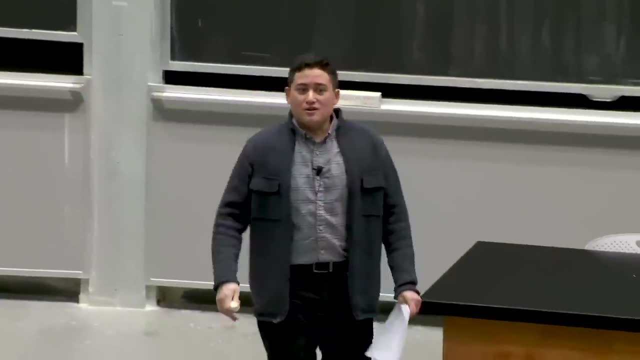 Maybe I tack on the year, Maybe I tack on the hour That you were born, And that's a bigger space of inputs and I wouldn't necessarily expect that two of you would be born in the same year, on the same day, in the same hour, right. 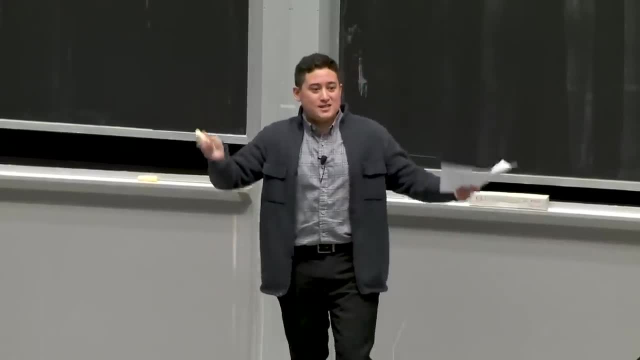 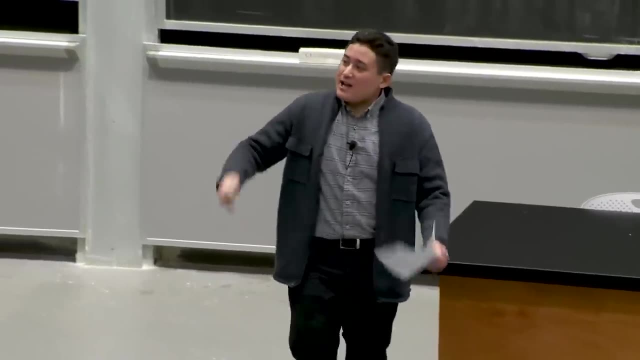 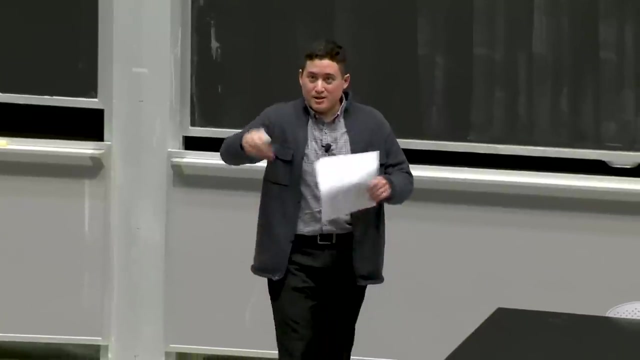 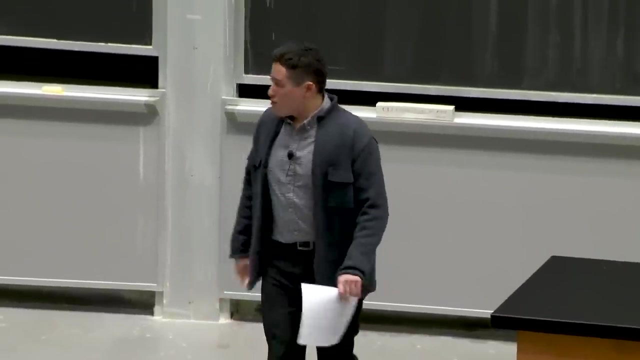 That would be a little less likely. In fact, as long as that space is larger than something like the square of the number of you, right then I'm less likely than even to have a pair of you. That's a, That's kind of a birthday problem. you may have seen in 042, potentially right. 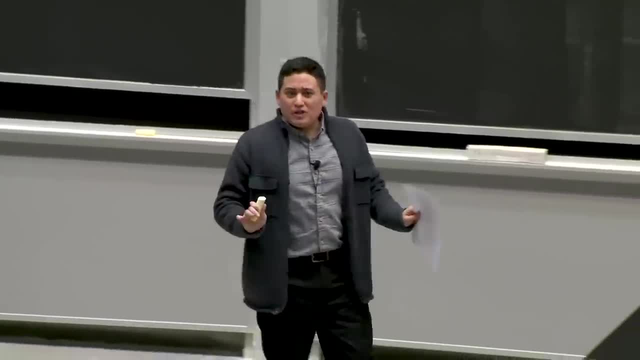 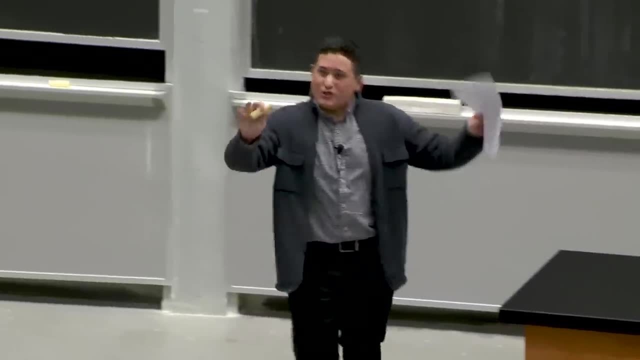 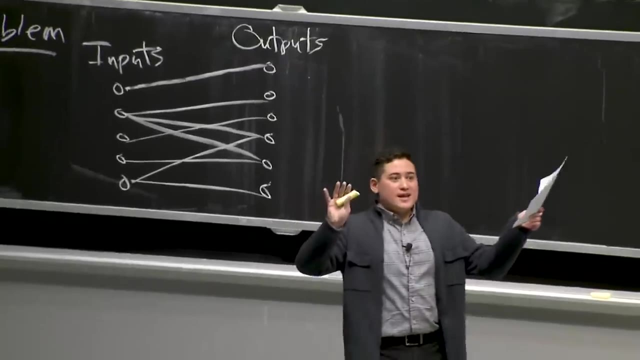 But in general I'm not gonna mess with probability so much here. I want a deterministic algorithm, right, A way of checking whether two of you have the same birth time, let's say Okay. So in general, in this class we're not gonna concentrate on inputs such as: is there a? 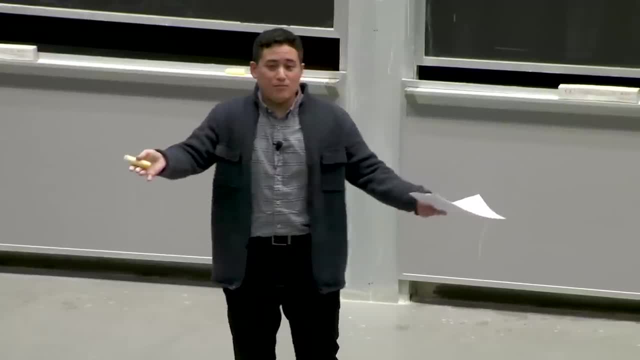 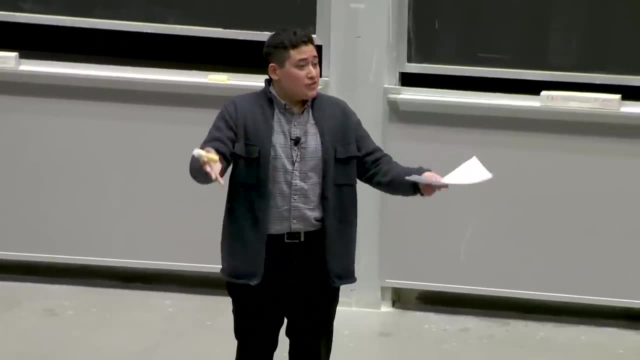 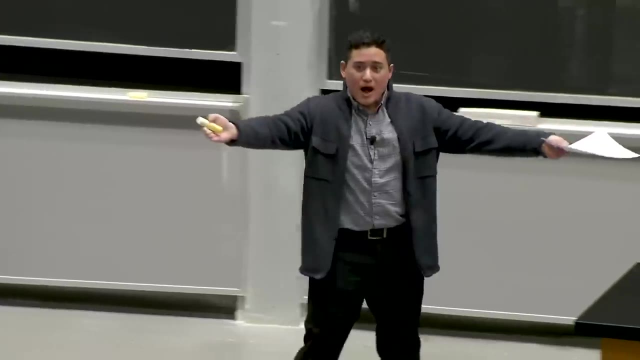 Pay attention. Is there a pair of you in this class that have the same birthday? That's kind of boring, right? I could just say: well, I could do a lot of different things, but what we do in this class, This is for a fixed classroom of you. 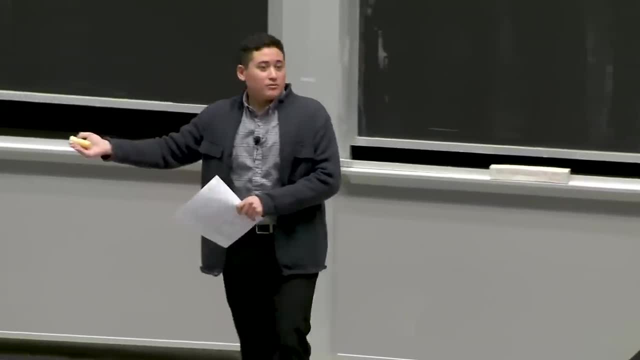 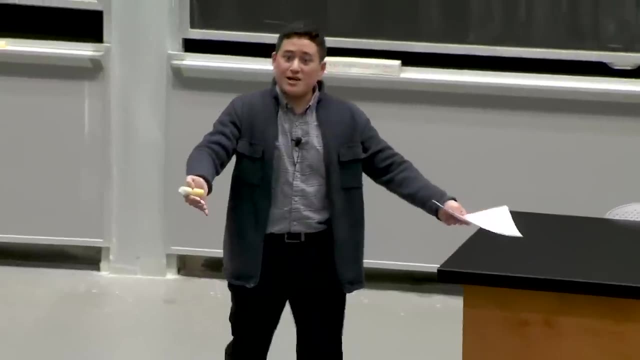 I want to make algorithms that are general to any classroom. right To go to your recitation. I want an algorithm that will apply to your recitation. I want an algorithm that not only applies to this classroom, but also the machine learning class before you. 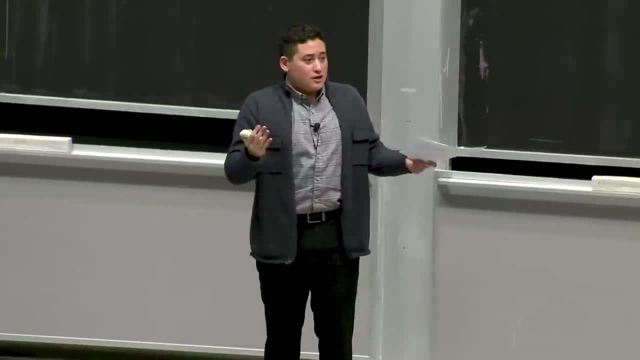 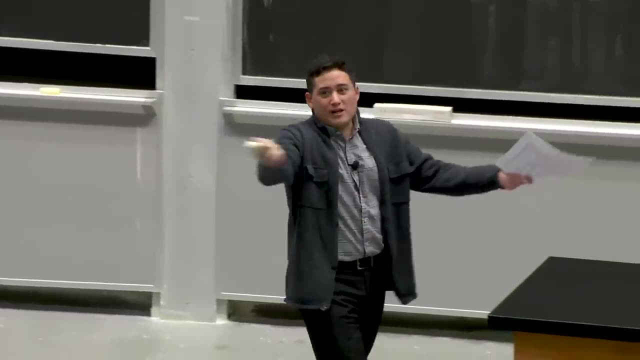 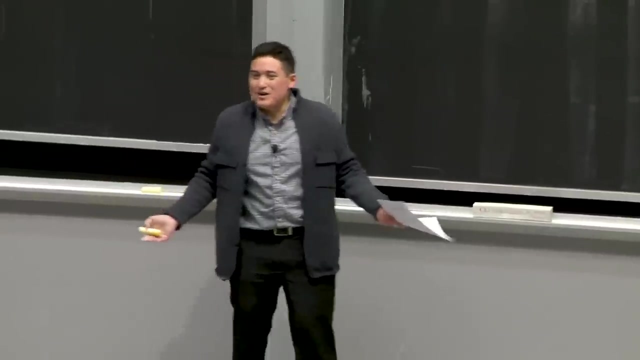 Right. I want an algorithm that can change its. It can accept an arbitrarily sized input, right. Here we have a class of maybe 300, 400 students, right? But I want my algorithm to work for a billion students, right. 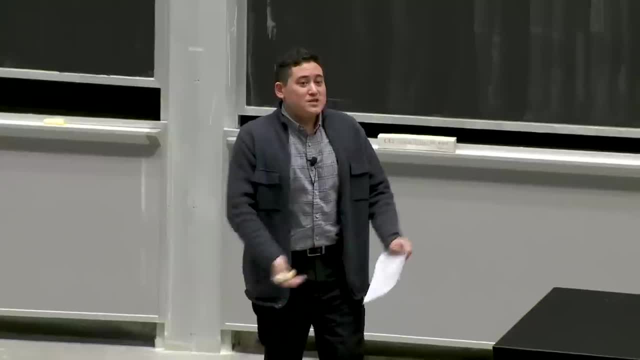 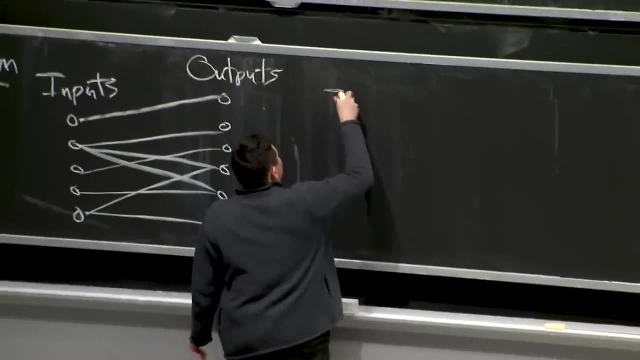 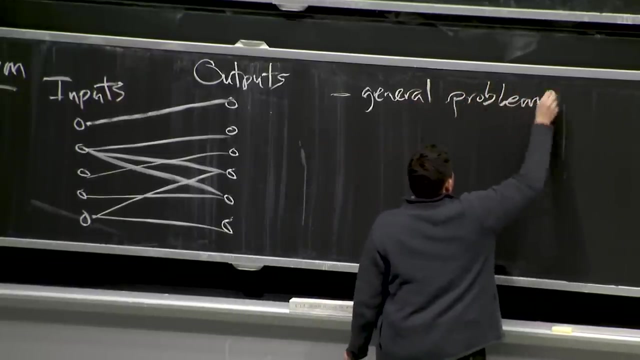 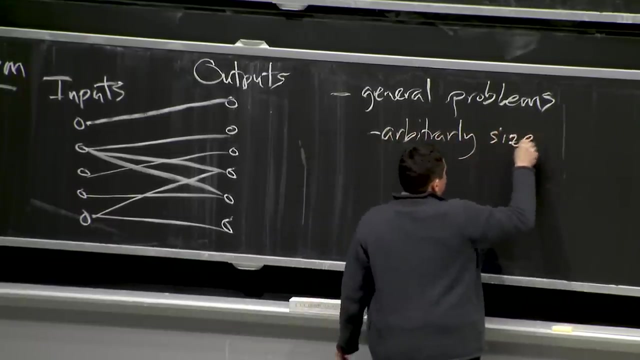 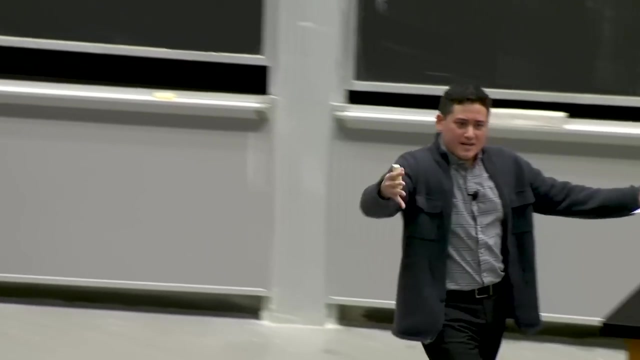 Maybe I'm trying to check if there's a match of something in the Facebook database or something like that, right, Okay, So in general, we are looking for general, General problems that have arbitrarily sized inputs. right, So, these inputs could grow very large, but we want a kind of a fixed size algorithm to 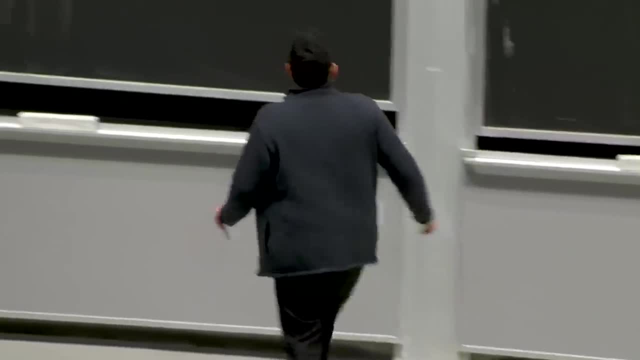 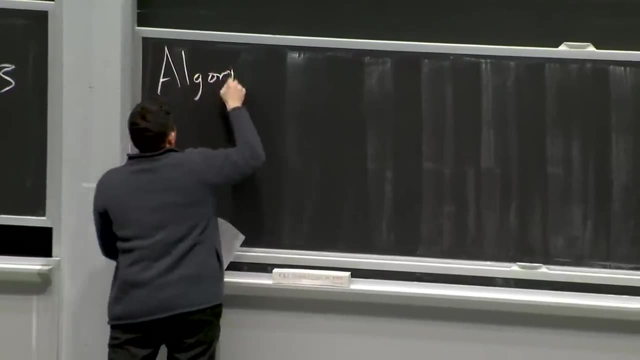 solve those problems. Okay, So what is an algorithm then? Okay, So what is an algorithm then? Okay, Okay, I don't know, I don't know, I don't know. Okay, Okay, Okay, Okay, Okay. 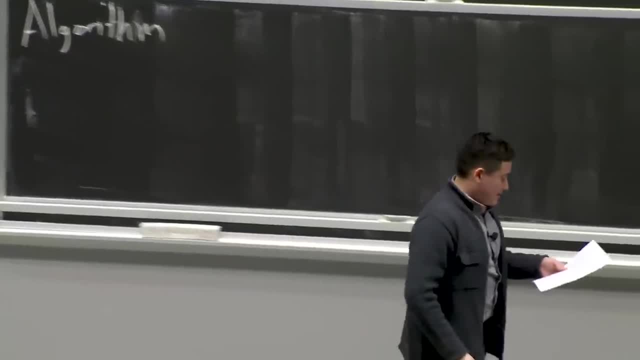 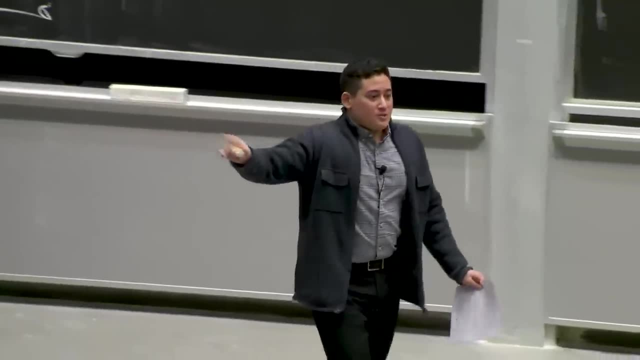 Yeah, No, I really can't spell. I told you Okay, I didn't lie to you. So an algorithm is a little different than a problem, Problem specification. I can state to you what this graph, or I can tell you what this. 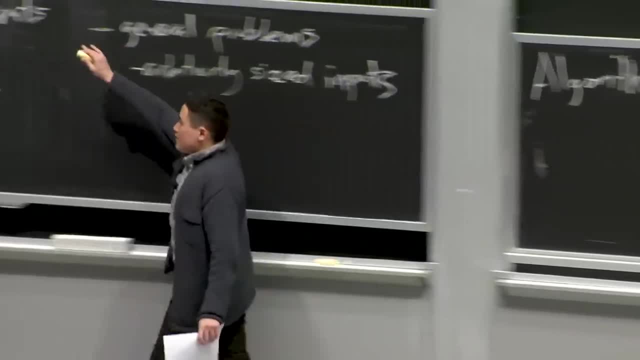 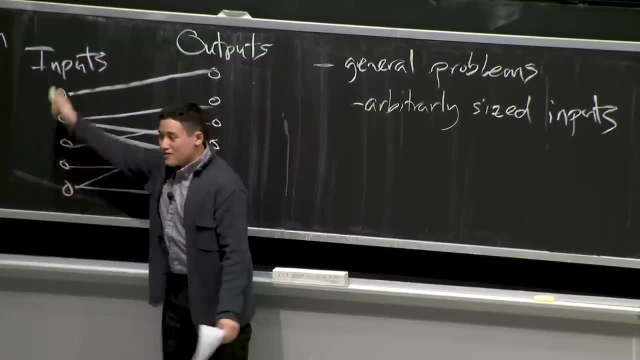 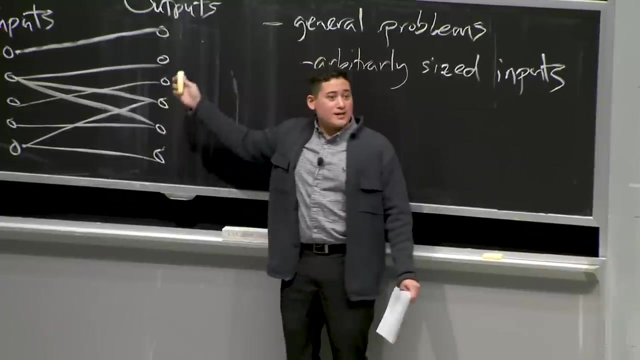 graph looks like An algorithm is really I don't know what the outputs are, I don't know what these edges are. I want a fixed-size kind of machine or procedure that if I give it an input it will generate an output, And if it generates an output, it better be one of these correct outputs. 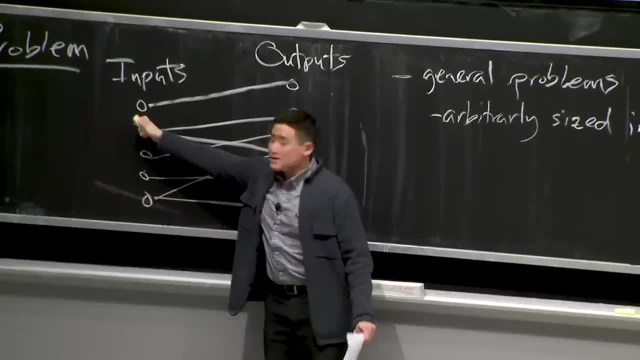 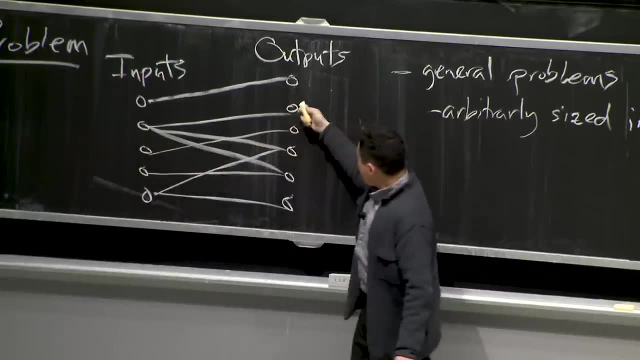 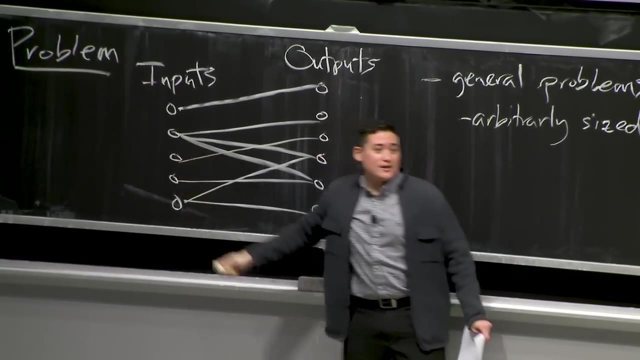 So if I have an algorithm that takes in this input, I really want it to output this output, or else it's not a correct algorithm. Similarly, for this one it could output any of these three outputs, But if it outputs this guy for this input, that would not be a correct. 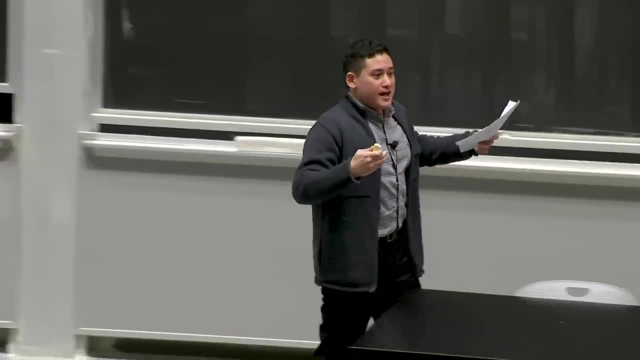 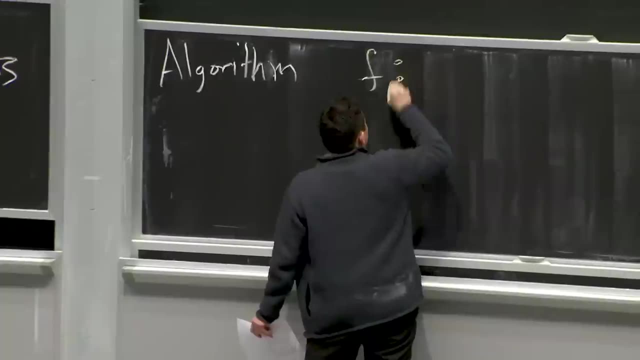 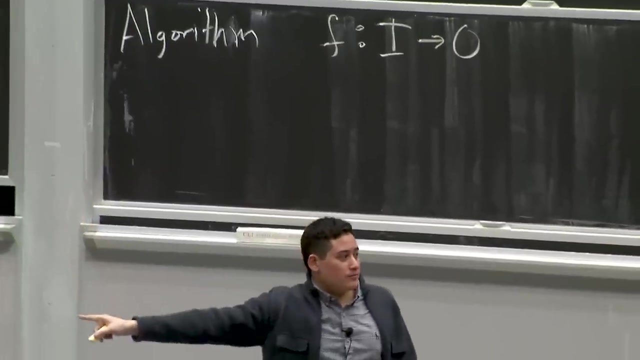 algorithm, And so generally what we want is: an algorithm is a function. It takes inputs to outputs. An algorithm is some kind of function that takes these inputs, maps it to a single output and that output better be correct based on our problem. So that's what our algorithm. 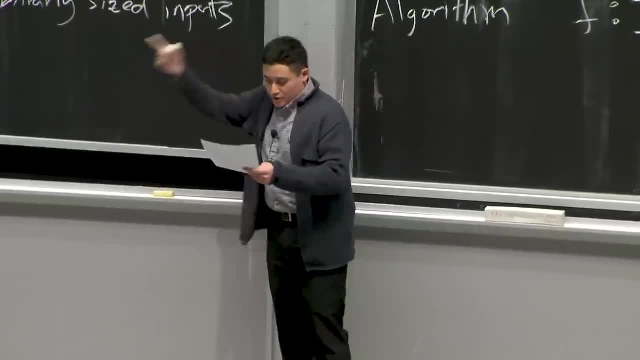 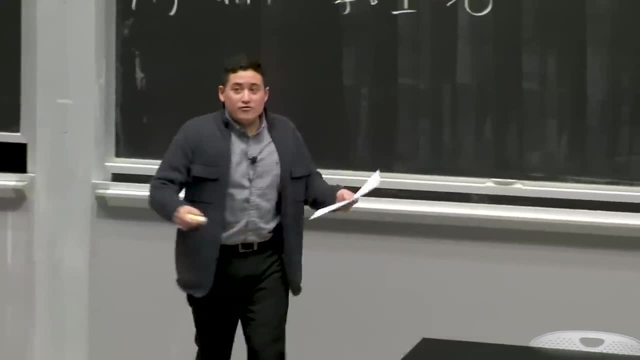 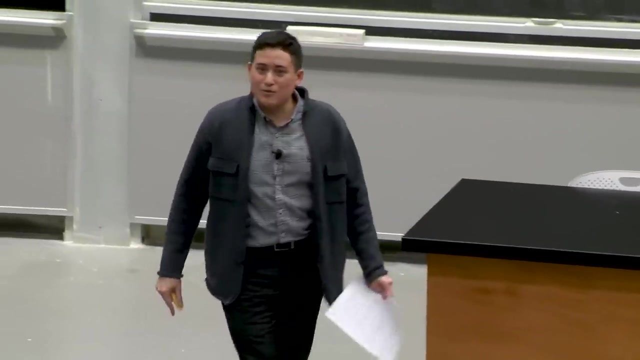 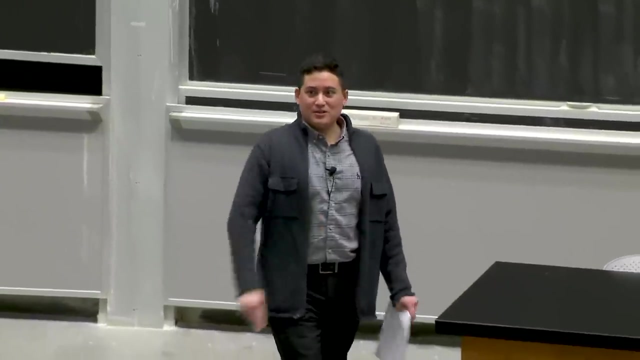 is 0. It solves the problem problem if it returns a correct output for every problem, input that is in our domain And the example for: Does anyone have a possible algorithm for checking whether any two of you have the same birth time as specified before I'm going to let someone else have? 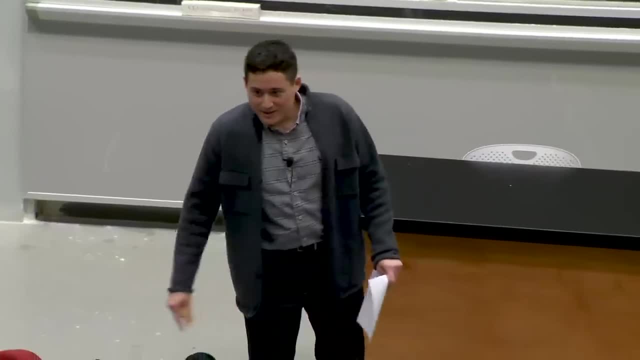 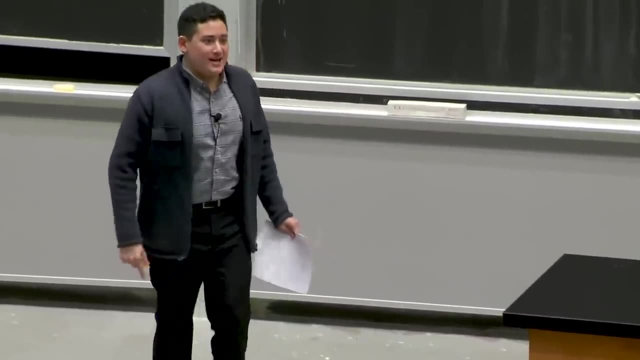 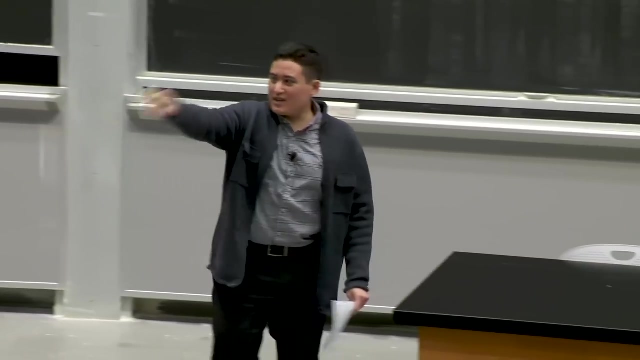 a try. Sure, Ah, great. So what your colleague has said is a great algorithm, but essentially what it's going to do is I'm going to put you guys in some order. okay, I'm going to give each of you a number one through however many number of students there are in this class. 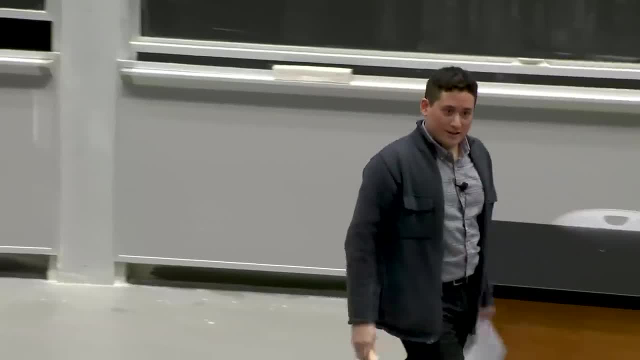 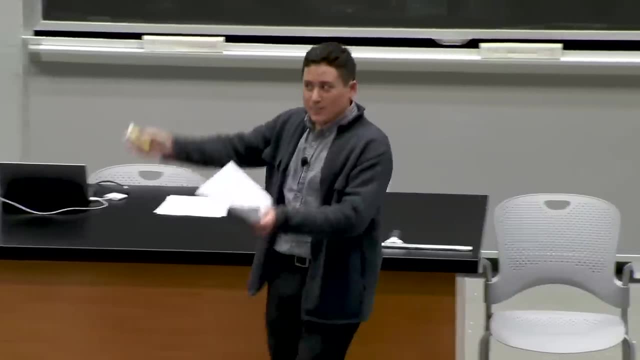 and I'm going to interview you one by one, right, I'm going to say what's your birthday, And then I'm going to write it down, right, I'm going to put it in some kind of format, a record, okay, And then, as I keep interviewing you, I'm going to find out your birthday. 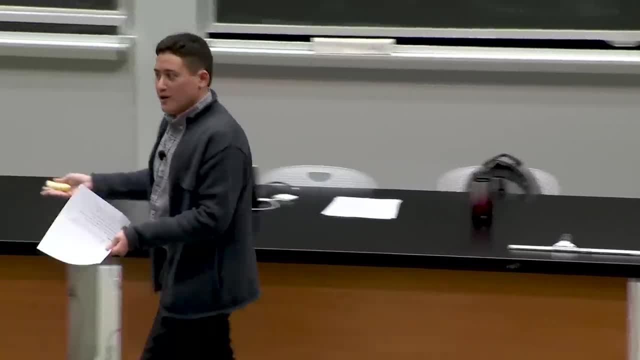 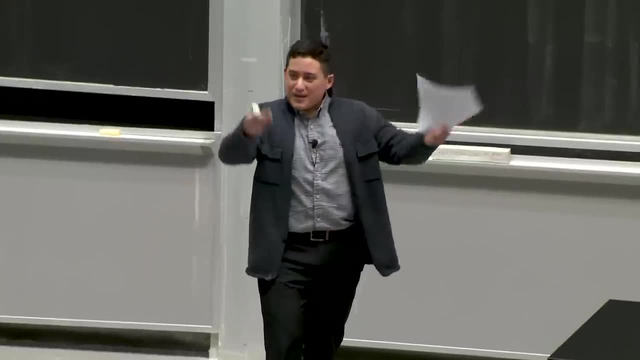 I'm going to check the record. I'm going to look through all the birthdays in the record. if I find a match, right, Then I return. yay, I found a pair and I can stop. Otherwise, if I get through the record list and I don't find a match, I just stick you at the end. 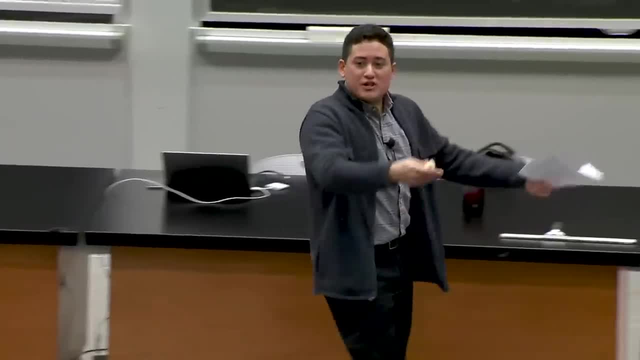 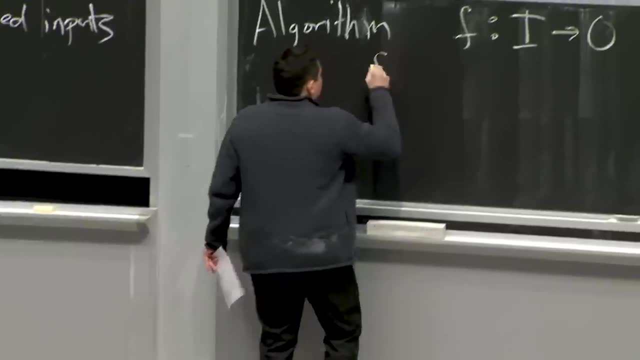 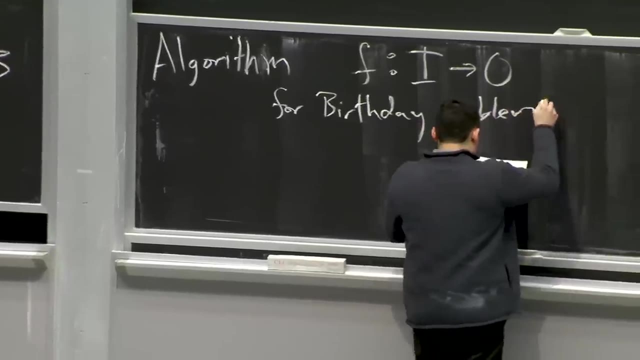 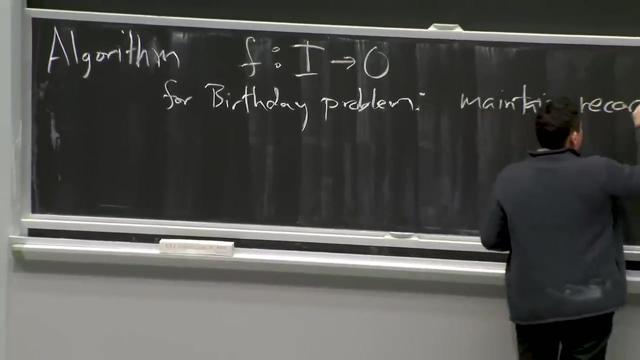 of the record, right? I add you to the record and then I move on to the next person. I keep doing this. Okay, so that's a proposed algorithm for this birthday. For birthday problem, For birthday problem. what's the algorithm here? Maintain a record. 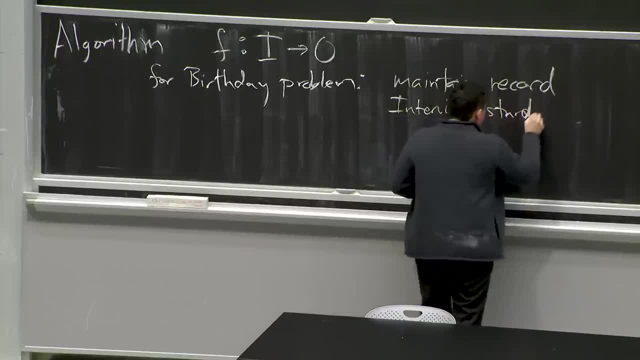 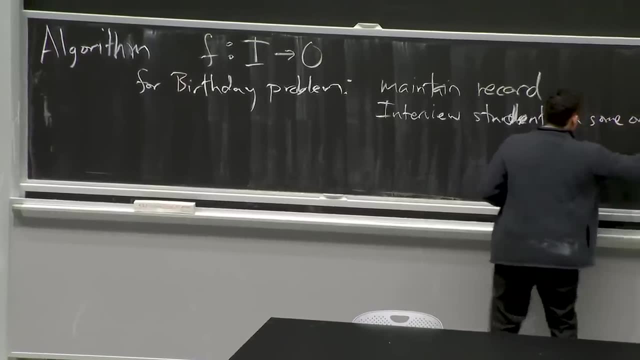 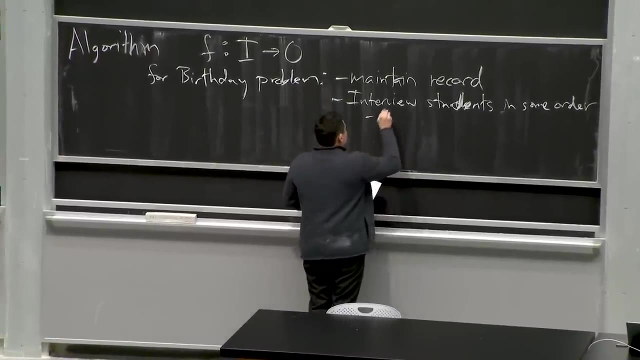 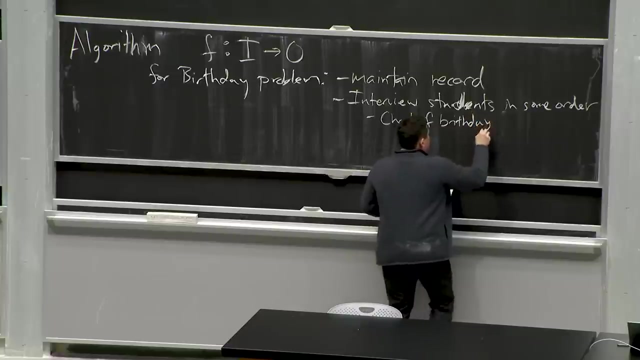 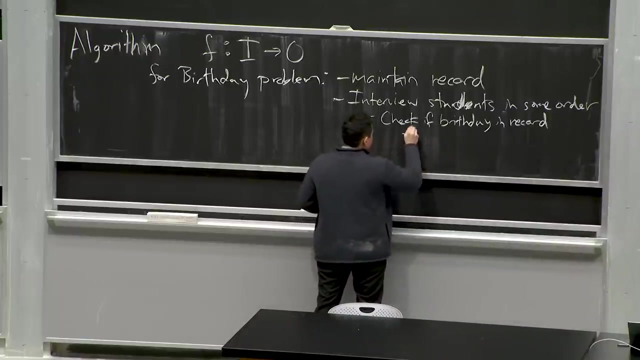 Interview students, students in some order. And what does interviewing a student mean? It means two things. It means check if birthday in record And if it is return a pair, So return pair. Otherwise, return a pair, Otherwise it's going to keep you standing. Okay, so what's the algorithm here? Maintain a record, Maintain a pair, So return a pair Otherwise. return a pair, Otherwise it's going to keep you standing, So return pair, Otherwise it's going to keep you standing. Also, return a pair Otherwise. 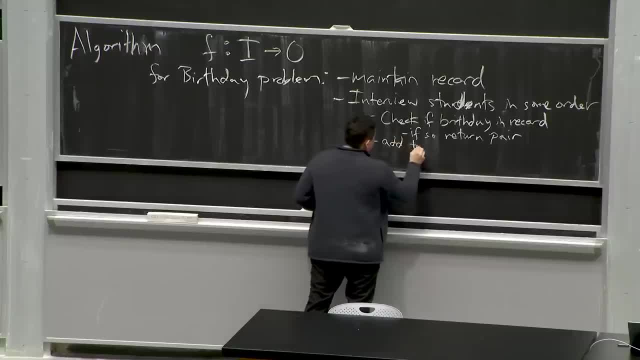 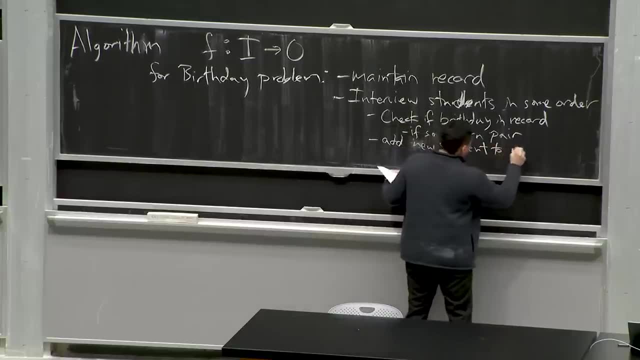 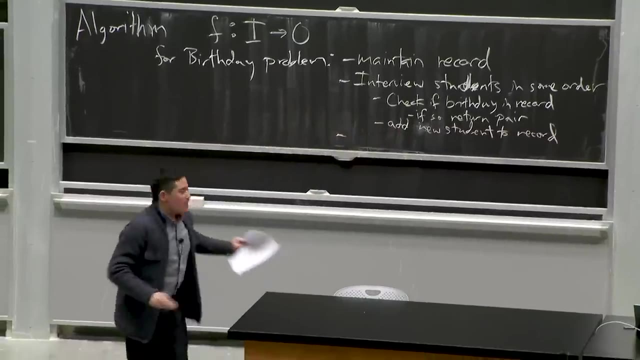 Maintain a pair, Otherwise you have to fix the number if a new character And then you have to Otherwise add a new student to record, And then at the very end, if I go through everybody and I haven't found a match yet, I'm 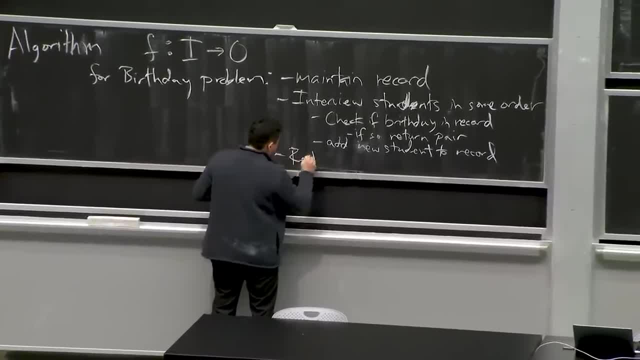 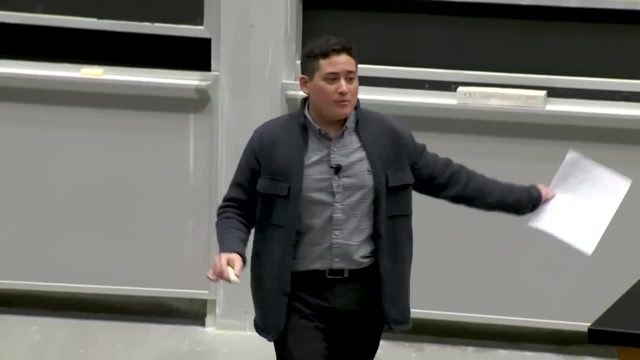 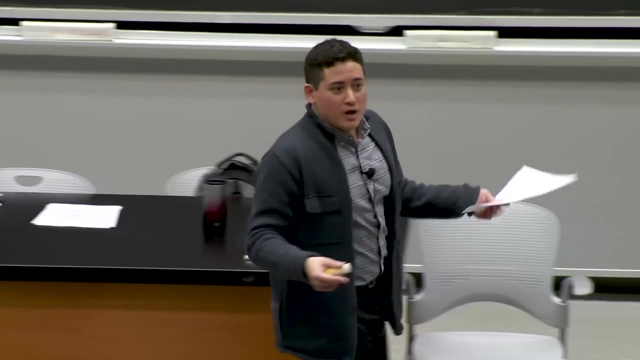 going to return that there is none. OK, so that's a statement of an algorithm. That's kind of the level of description that we'll be looking for you in the theory questions that we ask you on your problem sets. It's a verbal description in words that it's maybe not. 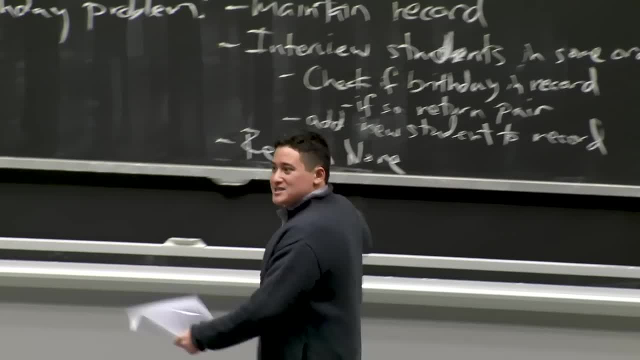 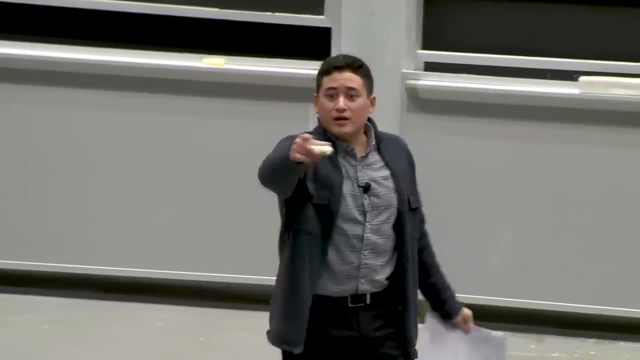 enough for a computer to know what to do. But if you said this algorithm to any of your friends in this class, they would at least understand what it is that you're doing. Yeah, Does an algorithm have to be a pure function in the mathematical system? 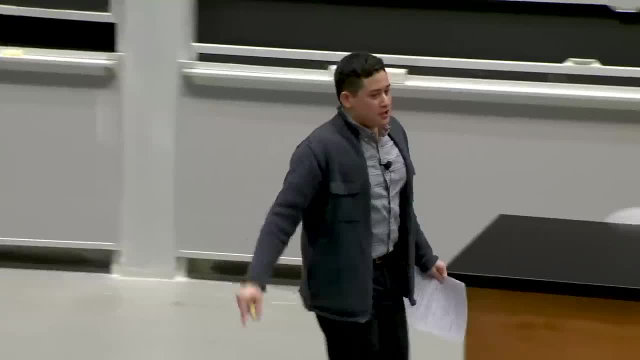 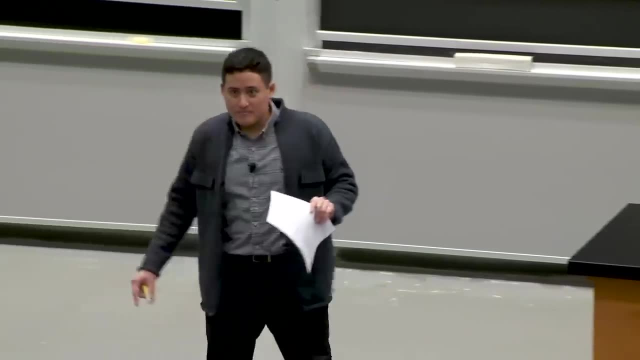 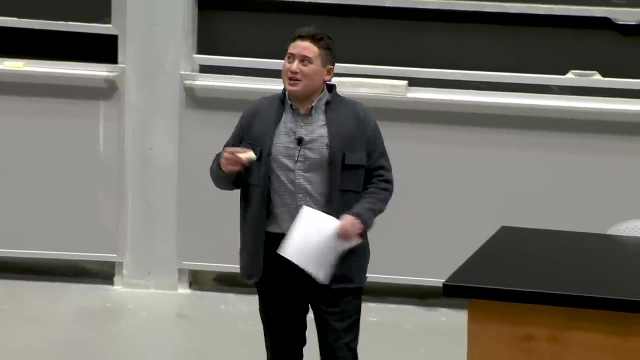 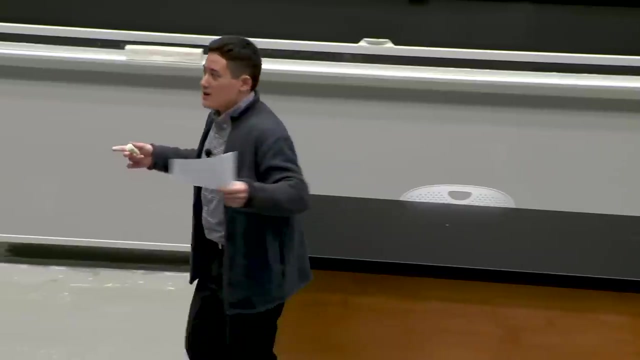 Pure function in the does an algorithm have to be a pure function in the mathematical sense as in it needs to map to a single output? So we're talking about kind of a functional programming definition of a function. right, This is. I am talking about the mathematical. 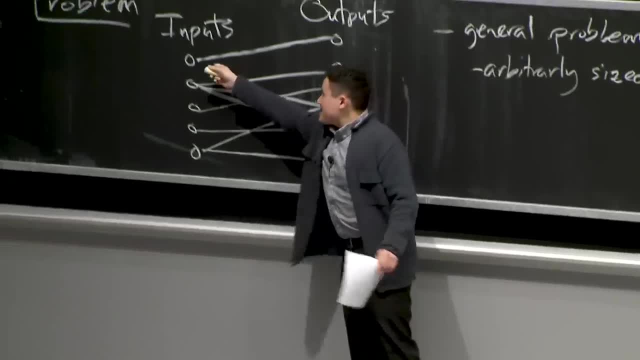 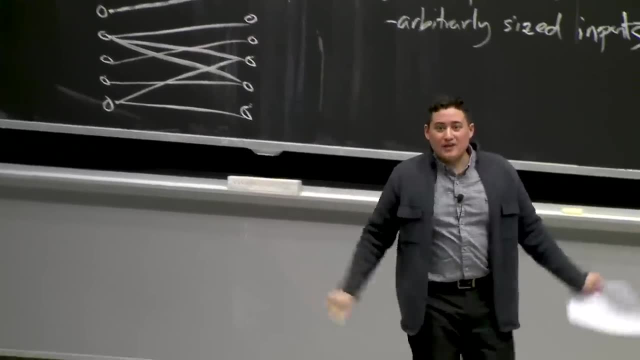 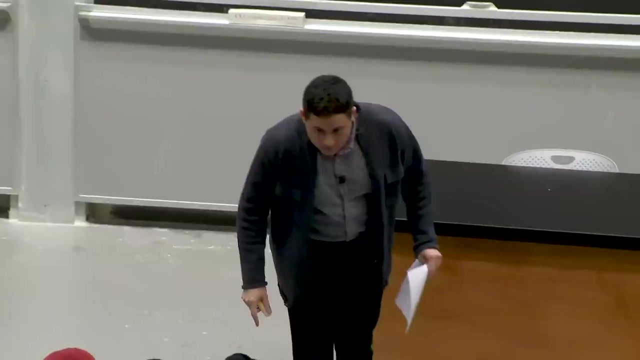 I have a binary relation And this thing has an output for every input, And there is exactly one output to every input. That's the mathematical definition of function that I'm using for when I'm defining an algorithm. Yeah, So basically is an algorithm like a plan? 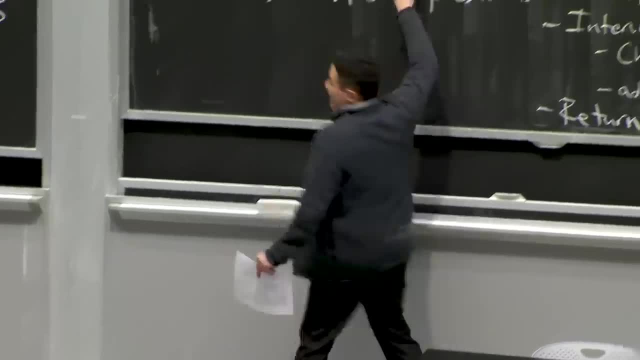 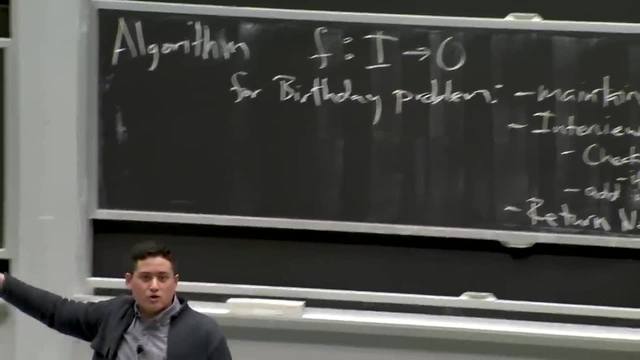 Yeah, an algorithm is a procedure that somehow I can do whatever I want, but I have to take one of these inputs and I have to produce an output And at the end it better be correct, Right? So it's just a procedure. 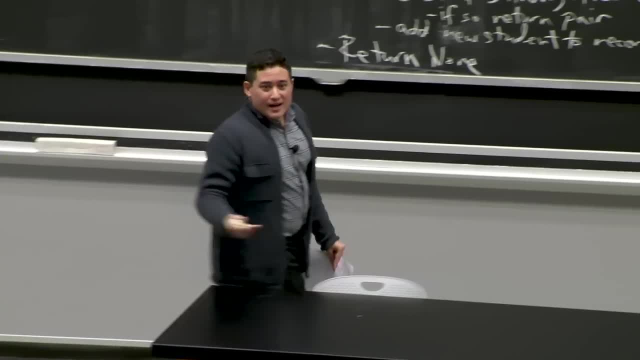 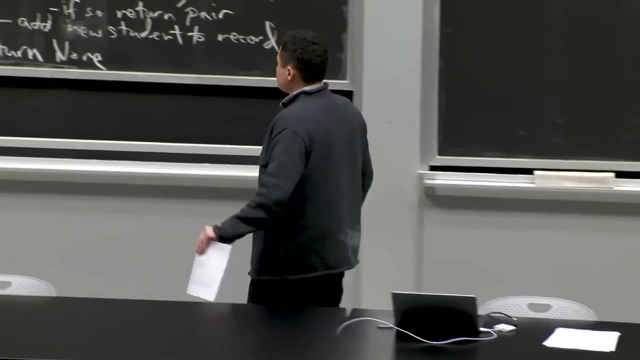 You can think of it as like a recipe. You can think of it as it's just some kind of procedure. Right, It's a sequence of things that you should do, And then at the end, you will return an output. OK, 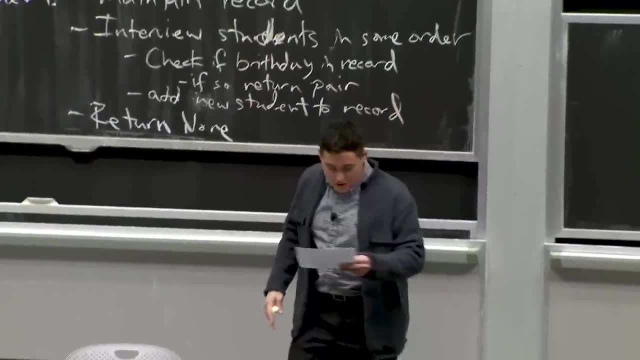 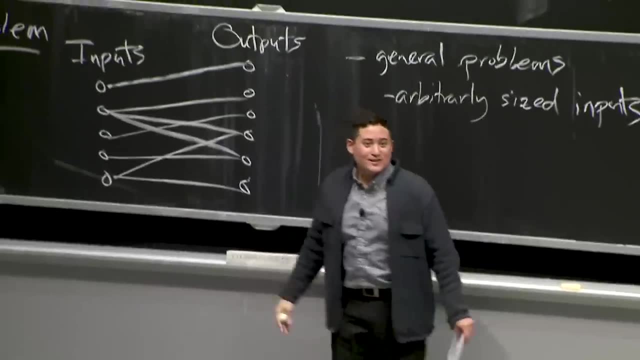 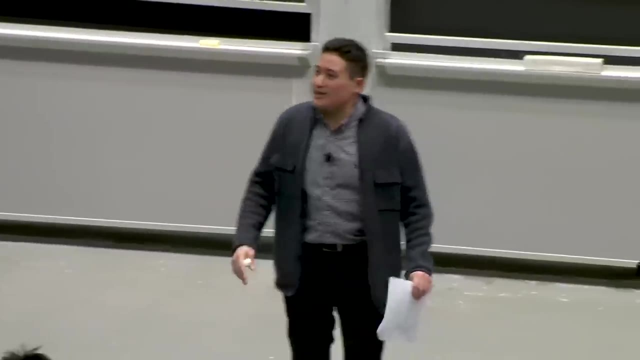 So here's a possible algorithm for solving this birthday problem. OK, Now I have given you what I argue to you, or I'm asserting to you, is a solution to this birthday problem, And maybe you guys agree- Yeah, You agree with me- and maybe some of you don't. 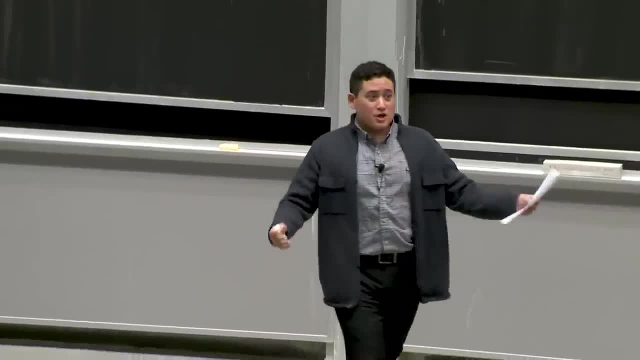 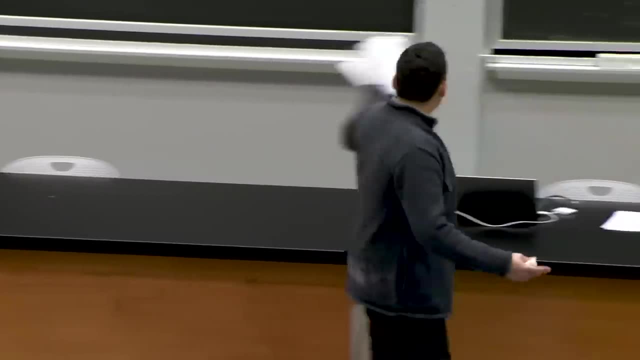 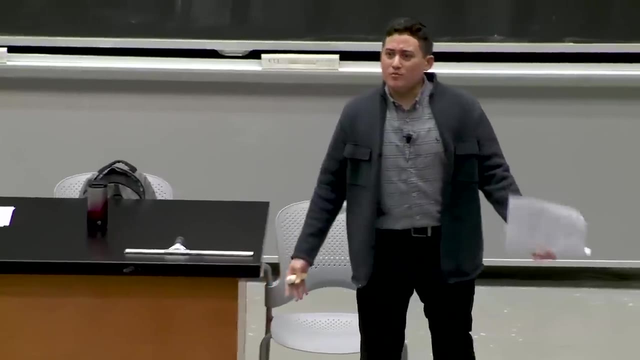 Right. So how do I convince you that this is correct, Right? Well, if I had you know, if I was just running this algorithm on, say, the four students in the front row here, I could argue it pretty well to you. 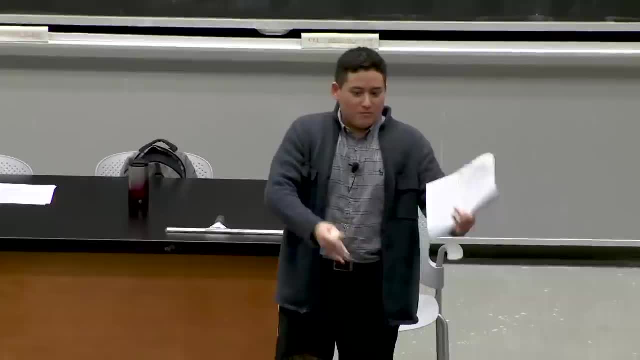 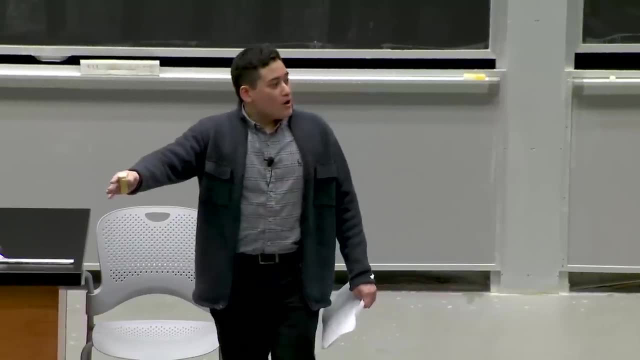 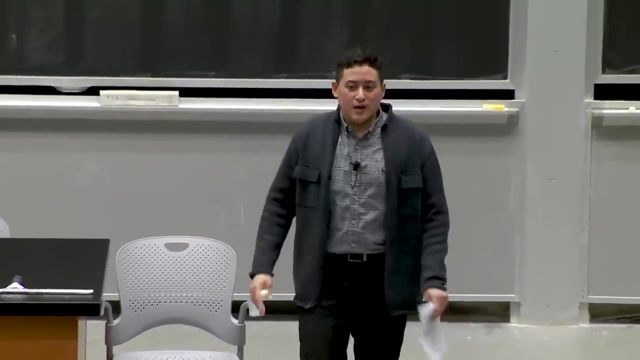 I could go through every you know. I could assign these four people birthdays in various combinations Of either they're none of them have the same birthday, Some two of them have the same birthday. I could try all possibilities And I could go through lots of different possibilities. 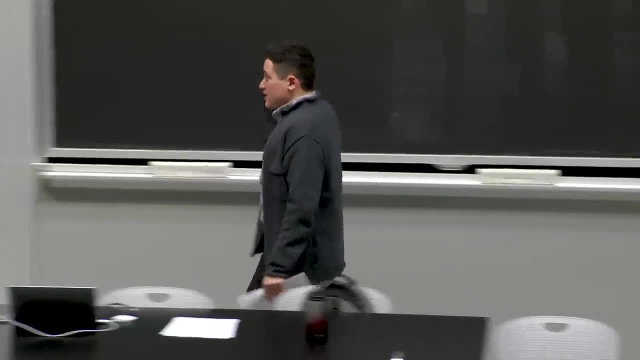 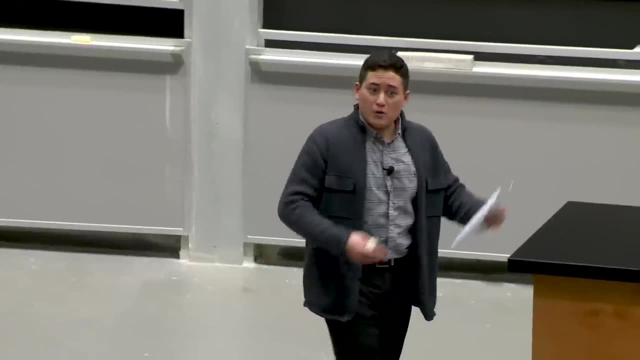 I could check that this algorithm returns the right answer in all such cases. Right, But when I have, I don't know, 300 of you, that's going to be a little bit more difficult to argue, And so if I want to argue something, 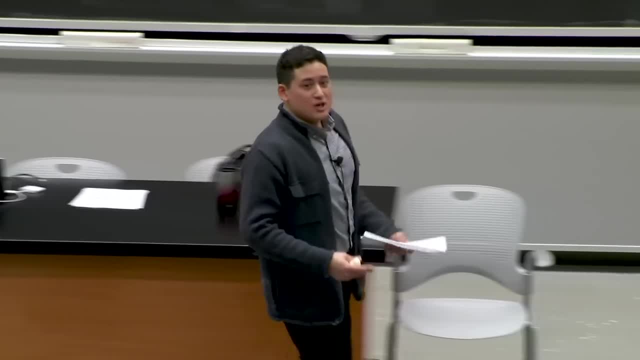 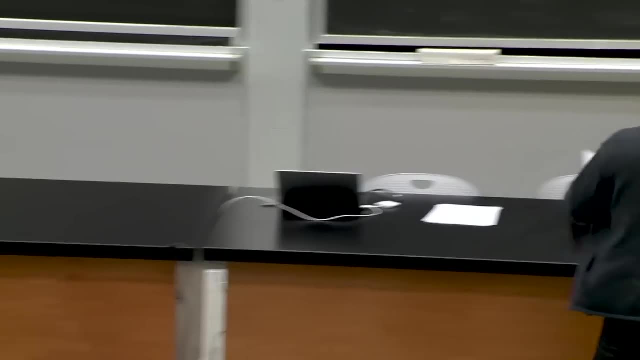 is correct in mathematics. I want to prove something to you for some large value. what kind of technique do I use to prove such things? Yeah, Yeah, Induction right. And, in general, what we do in this class, what we do. 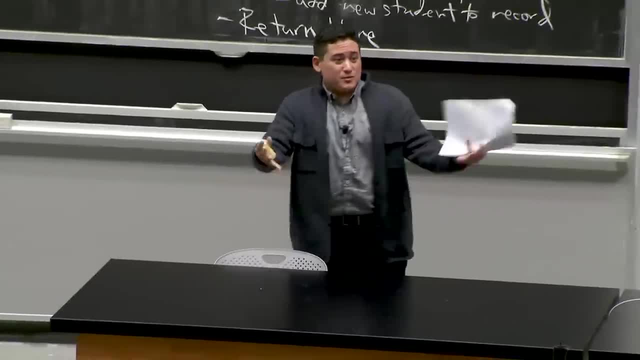 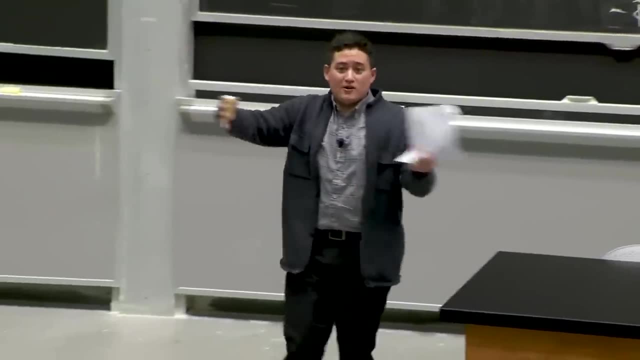 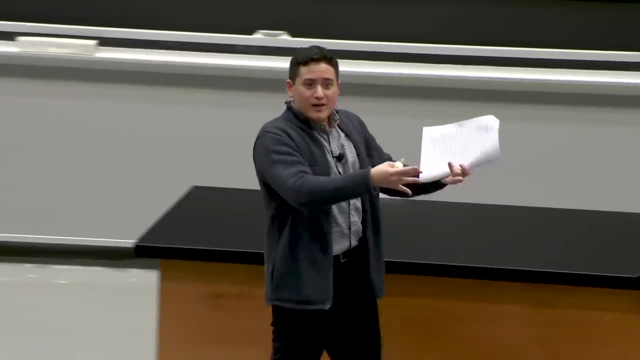 as a computer scientist is we write a constant size piece of code, right? that can take on any arbitrarily large size input, right? If the input can be arbitrarily large but our code is small, then that code needs to loop or recurse or repeat. 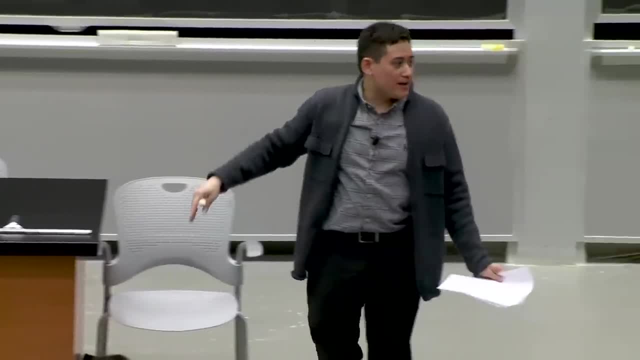 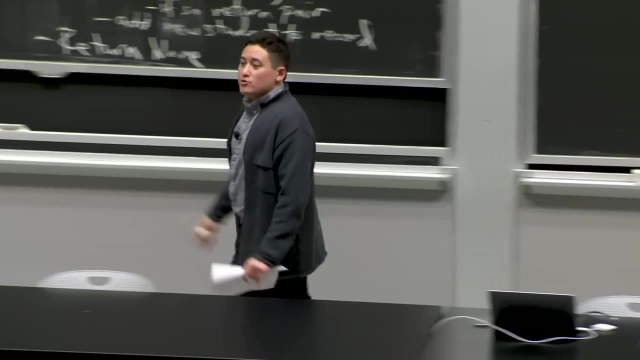 some of these lines of code In order to just read that output right, And so that's another way you can arrive at this conclusion that we're going to probably need to use recursion induction, and that's part of the reason why we ask you to take a course on proofs. 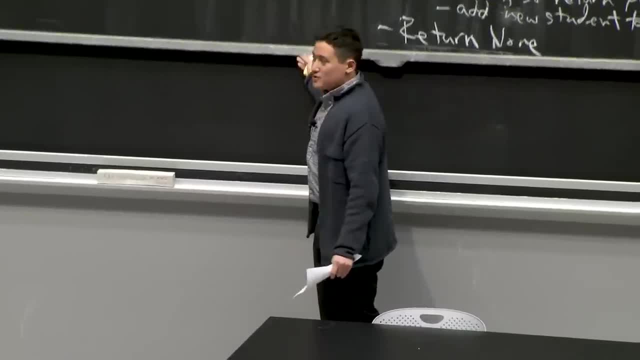 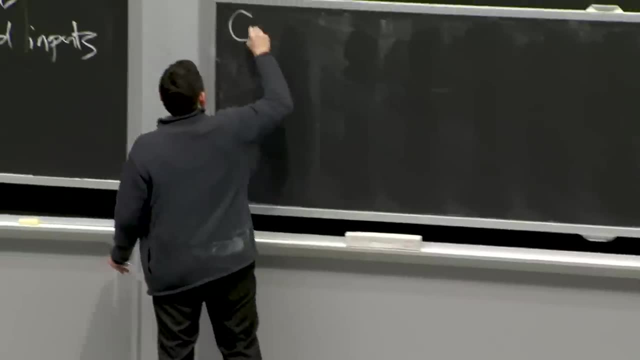 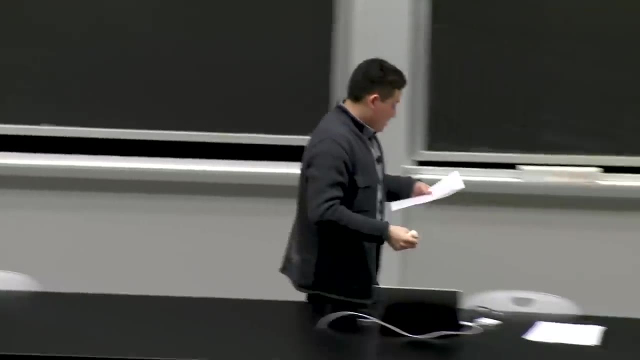 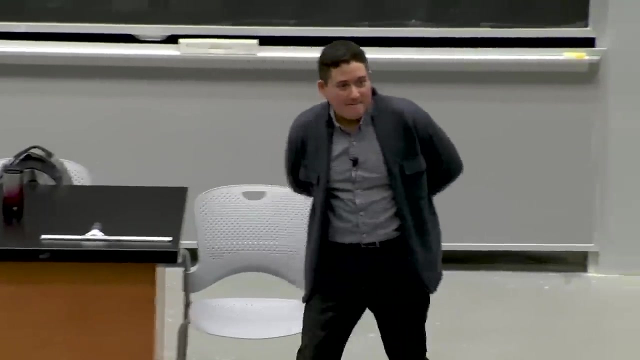 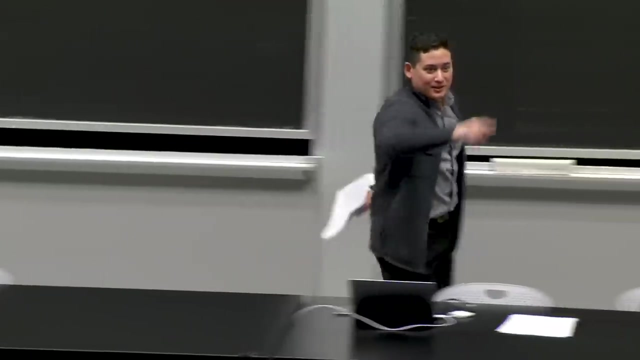 and inductive reasoning and discrete mathematics before this class. OK, So how do we prove that this thing is correct? We've got to use induction. So how can we set up this induction? What do I need for an inductive proof? Sure, 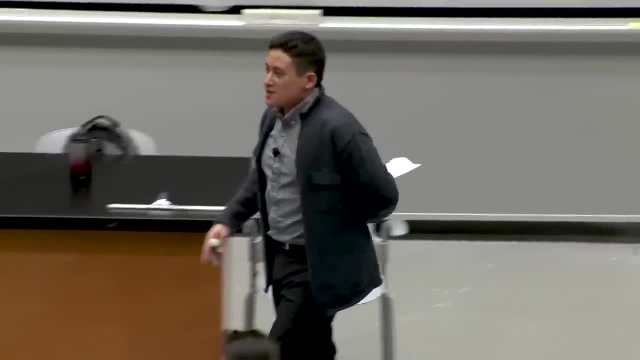 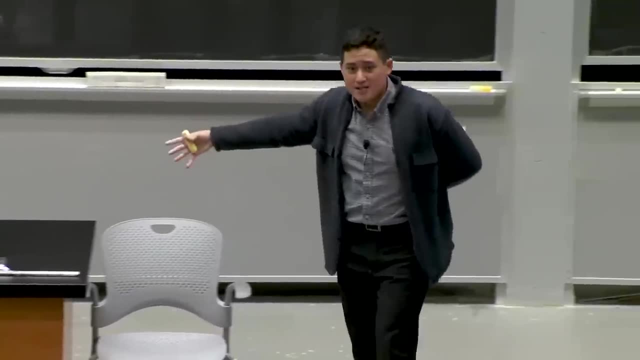 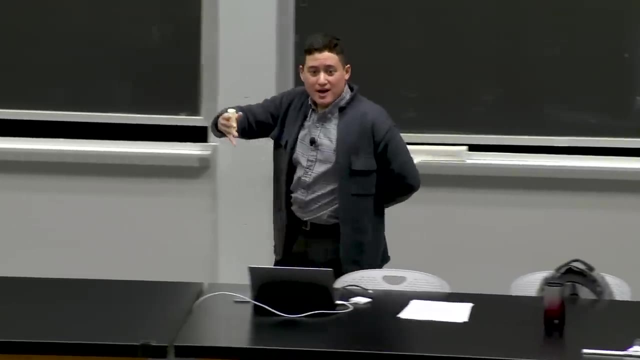 Base case. we need a base case. We need some kind of predicate, yeah, but we need some kind of statement of a hypothesis, of something that should be maintained, OK. And then we need to have an inductive step which basically says: I take a small value of this thing. 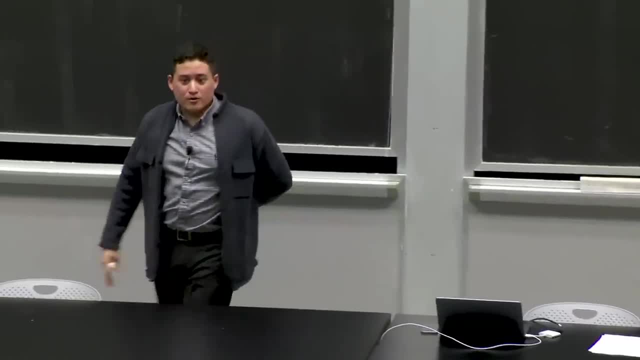 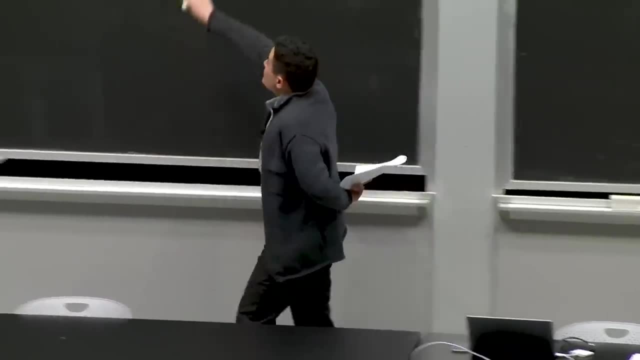 I use the inductive hypothesis and I argue it for a larger value of my well-ordered set that I'm inducting over right. OK, So for this algorithm, if we're going to try to prove correctness, what I'm going to do, 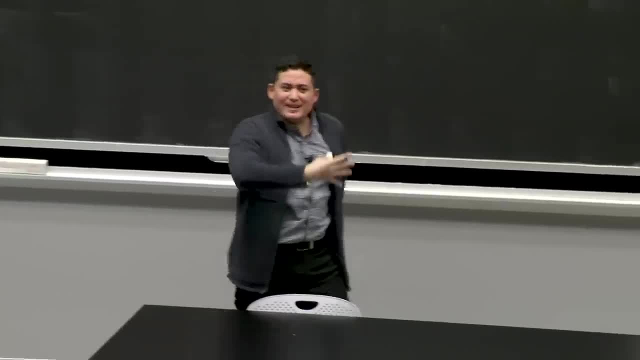 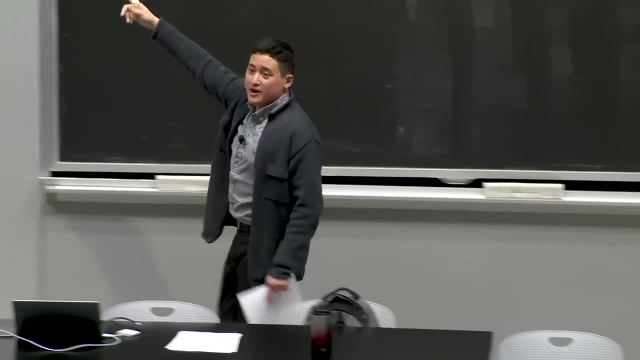 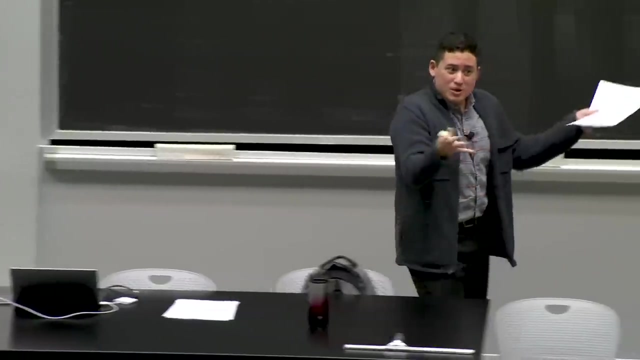 is I'm going to? what do I want to prove for this thing? That, at the end of interviewing all of you, that my algorithm, it, has returned with a pair that match, or if we're in a case where there wasn't a pair somewhere? 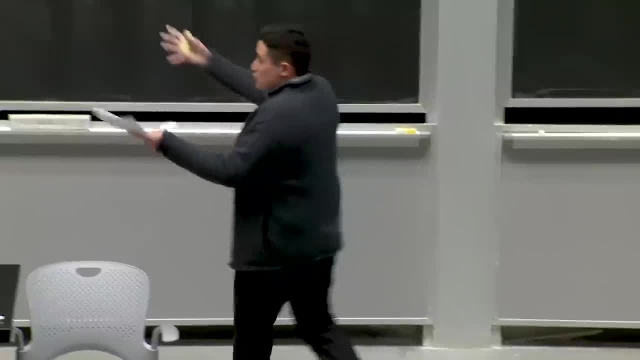 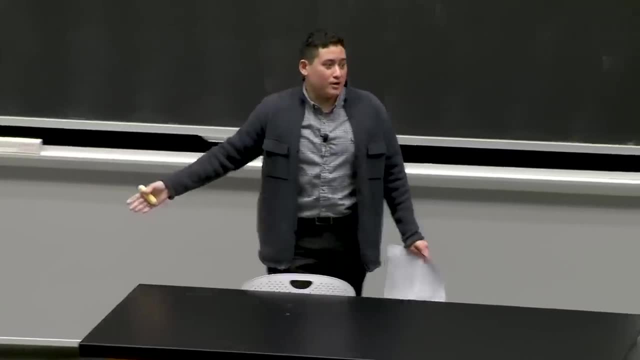 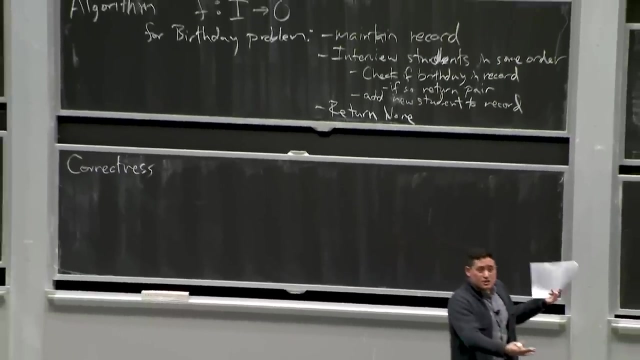 in my set that it returned none. right, That would be correct, right? So how can I generalize that concept to make it something I can induct on right? What I'm going to do is I'm going to say, let's say, after I've interviewed the first k students, right? 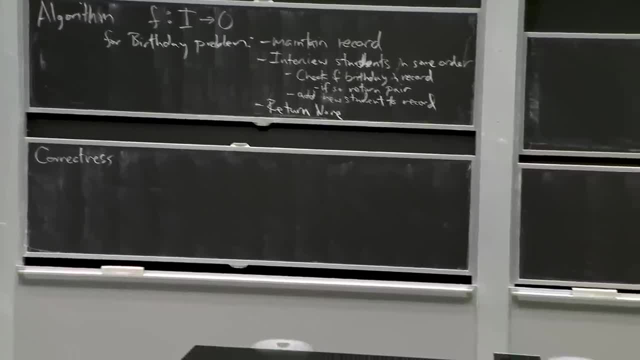 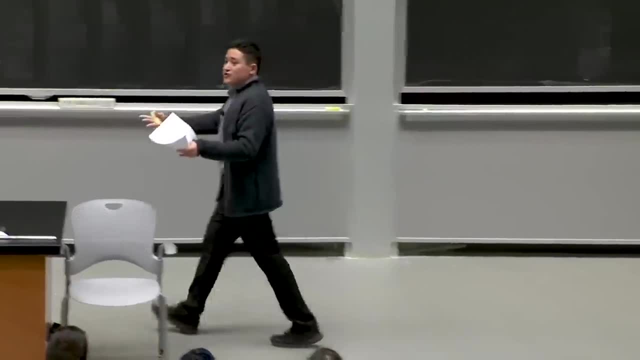 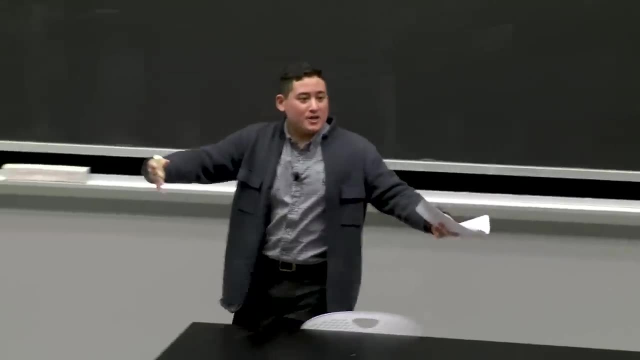 OK, And if there was a match in those first k students, I want to be sure that I've returned a pair right? Because if, after I interview all of you, I've maintained that property, then I'll be sure at the end of the process. 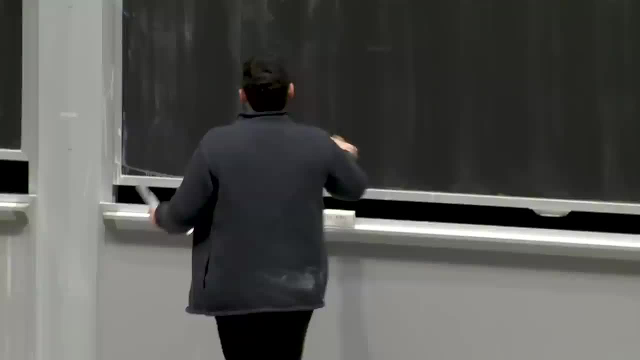 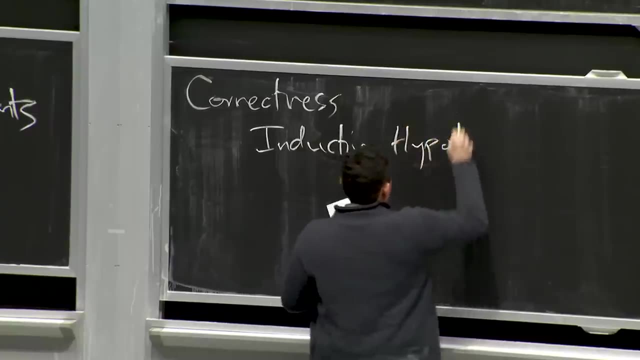 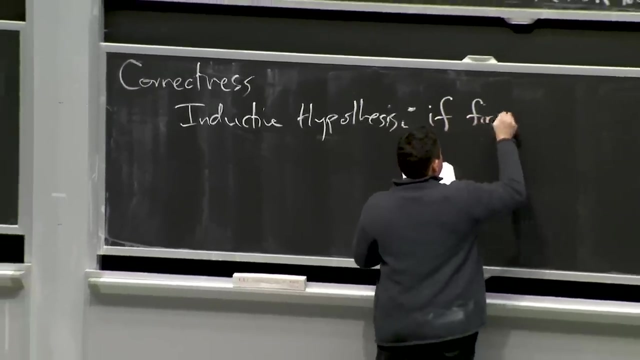 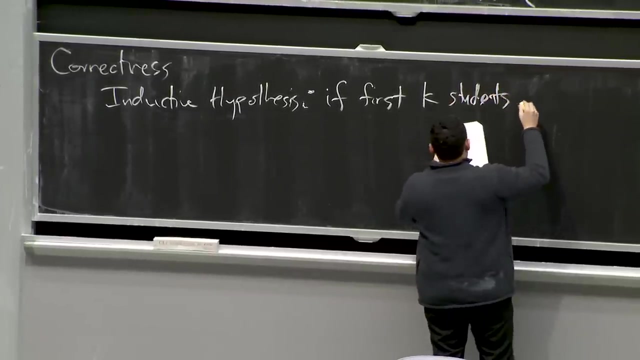 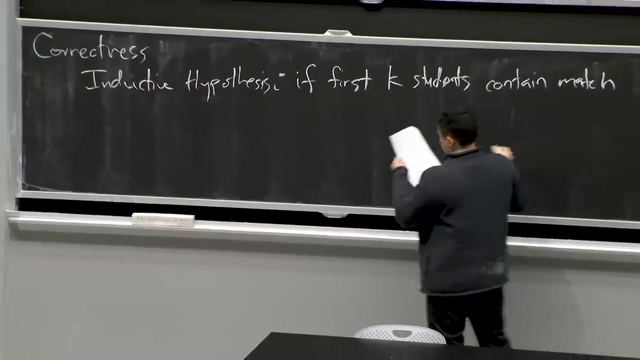 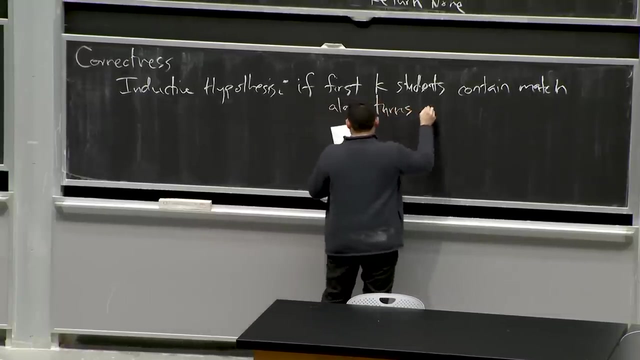 I will have returned a pair if one exists. So here's going to be my inductive hypothesis: OK, If first k students contain a match, algorithm returns a match before. OK, Let's see, Let's see, Let's see. 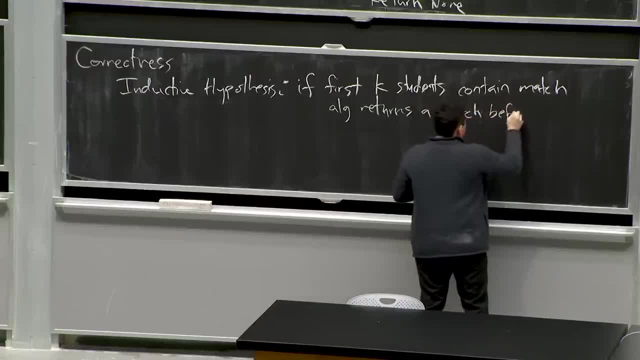 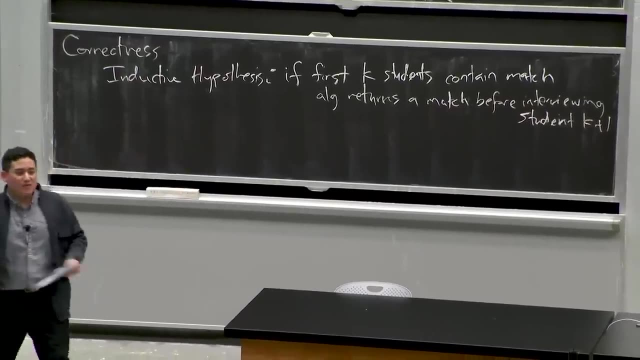 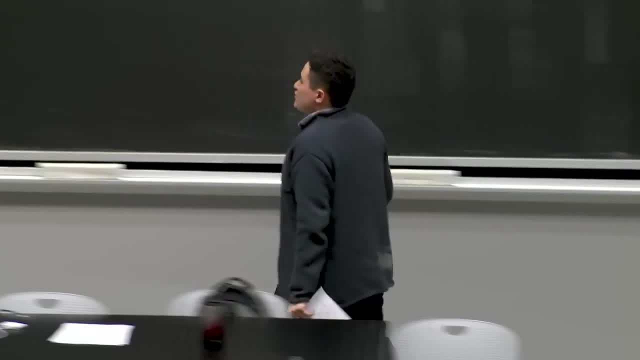 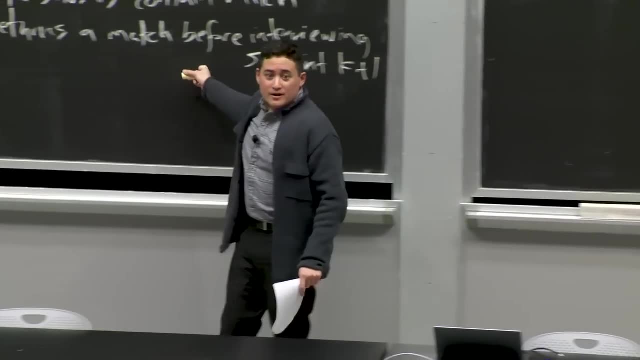 right and at the end of my thing. I'm trying to interview student n plus 1.. Oh, student n plus 1 is not there. If I have maintained this, Then if I replace k with n, then I will have returned a match before interviewing. 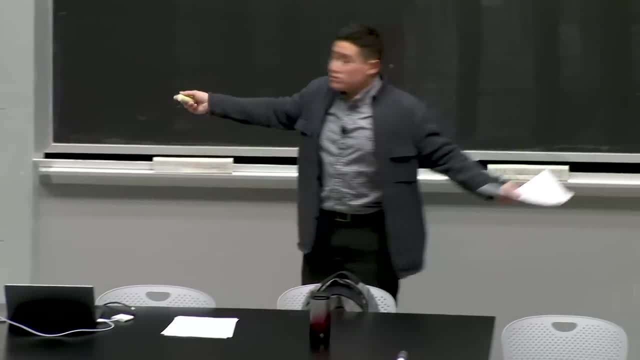 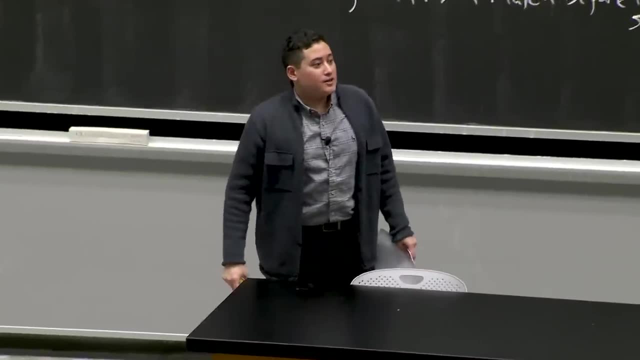 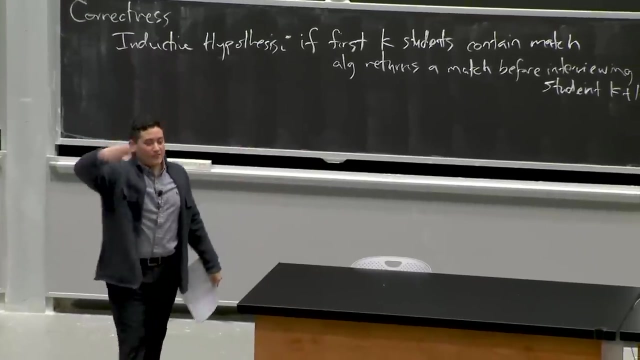 the last student, or when I have no more students left, And then this algorithm returns none, as it should. right, OK, so this inductive hypothesis sets up a nice variable to induct on right. This k I can have, increasing up to n. 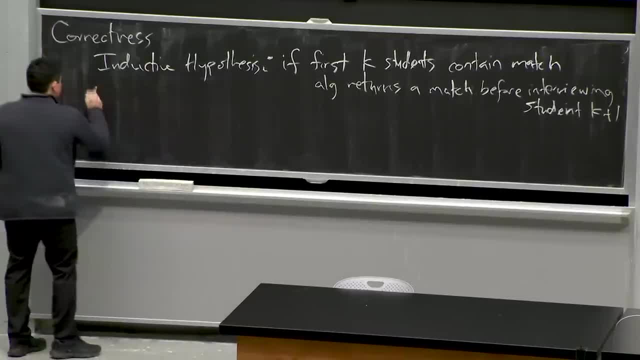 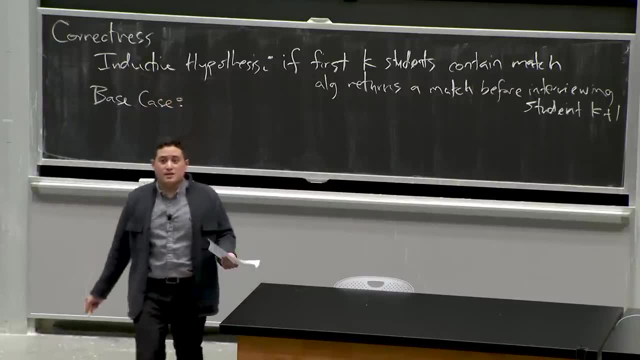 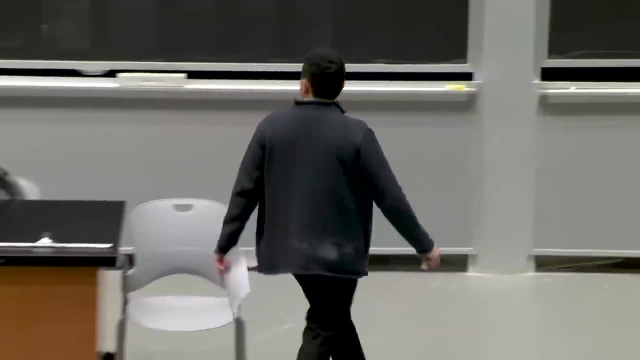 starting at some base case. So what's my base case here? My base case is the easiest thing I can do. sure, 2, that's an easy thing I could do. I could check those possibilities, but there's an even easier base case, yeah. 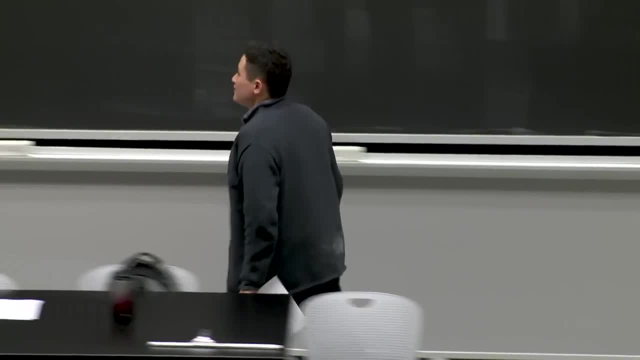 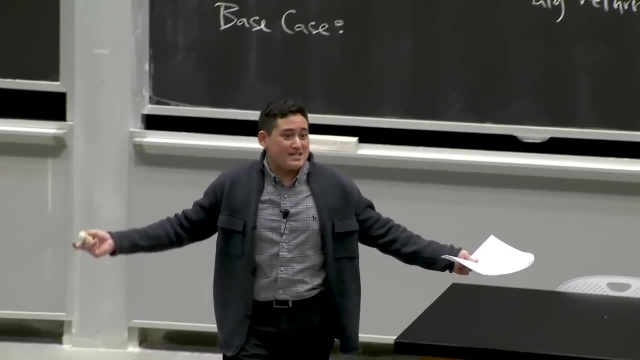 There's an even easier base case than 1. 0, right After interviewing 0 students, I haven't done any work right. Certainly the first 0. 0.. 0. 0 can't have a match right. 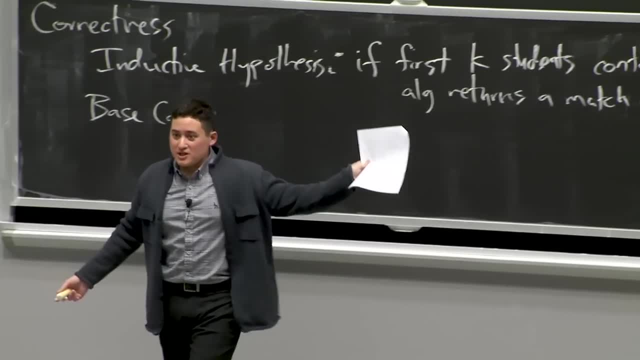 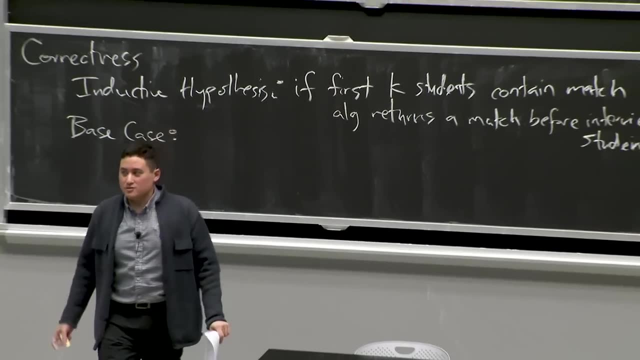 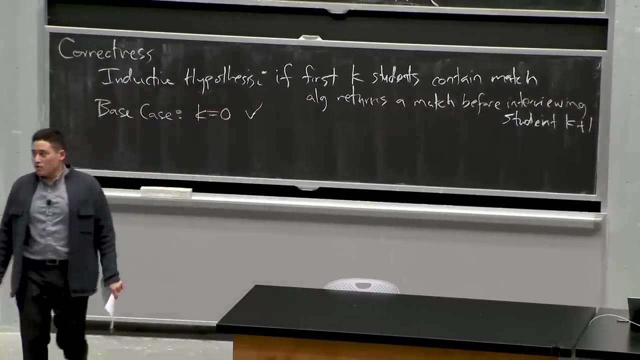 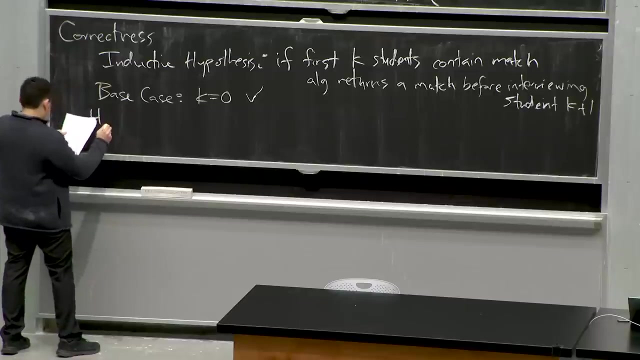 And so this predicate, this inductive hypothesis, is true, just because this initial predicate is false, right? So I can say: base case 0, check. Definitely this predicate holds for that. OK, now we get to go for the meat of this. 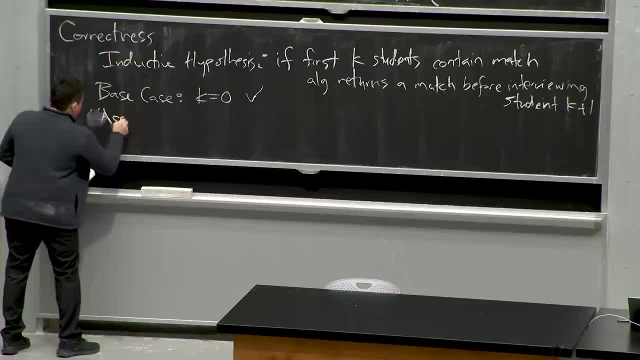 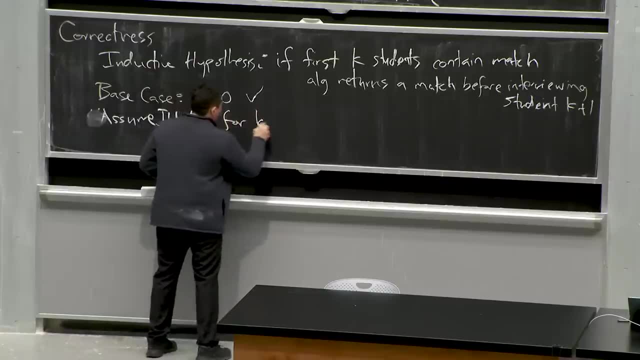 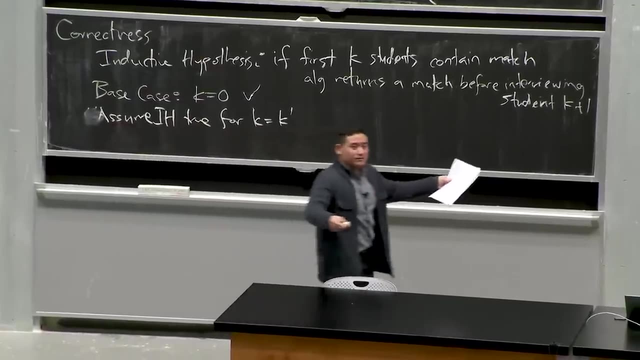 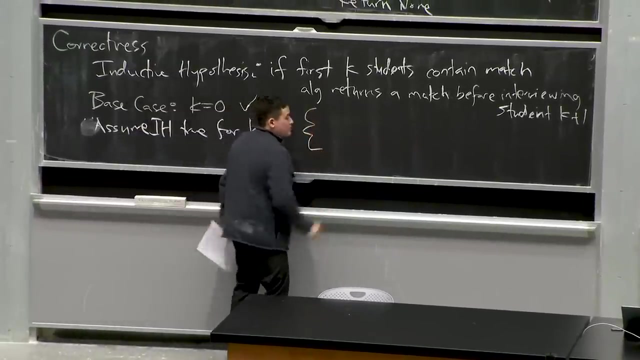 This thing right. Assume the inductive hypothesis true for k equals, say some k prime, OK, And we're considering k prime plus 1, right? Then we have two cases. One of the nice things about induction is that it isolates our problem to not you know. 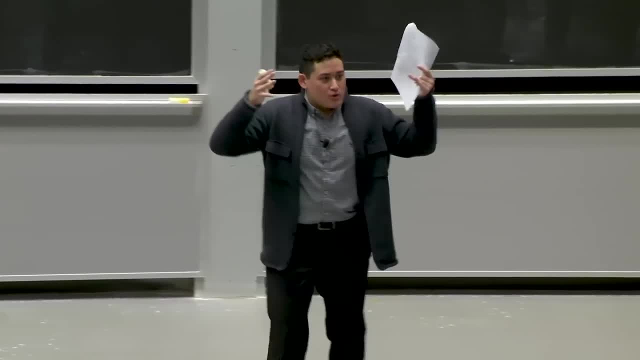 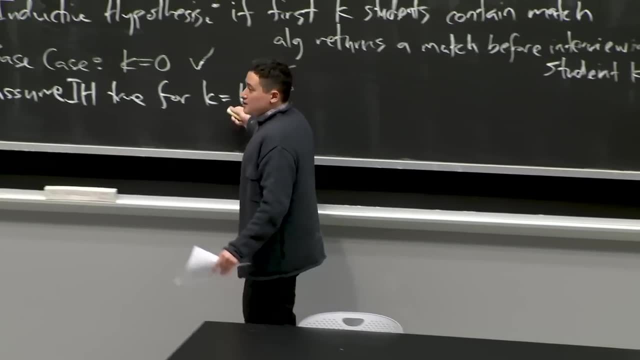 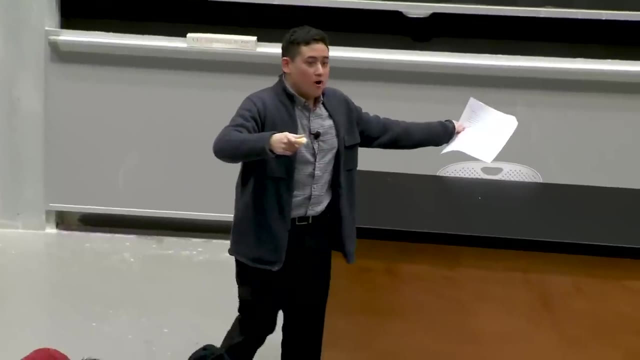 not consider everything all at once, but break it down into a smaller interface so I can do less work at each step right? So there are two cases: Either the first k already had a match, right, In which case by our inductive hypothesis. 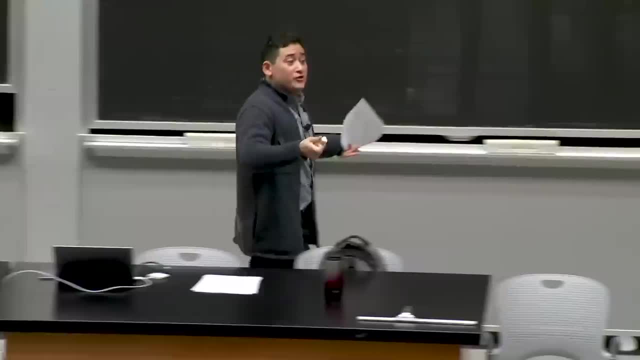 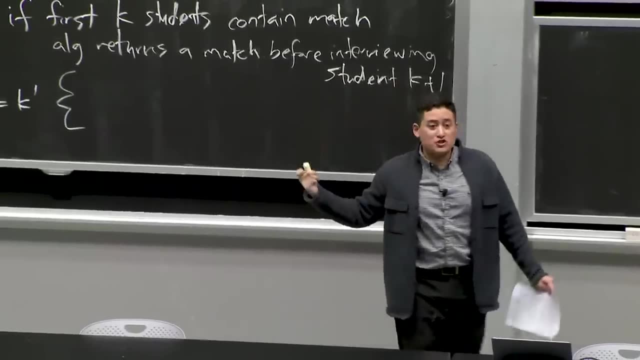 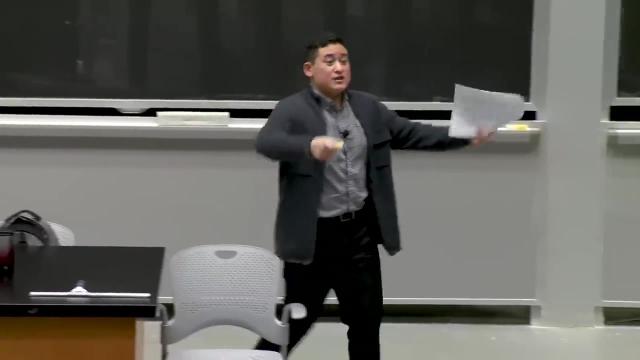 we've already returned the correct answer, right. The other case is the: It doesn't have a match and we interview the k plus 1 student, the k prime plus 1 student, If there is a match in the first k prime plus 1 students. 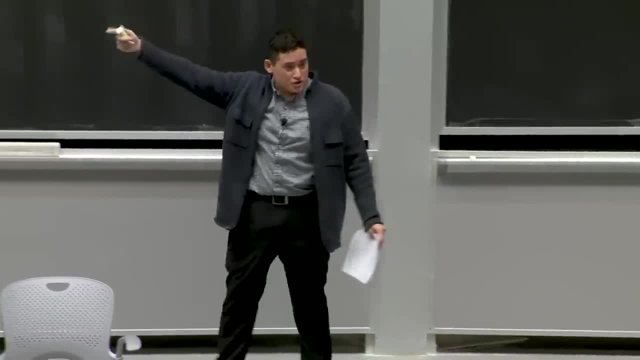 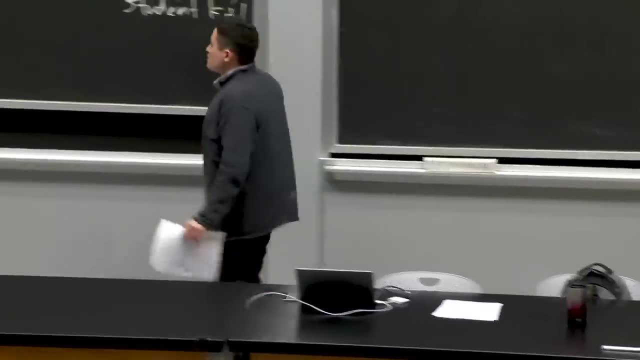 then it will include k prime plus 1,, the student k prime plus 1, because otherwise there would have been a match in the things before it, right? So there are two cases. If k, k, k, k, k. 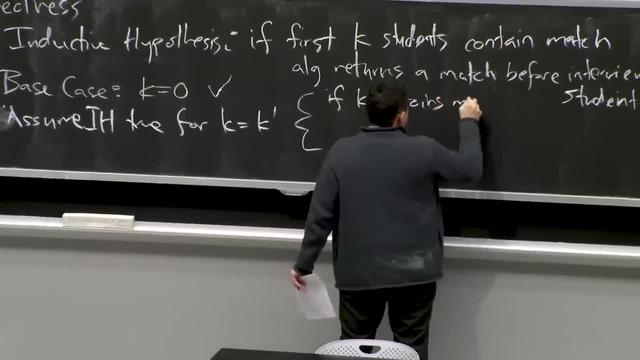 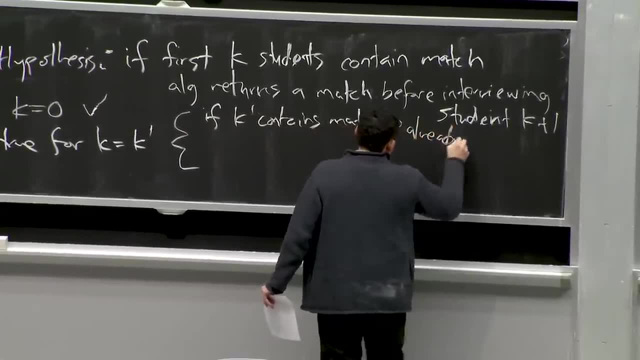 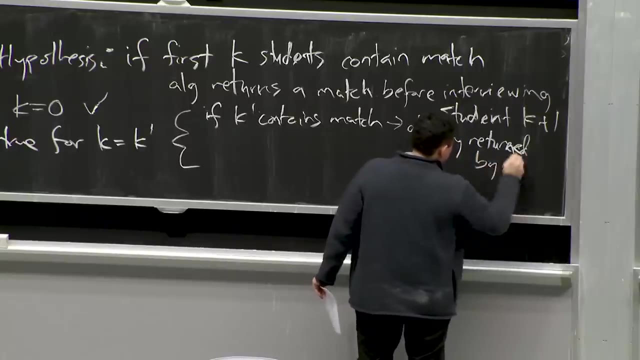 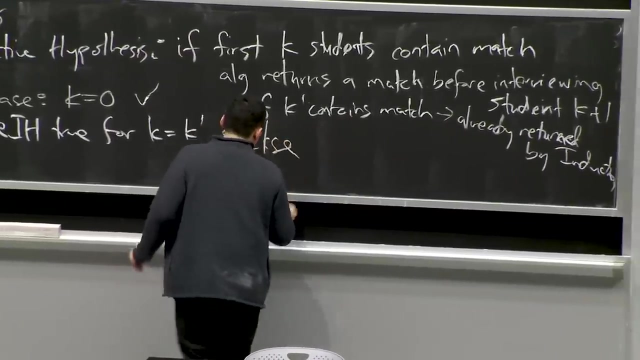 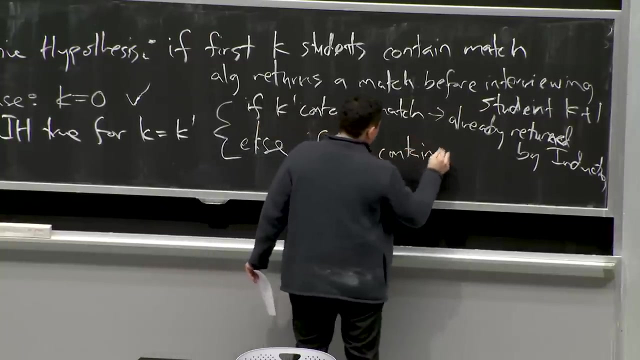 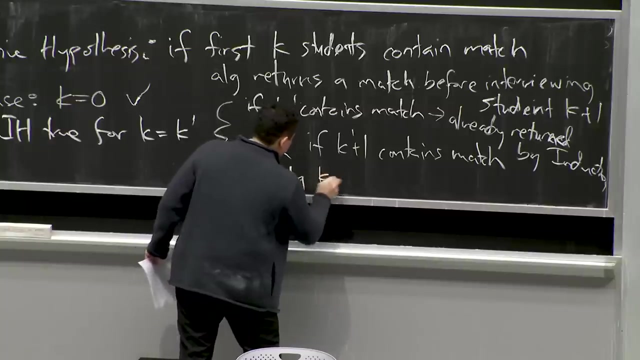 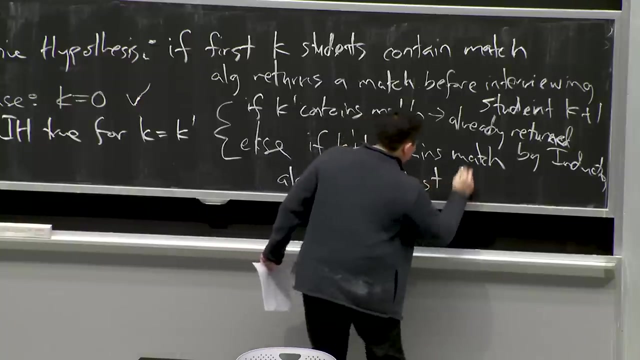 contains match k prime. If first k contains match already returned, turn mid by induction right Else. if k prime plus 1 students contains match, the algorithm checks all of the possibilities. k prime checks against all students, essentially by brute force. 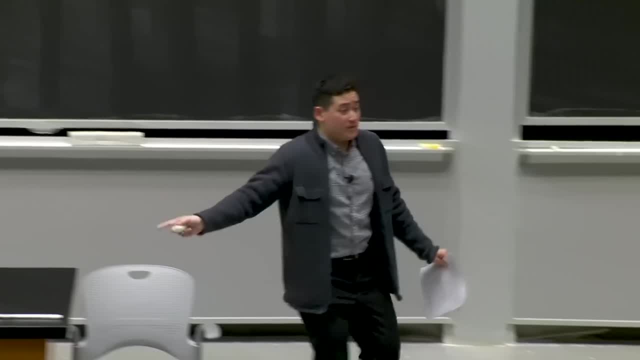 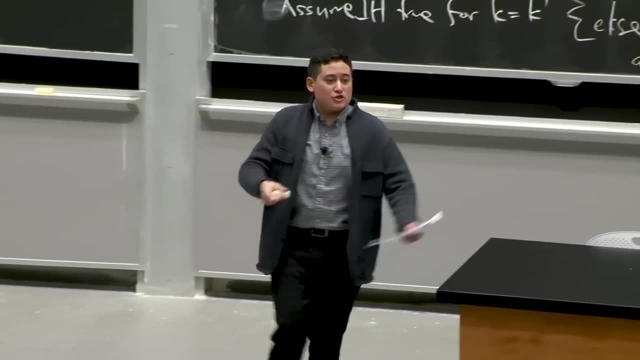 It's a case analysis. I check all of the possible possibilities right. This check if birthday is in record. I haven't told you how to do that yet, But if I'm able to do that, I'm going to check if it's in the record. 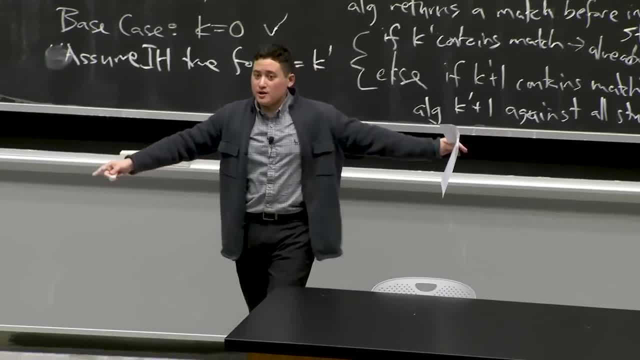 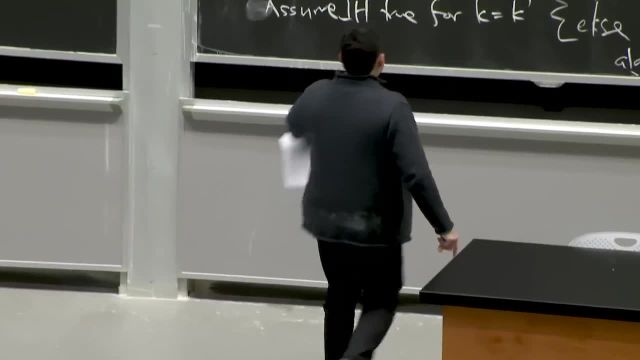 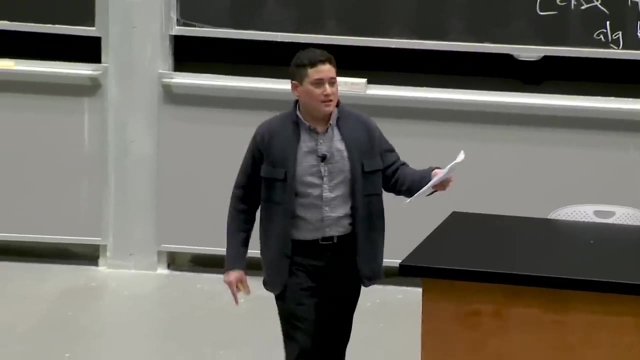 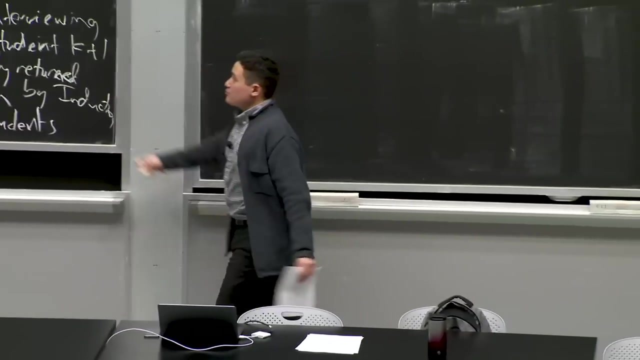 If it's in the record, then there will be a match and I can return it. Otherwise, I have re-established the inductive hypothesis for the k prime plus one students. Does that make sense, Dennis? Yeah, OK, So that's how we prove correctness. 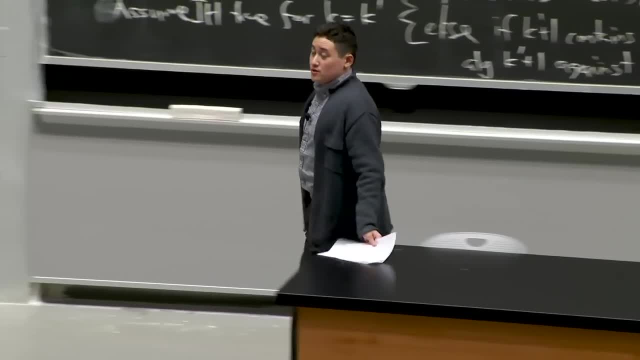 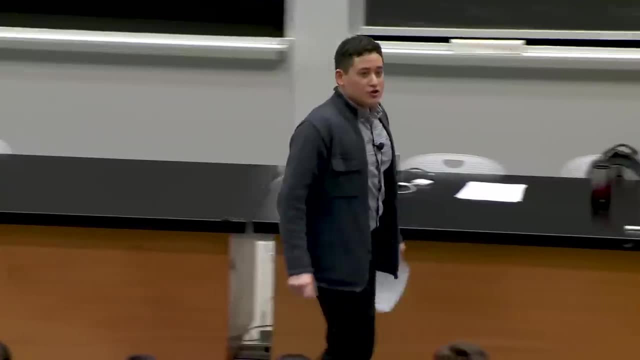 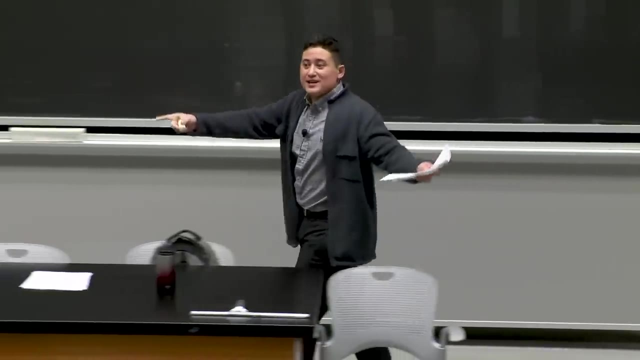 This is a little bit more formal than we would ask you to do in this class all the time, but it's definitely sufficient for the levels of arguments that we will ask you to do. The bar that we're usually trying to set is if you communicated to someone else taking 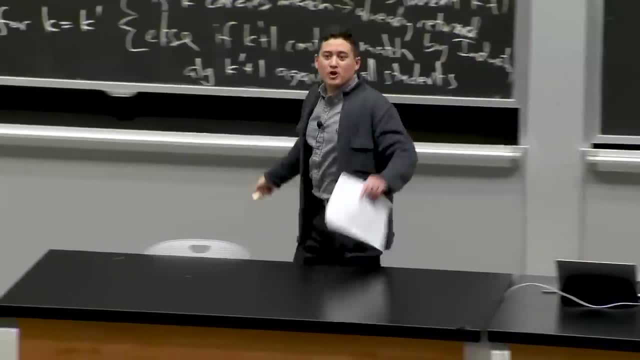 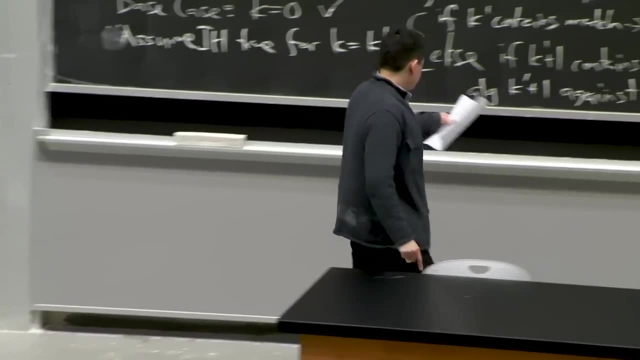 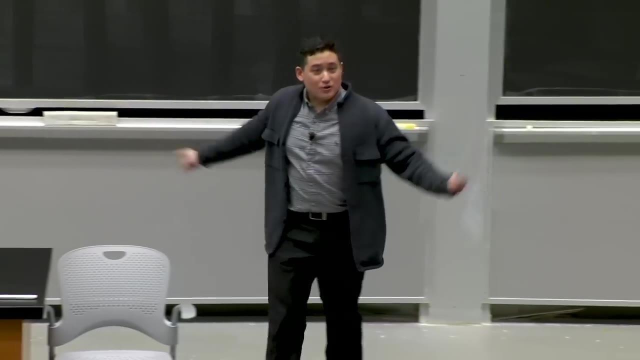 this class what your algorithm was. they would be able to code it up and tell a stupid computer how to do that. OK, So any questions on induction. You're going to be using it throughout this class, And so if you're unfamiliar with this line of argument, then you should go review some. 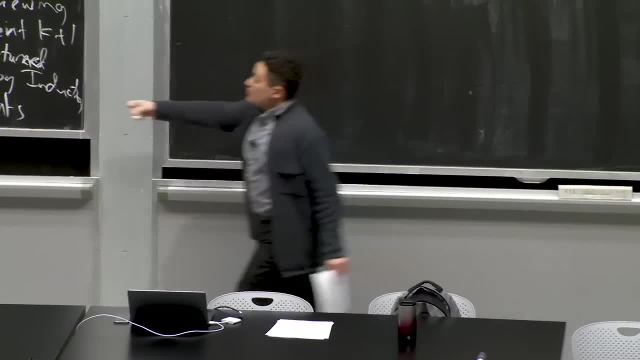 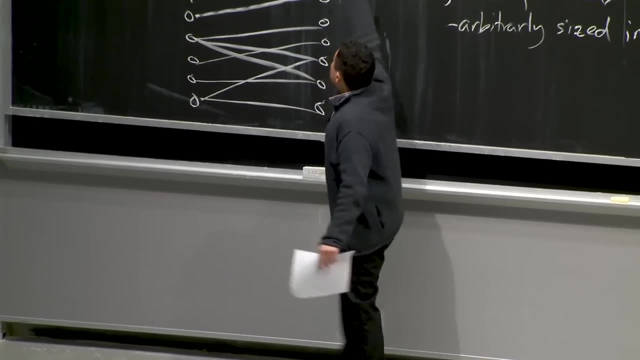 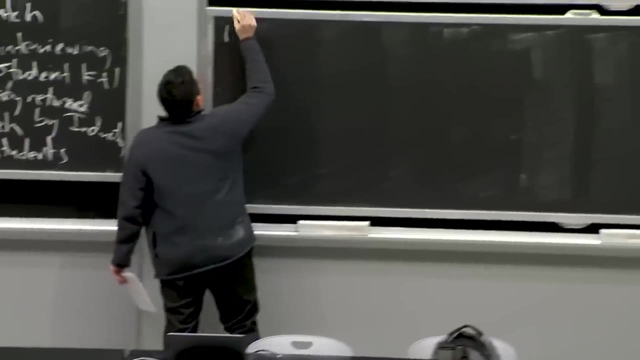 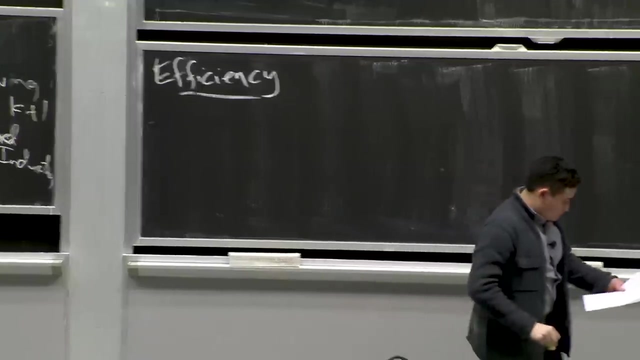 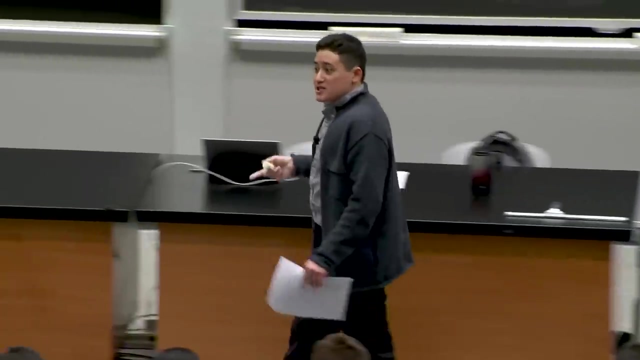 of that. That would be good. OK, So that's correctness, being able to communicate that the algorithm we stated was correct. Now we want to argue That it's efficient. right? What does efficiency mean? Efficiency just means not only how fast does this algorithm run, but how fast does it compare. 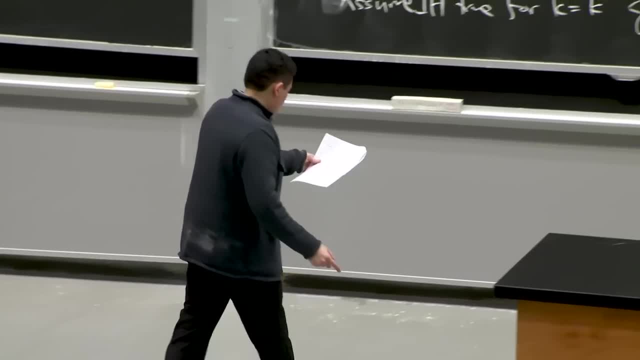 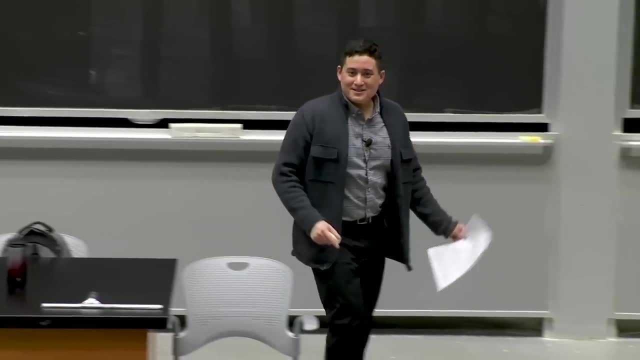 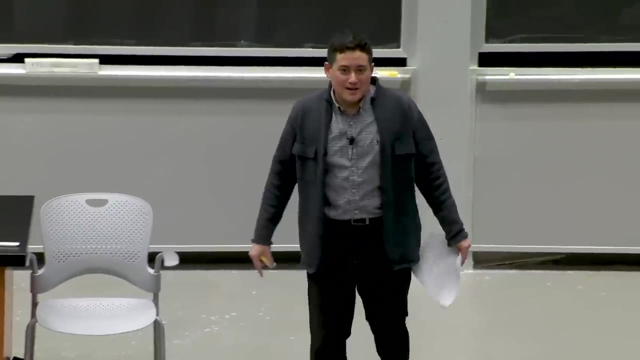 to other possible ways of approaching this problem, right? So how could we measure how fast an algorithm runs? This is kind of a silly question. Yeah, Yeah, Just well, I mean just record the time it takes for a computer to do this thing. 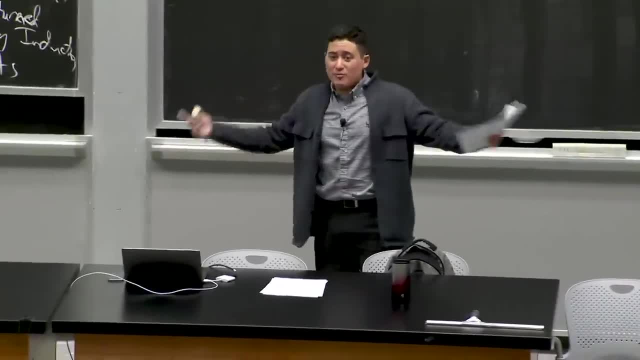 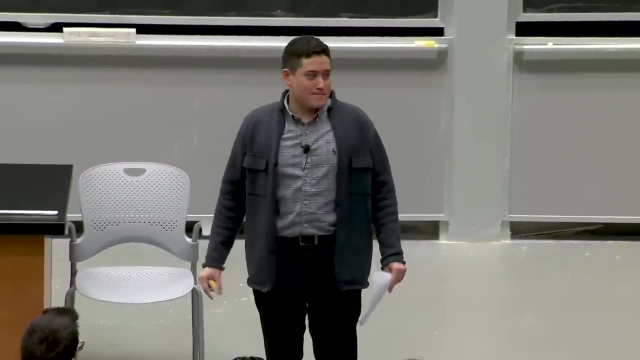 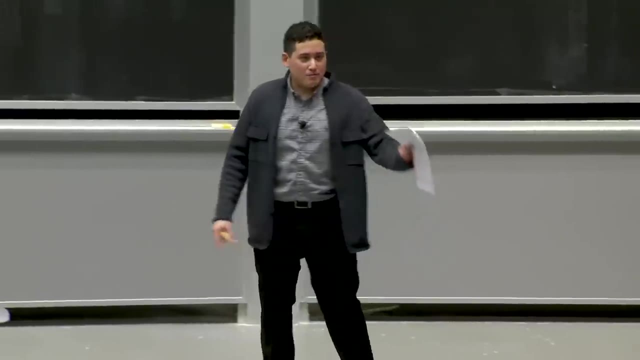 right Now, there's a problem with just coding up an algorithm telling a computer what to do and timing how long it takes Why? Yeah, It would depend on the size of your data set. OK, And you don't need to do this right. 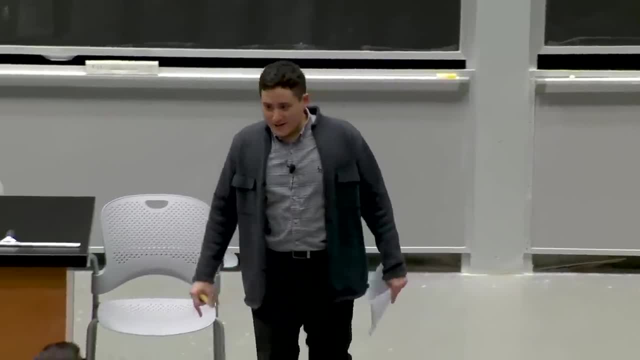 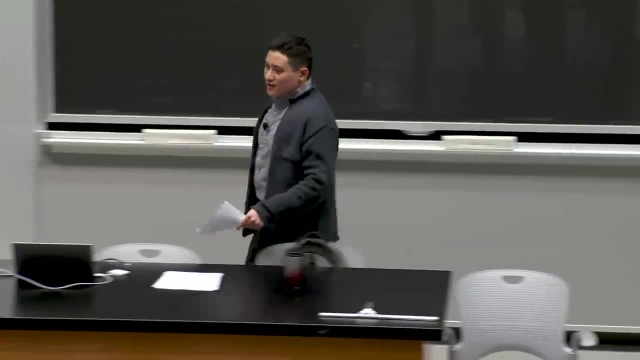 So you don't have to do this, You don't have to do that. But there's a bigger problem there. Yeah, It depends on the strength of your computer, right? So I would expect that you know if I had a watch calculator and I programmed it to. 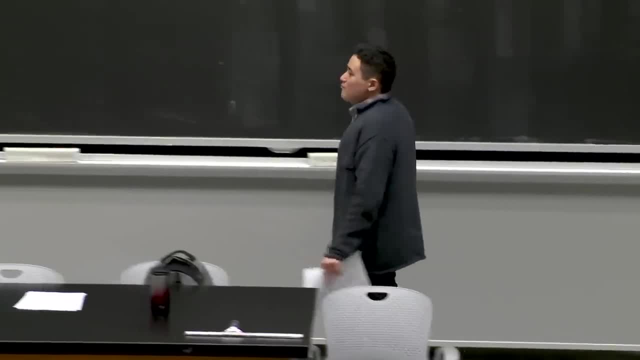 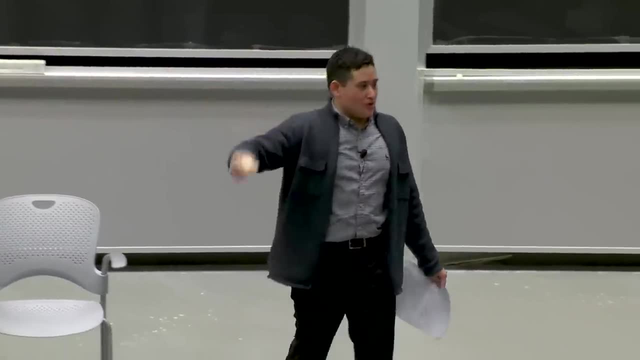 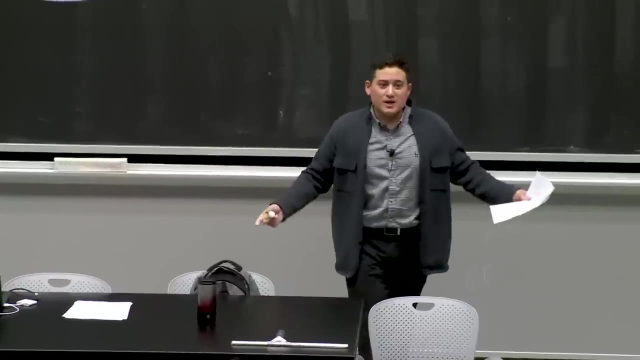 do something right. that might take a lot longer to solve a problem than if I asked you. know IBM's research computer right to solve the same problem using the same algorithm, Even with the same code? right, Because its underlying operations are much faster, right. 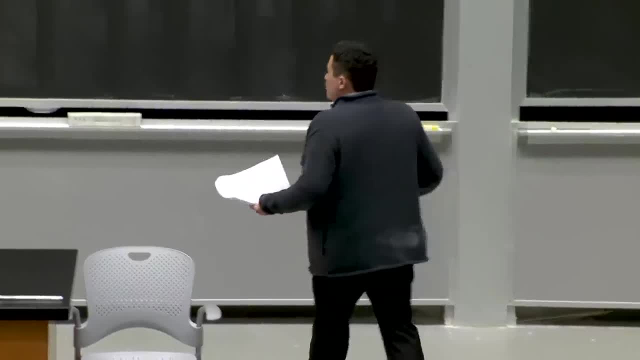 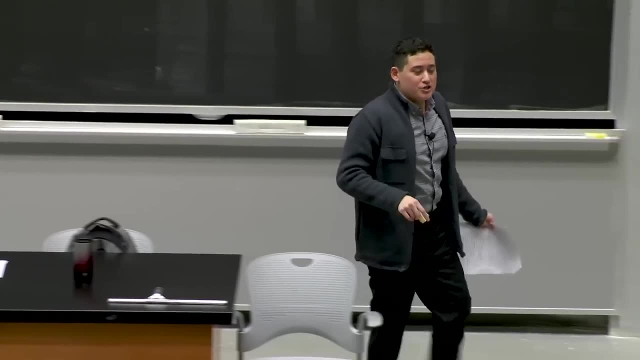 How it runs is much faster, So I don't want to count how long it would take on a real machine. I kind of want to abstract the time it takes the machine to do stuff out of the picture. What I kind of want to say is: let's assume that each kind of fundamental operation, that 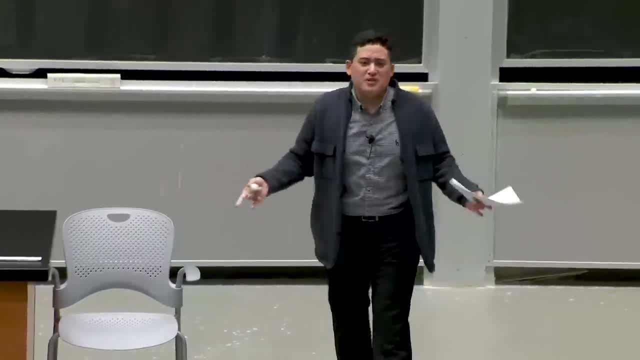 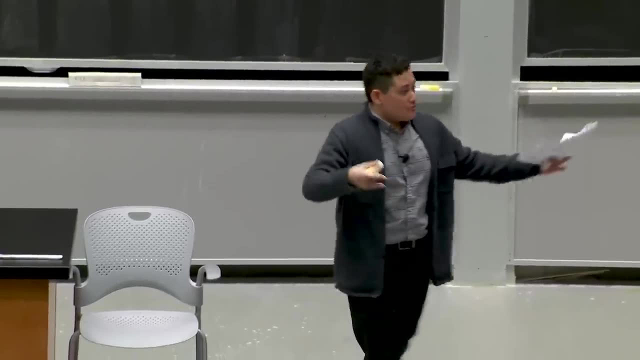 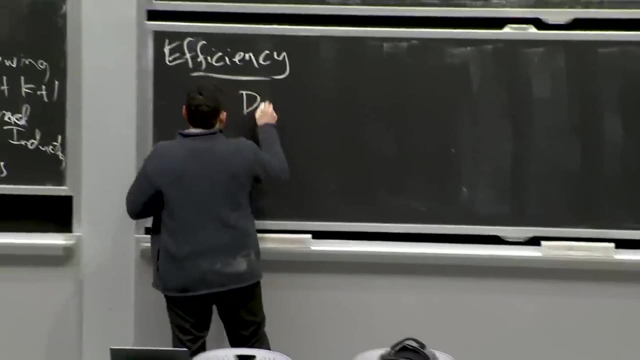 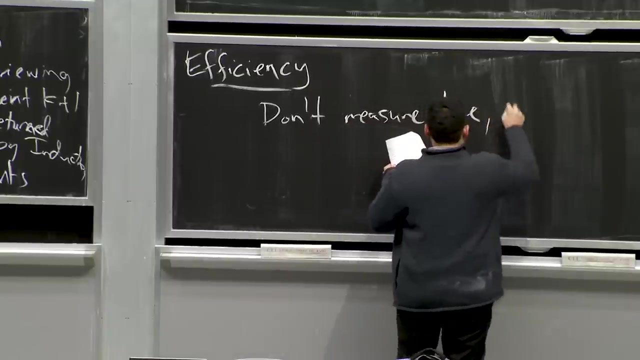 the computer can do takes some fixed amount of time. OK, How many of those kinds of things, How many of those kinds of fixed operations does the algorithm need to perform to be able to solve this problem, Right? So here we don't measure time. 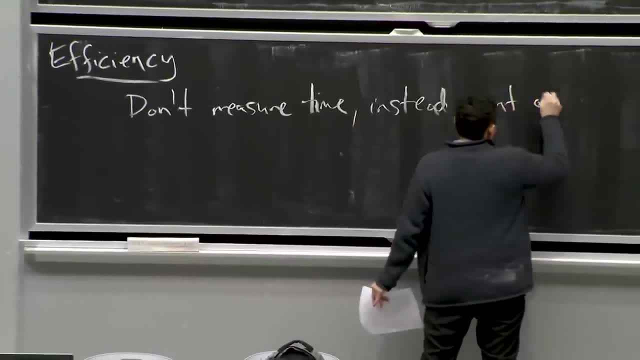 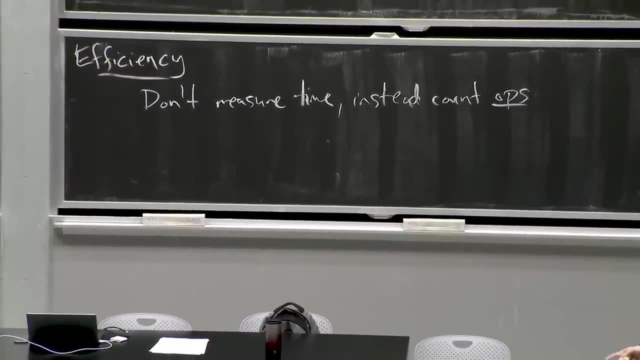 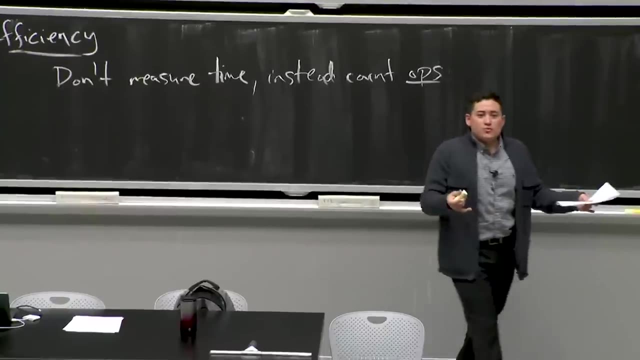 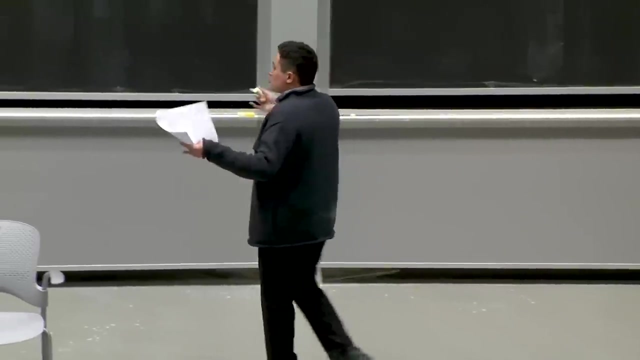 Instead count kind of fundamental operations. OK, We'll get to what some of those fundamental operations are In a second. But the idea is we want a measure of how well an algorithm performs, not necessarily an implementation of that algorithm, right, Kind of an abstract notion of how well this algorithm does. 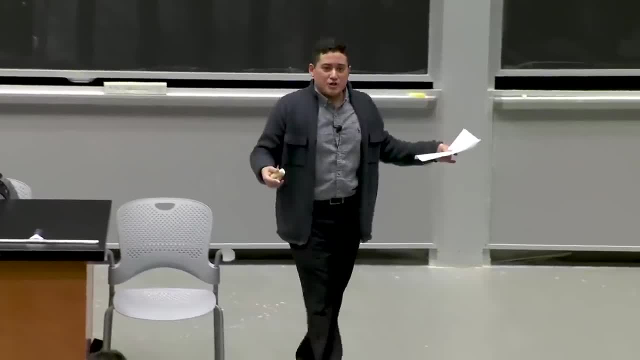 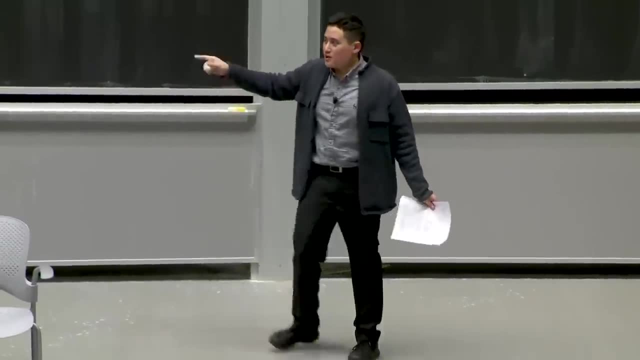 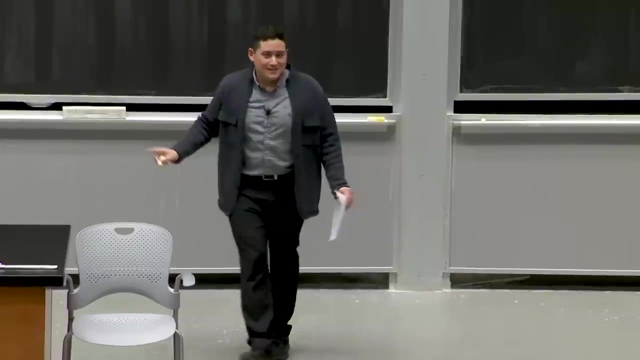 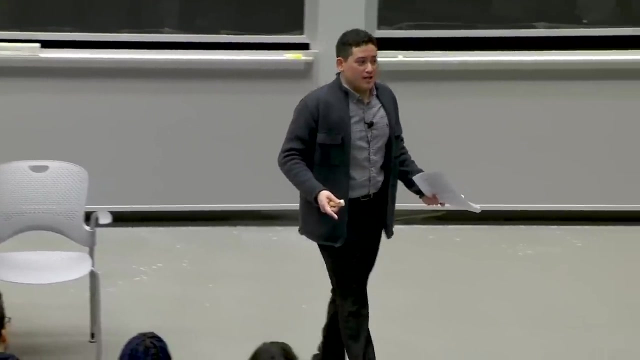 And so what we're going to use to measure time or efficiency, right, is something called asymptotic analysis. Anyone here understand what asymptotic analysis is? I think it's in both of your prerequisites, I think. But we will go through a formal definition of asymptotic notation in recitation tomorrow. 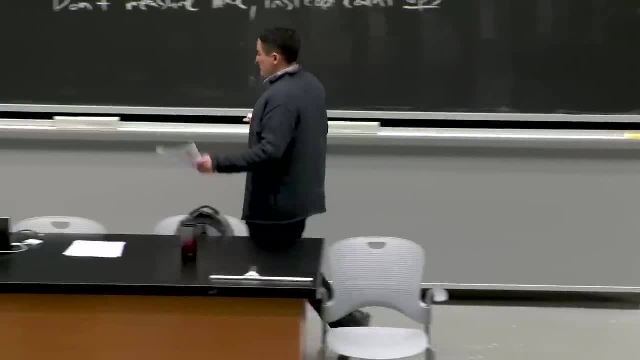 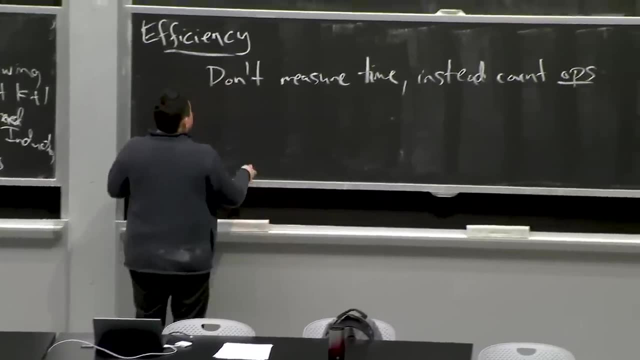 and you'll get a lot of practice in comparing functions using an asymptotic analysis. But just to give you an idea, right, the idea here is we don't measure time, We instead measure ops And, like your colleague over here was saying, before we measure time. 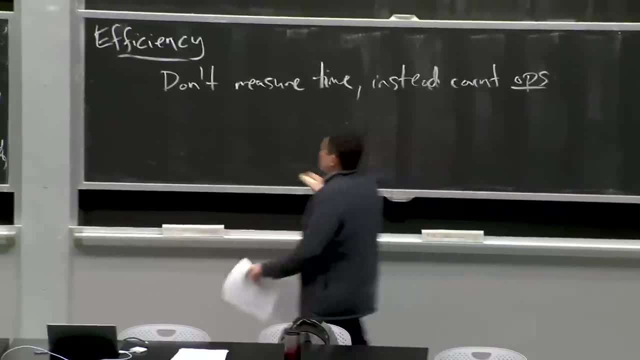 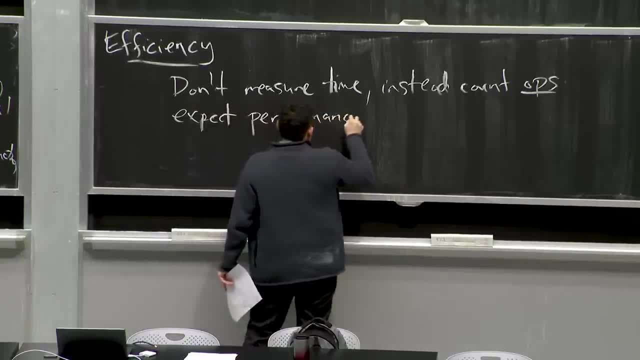 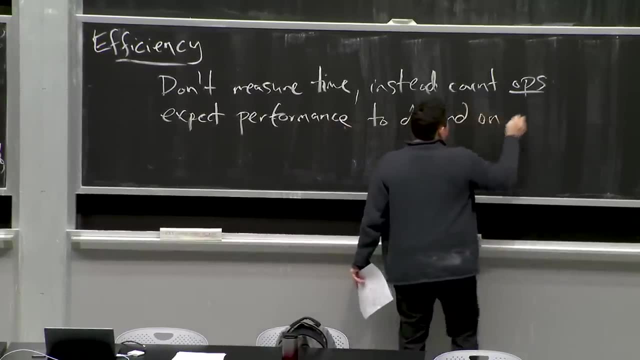 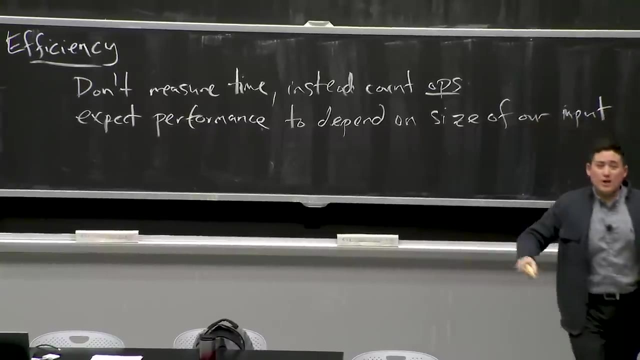 We measure time. We measure time. I'm going to use performance instead of time here. We expect that to depend on size of our input, right, If we're trying to run an algorithm to find a birthday in this section, we expect the. 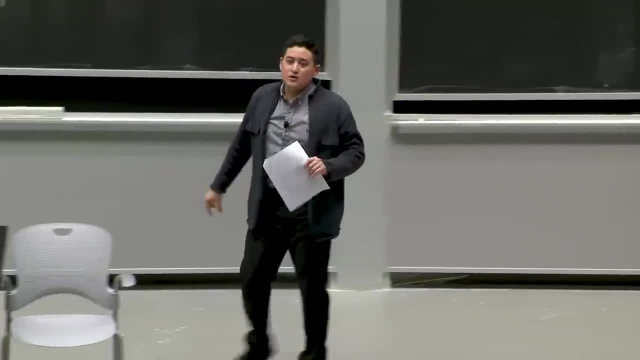 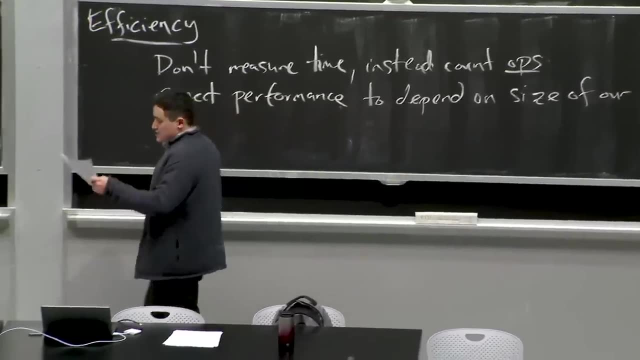 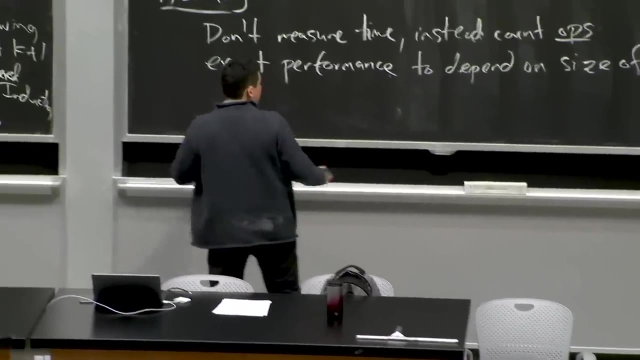 algorithm to run in a shorter amount of time than if I were to run the algorithm on all of you, right? So we expect it to perform differently depending on the size of the input, and how differently is how we measure performance relative to that input. Usually we use n as. 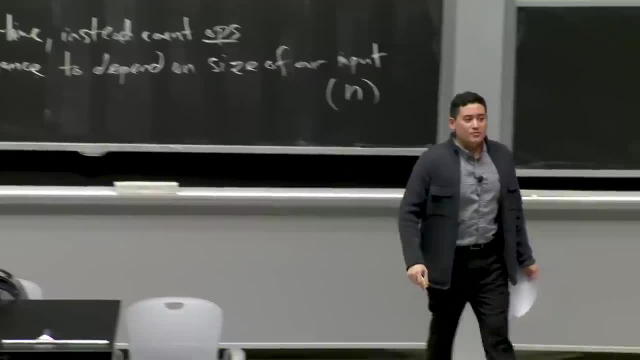 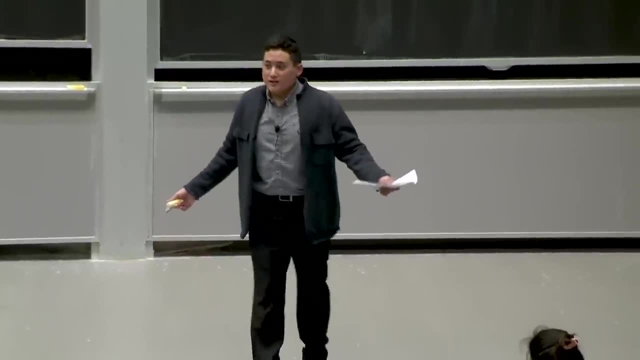 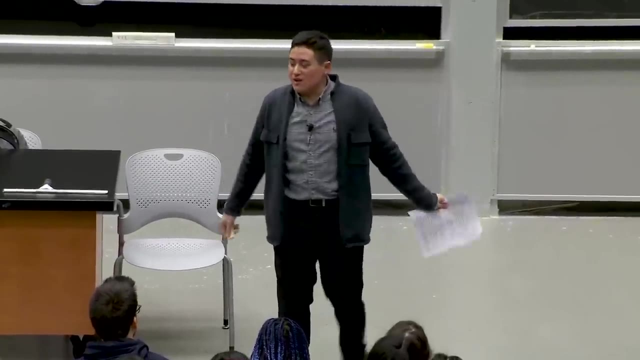 a variable for what the size of our input is right, But that's not always the case. So, for example, if we have an array that I give you an n by n array, right That we're going to say n, but what's the size of our input? How much information do I need to convey? 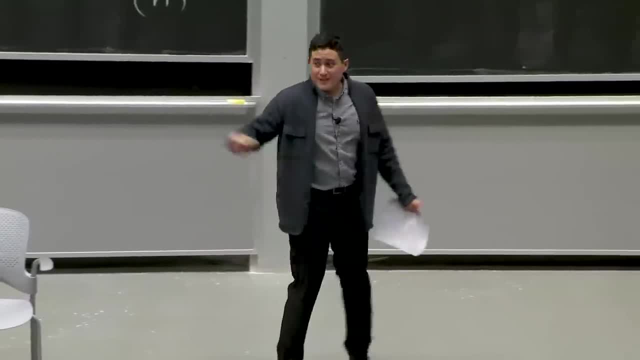 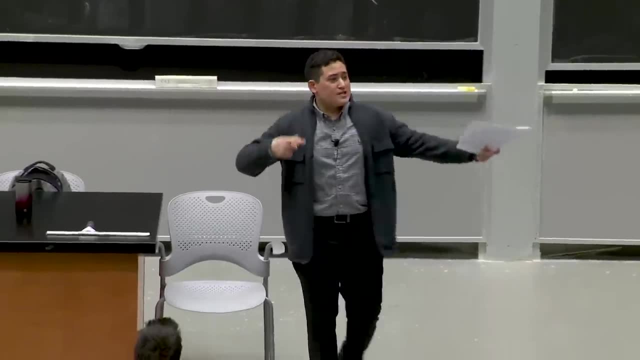 to you. to give you that information. It's n squared right, So that's the size of our input in that context, right? Or if I give you a graph, it's usually the number of vertices plus the number of edges. That's how big, how much space I would need to convey to you. 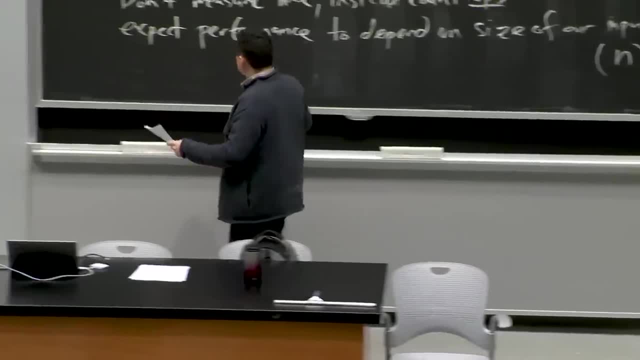 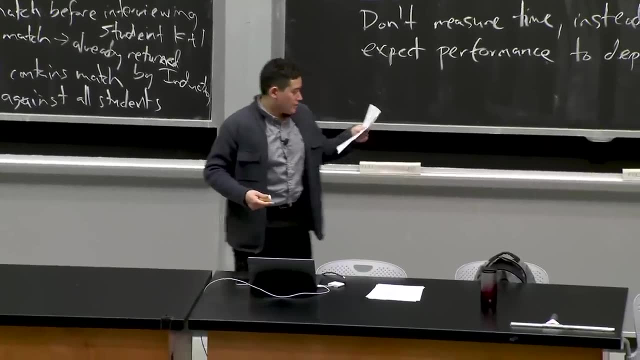 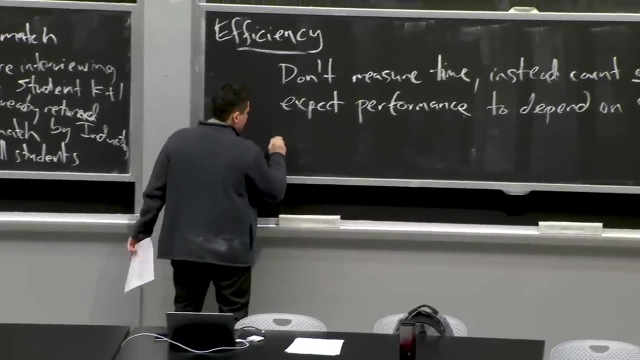 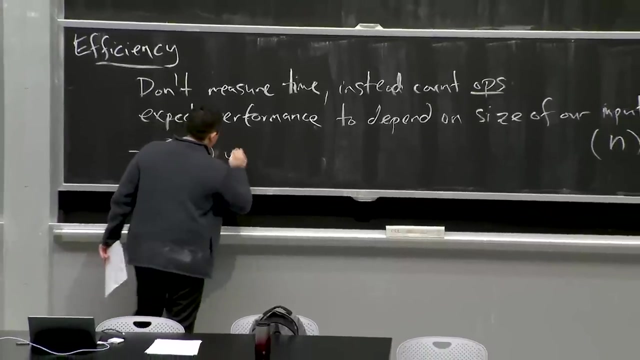 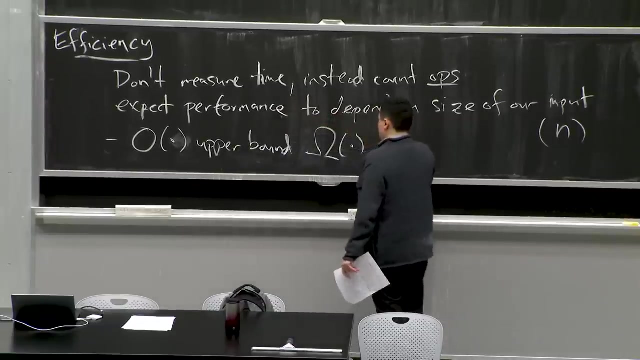 that graph, That information. OK, So we compare how fast an algorithm is with respect to the size of the input, right, And if that, we will use the asymptotic notation. We have big O notation, which corresponds to upper bounds. We will have omega, which corresponds to upper bounds. 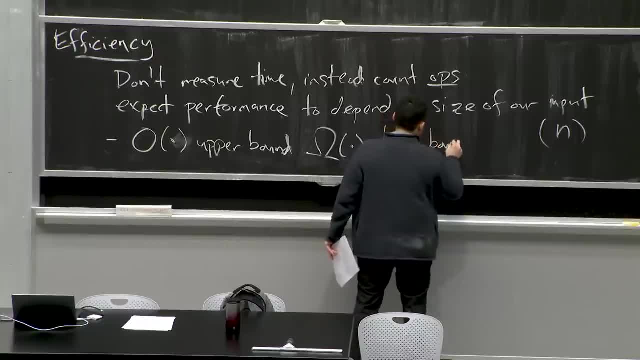 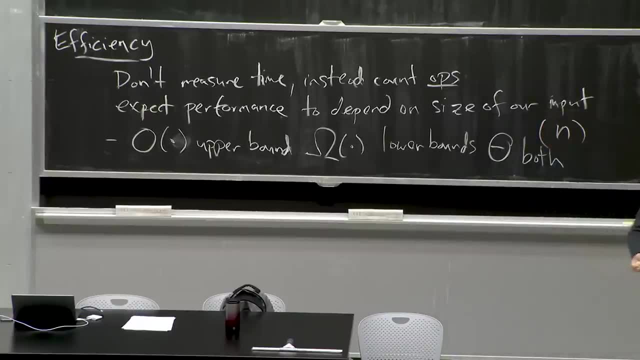 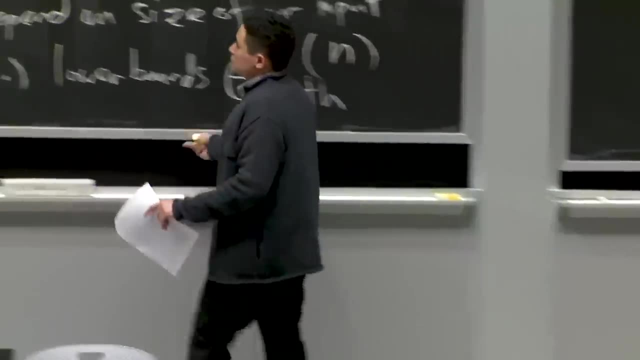 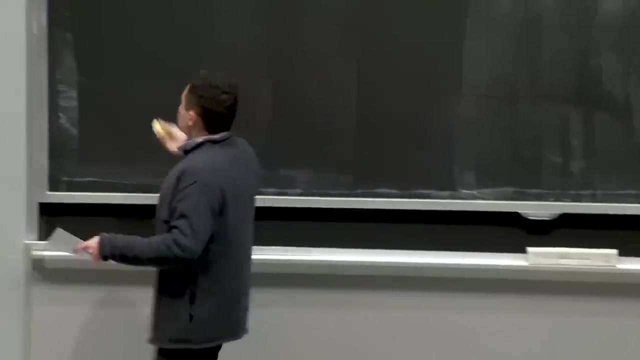 And we have theta, which corresponds to lower bounds, And we have theta, which corresponds to both right. This thing is tight. It is bounded from above and below by a function of this form. OK, Now we have a couple of common ways, a couple of common functions. 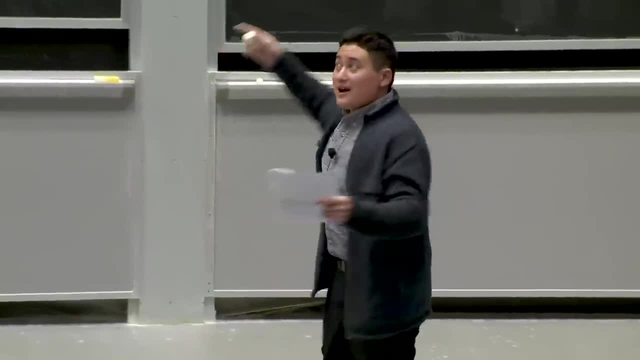 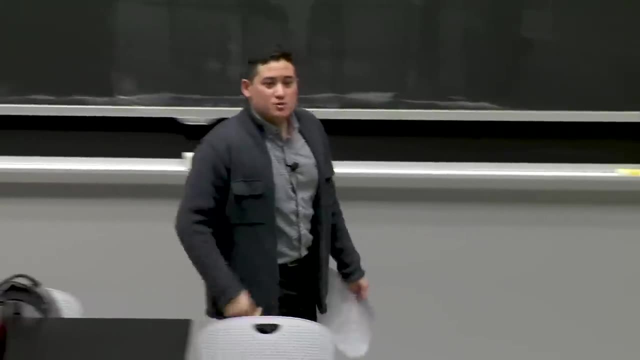 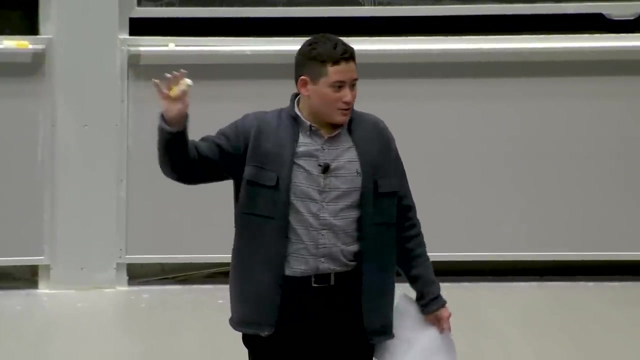 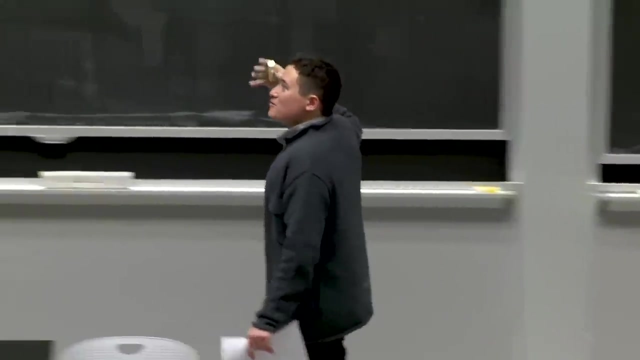 That algorithms their running time. we have a couple of common functions that relate an algorithm's input size to its performance, some things that we saw all the time. Can anyone give me some of those? Say again, Insert that, Sorry, So like a function. I'm not asking this question, well, But has anyone heard of 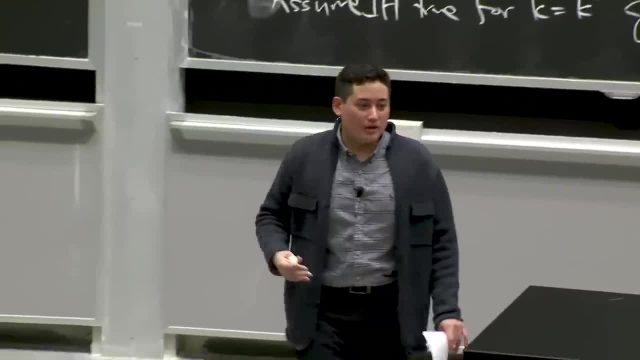 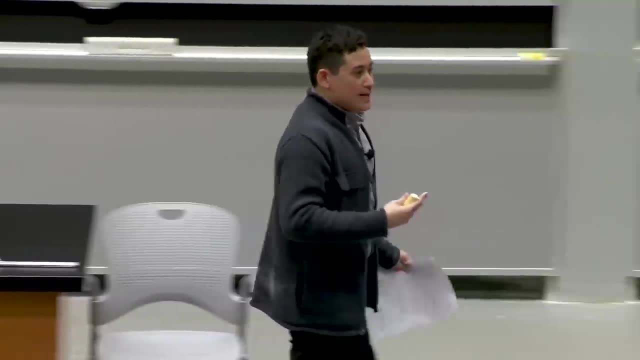 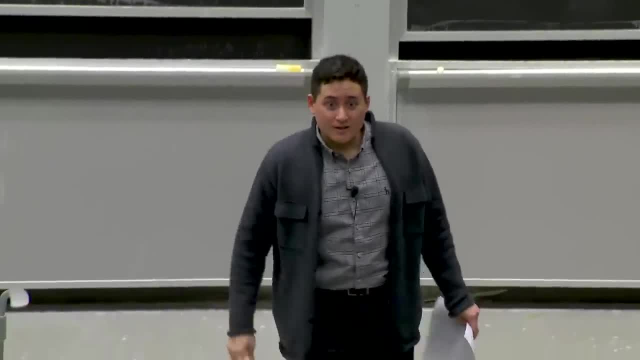 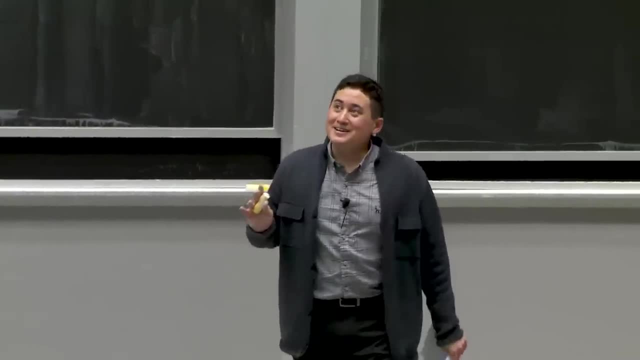 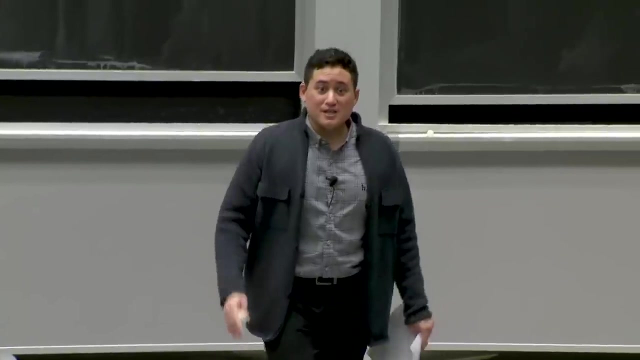 of my input, right Yeah, Say again, Like putting something in a list, Like putting something in a list, OK, so that's. there's a lot behind that question that we'll go into later this week, But that's an example of if I do it in a silly way. I 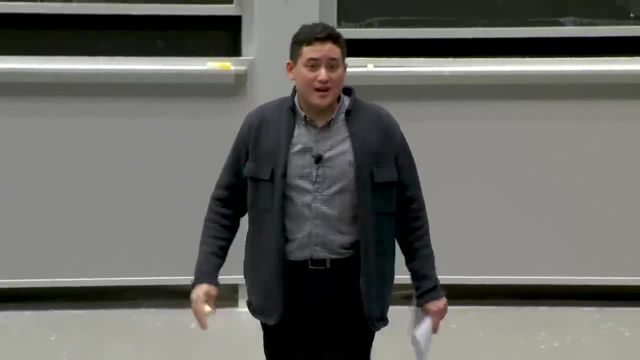 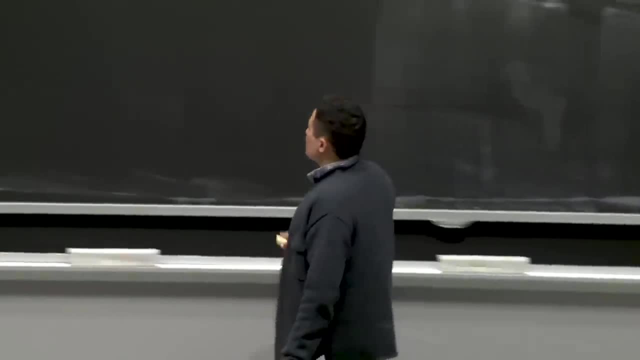 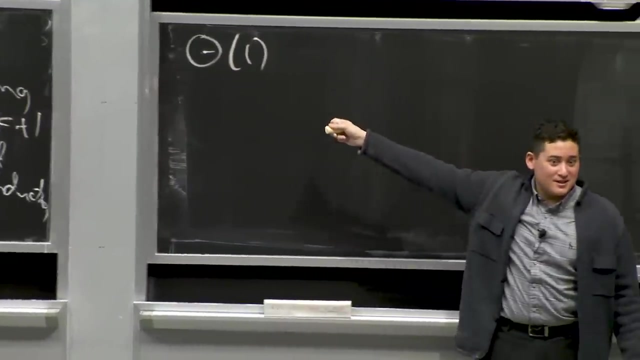 stick something in the middle of a list and I have to move everything. that's an operation that could take linear time, right? OK, So linear time is a type of function. We've got a number of these. I'm going to start with this one. Does anyone know what this one is? 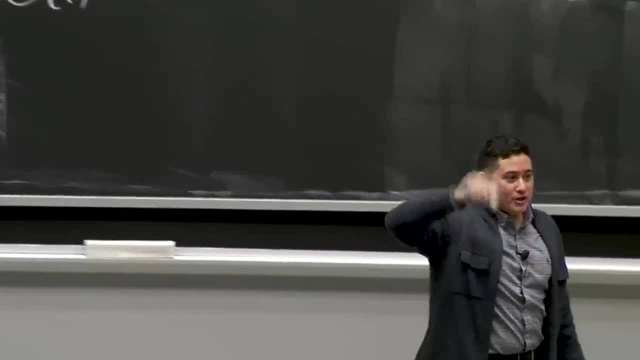 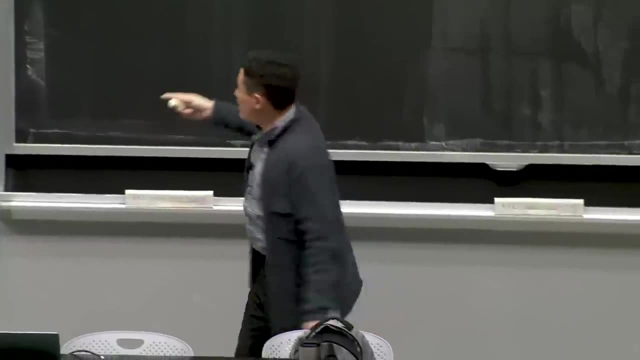 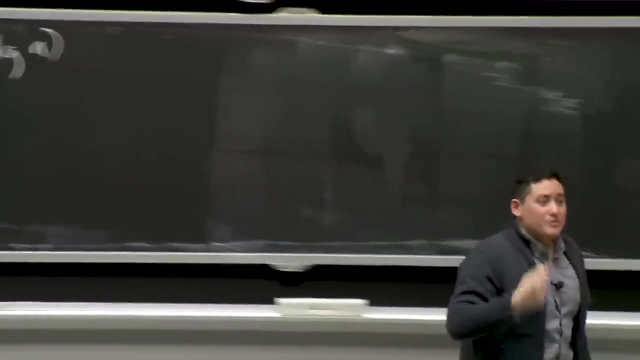 Constant time. OK, Basically, no matter how I change the input, the amount of time this running time, the performance of my algorithm takes, it doesn't really depend on that. OK, The next one up is something like this: This is logarithmic time. OK, We have theta n, which. 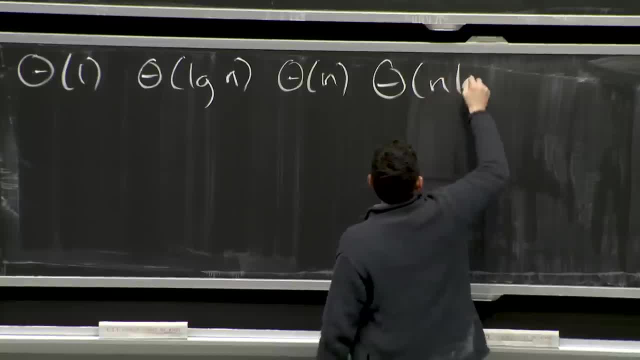 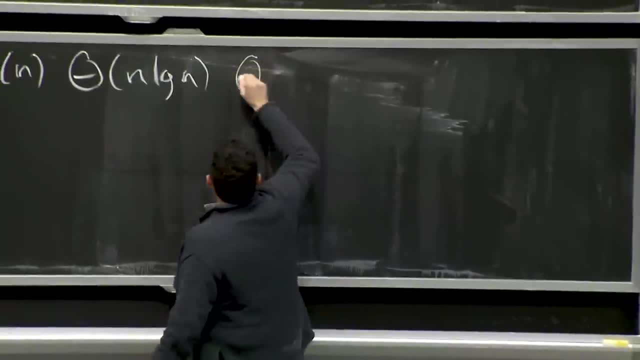 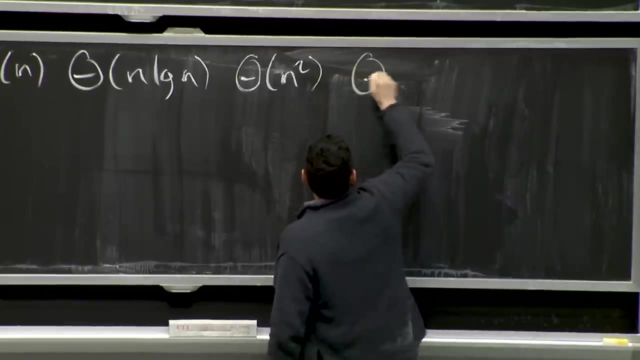 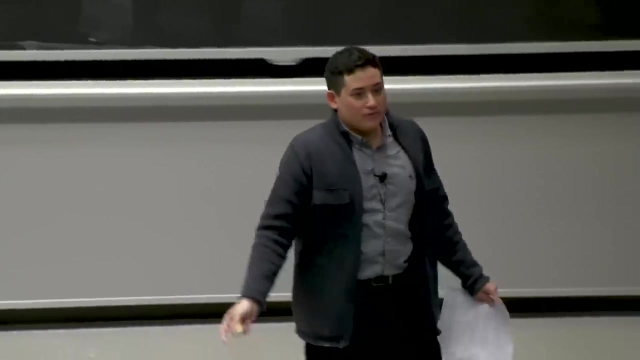 is linear: n log n. right. Sometimes we call this log linear, but we usually just say n log n. OK, We have a quadratic running time In general. if I have a constant power up here, right, OK, It's n to the c for some constant. This is what we call polynomial time, right As long. 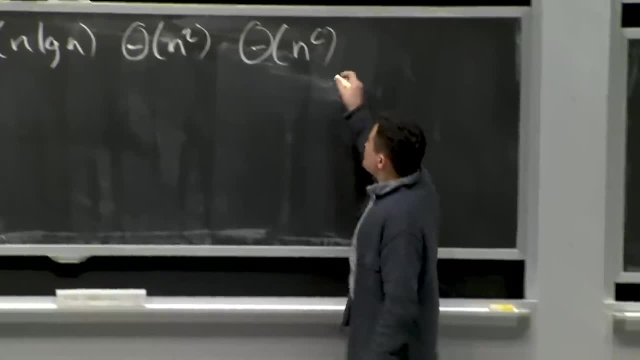 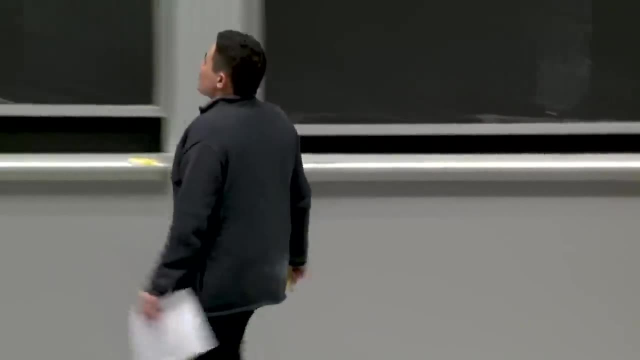 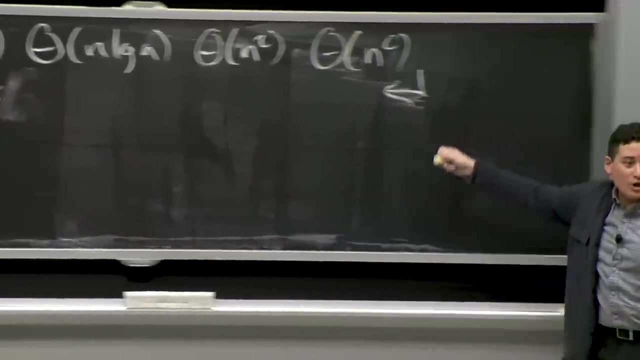 as c is some constant, And this, right here, is what we mean by efficient in this class usually right. In some other classes, right, when you have big data sets, maybe this is efficient, right, But in this class generally what we mean is polynomial, And as you get, 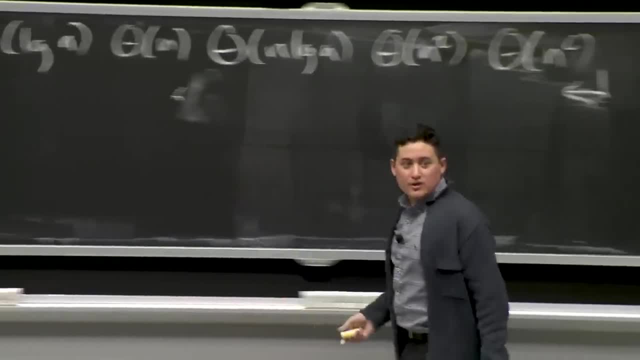 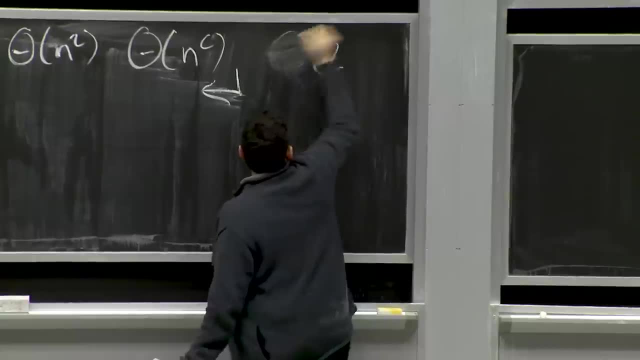 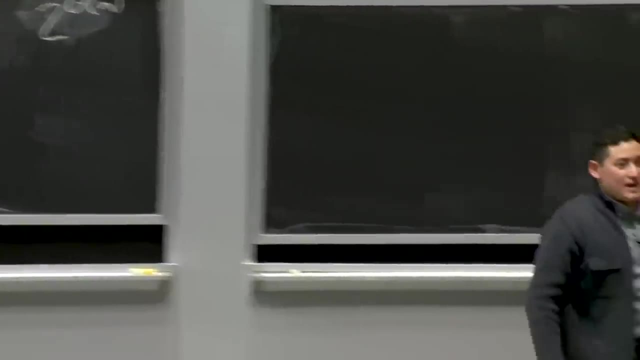 down this thing. these things are more and more efficient. OK, There's one class I'm going to talk to you about over here which is something like: let's do this: 2 to the theta of n, right Exponential time. this is some constant to. 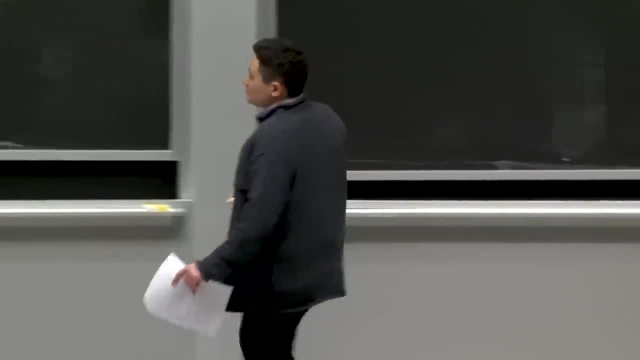 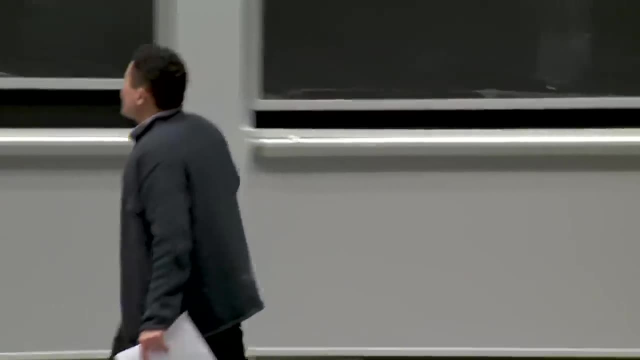 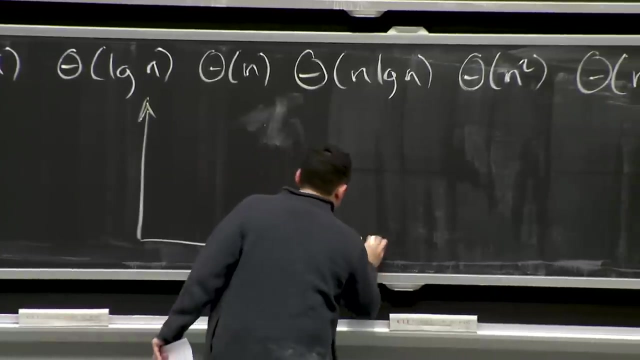 a function of n that's, let's say, super linear. That's going to be pretty bad. Why is it pretty bad? Well, I'm going to plot some of these things as a function of n. right, Let's say I plot. 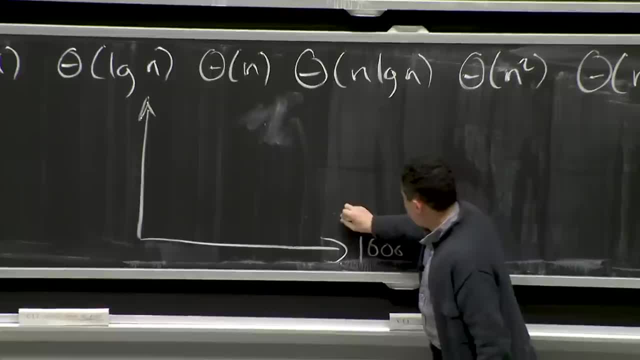 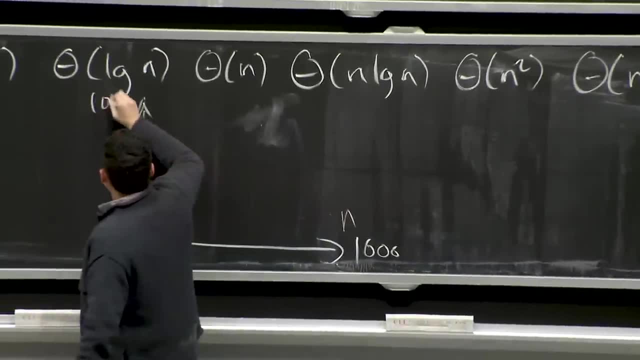 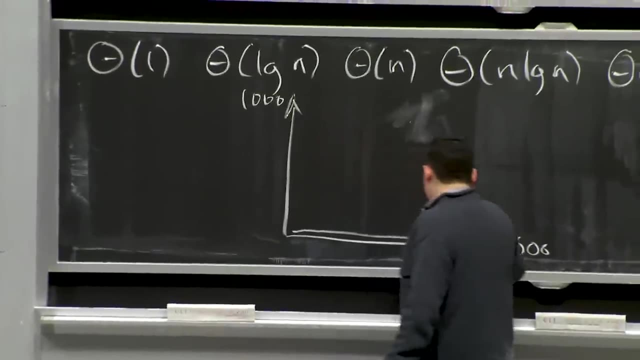 values of up to 1,000 on my n scale here. OK, What does constant look like? Maybe this is 1,000 up here too. What does a constant look like? Looks like a line, right, It looks like a line over here. somewhere. It could be as high as I want, But eventually any. 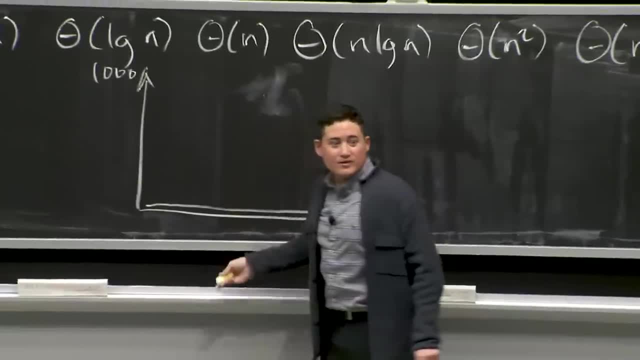 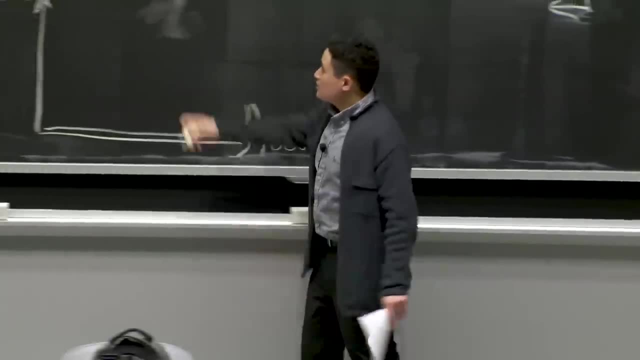 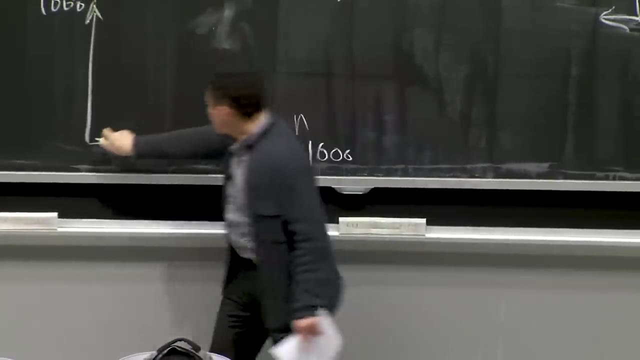 thing that's an increasing function will get bigger than this right, And on this scale, if I use log, base 2 or some reasonable small constant, what does log look like? Well, let's do an easier one. What does linear look like? Yeah, this right. 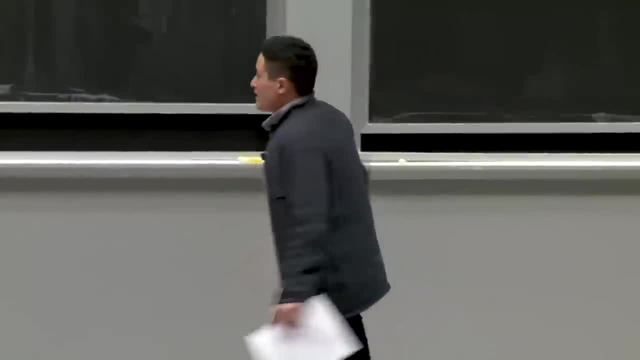 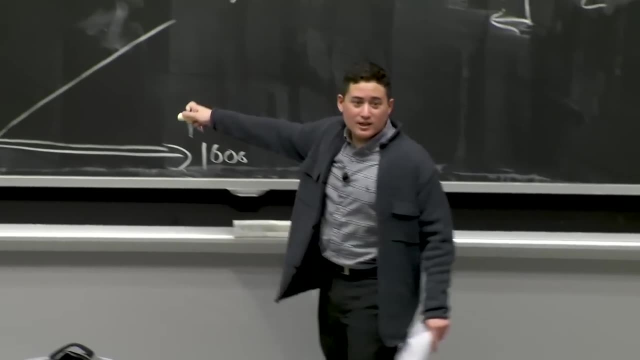 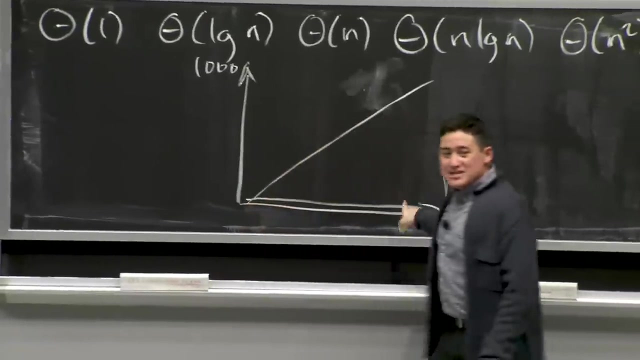 That's what I saw a lot of you doing. OK, That's linear, That's the kind of base that we are comparing everything against. What does log look like Like this? OK, But at this scale, right at this scale, really, it's much closer to constant than 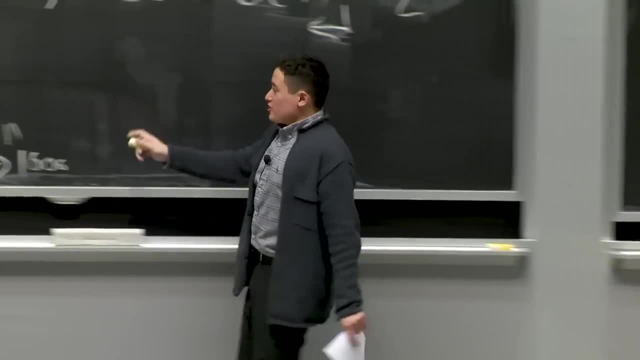 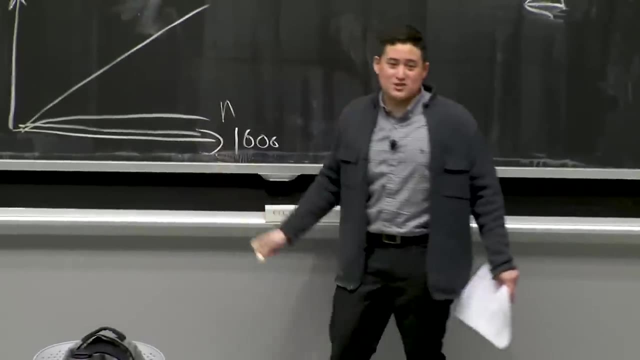 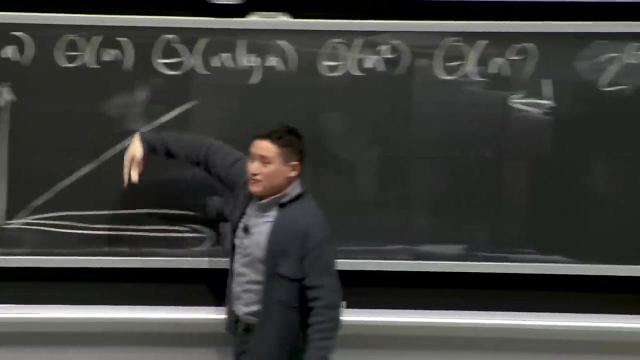 linear And actually, as n gets much, much larger, this almost looks like a straight line, It almost looks like a constant. So log is almost just as good as constant, right? What does exponential look like? It's the exact inverse of this thing. right, It's the. 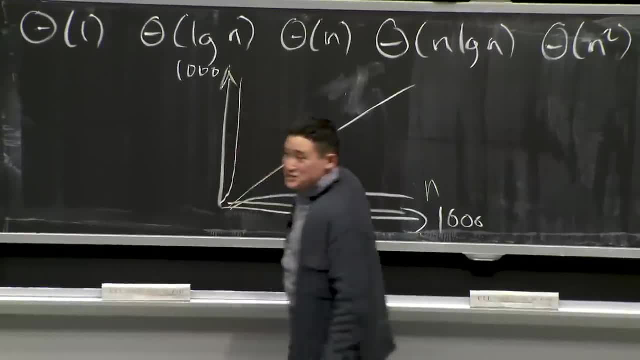 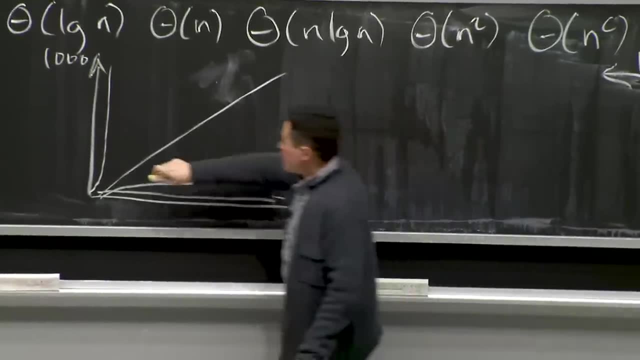 one. So log is almost just as good as constant. It's the exact inverse of this thing. right, It's almost an exact straight line going up. So this is crap. This is really good. Almost anything in this region over here is better. 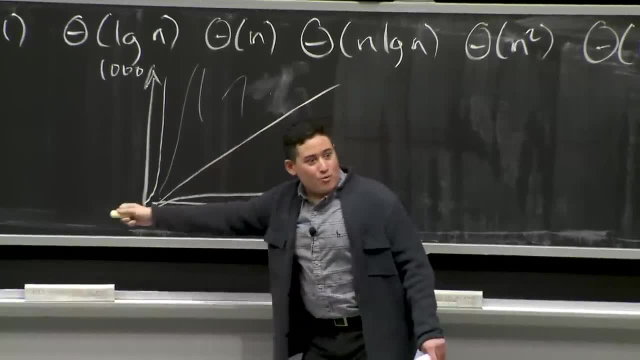 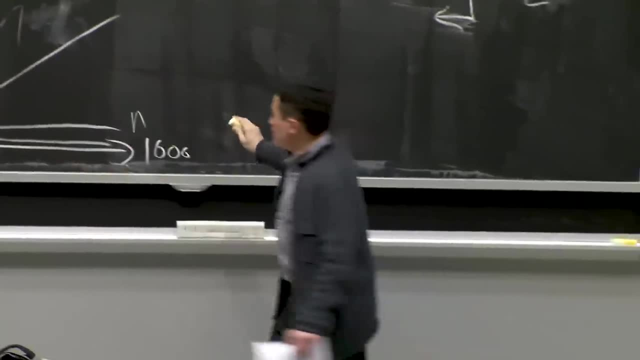 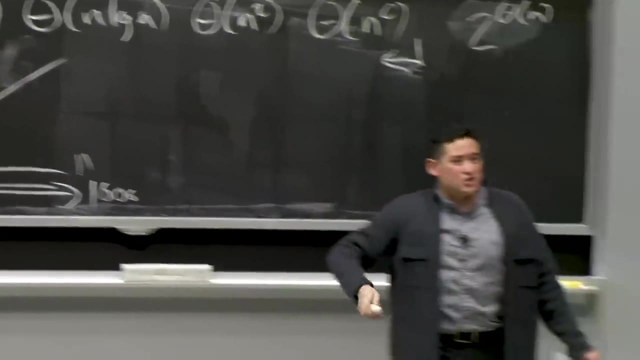 At least I'm gaining something. I'm able to not go up too high relative to my input size. So quadratic, I don't know, is something like this, and n log n is something like this, And log n after a long time really starts just looking linear with a constant multiplied. 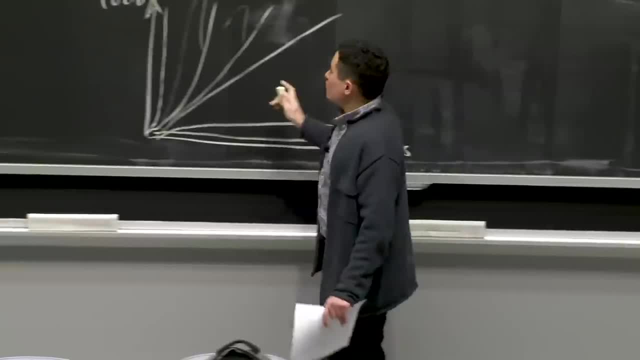 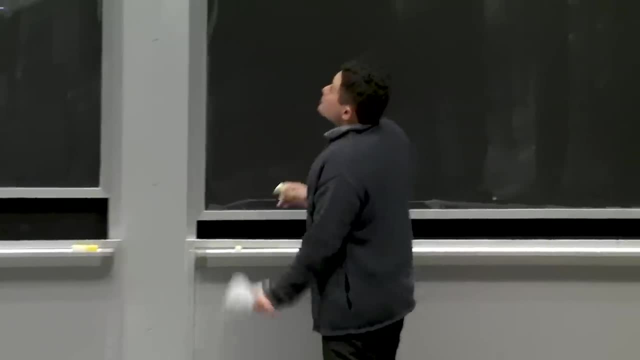 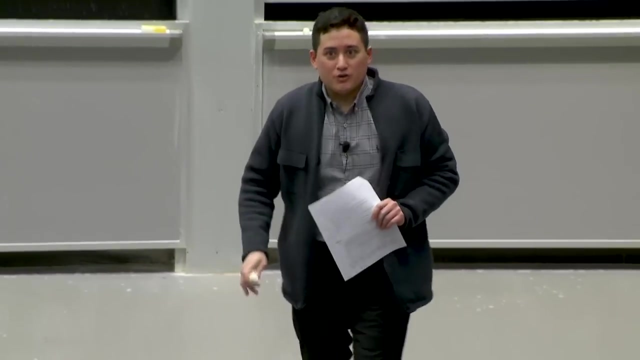 in front of it. So these things good, that thing bad. That's what that's trying to convey. So how do we measure these things if I don't know what my fundamental operations are that my computer can use? So we need to define some kind of model of computation. 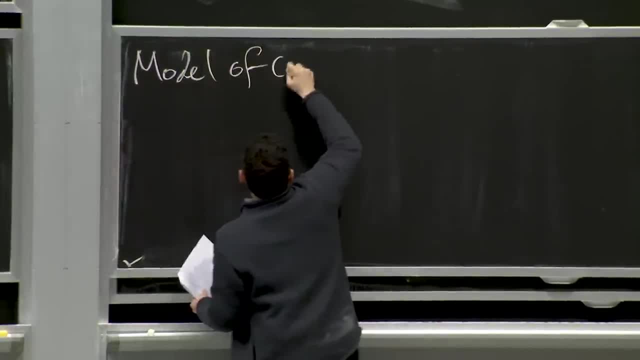 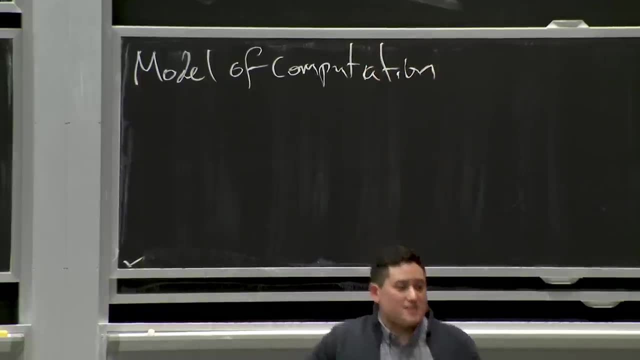 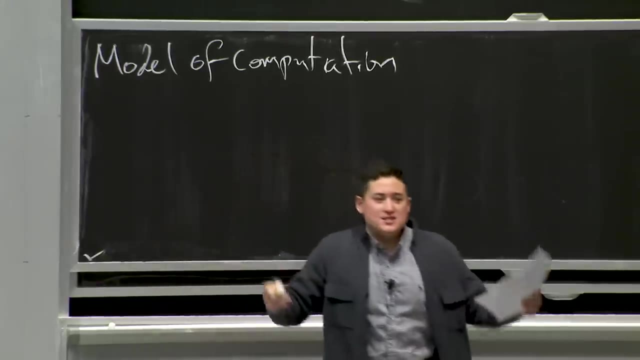 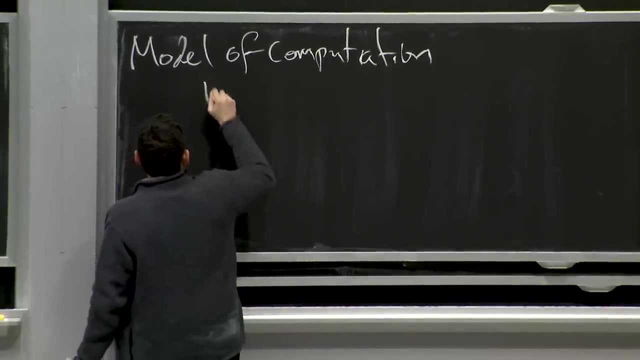 For what our computer is allowed to do in constant time in a fixed amount of time. In general, what we use in this class is a machine called a word RAM, which we use for its theoretical brevity, Word RAM. It's kind of a.